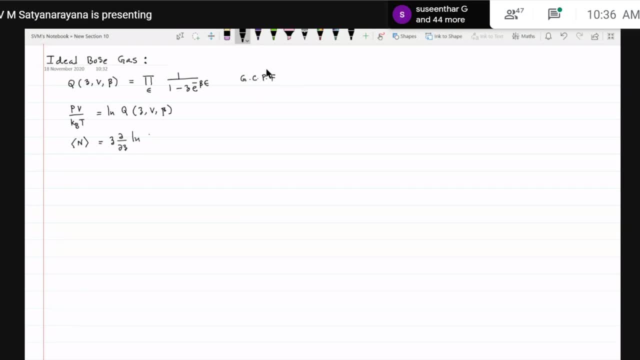 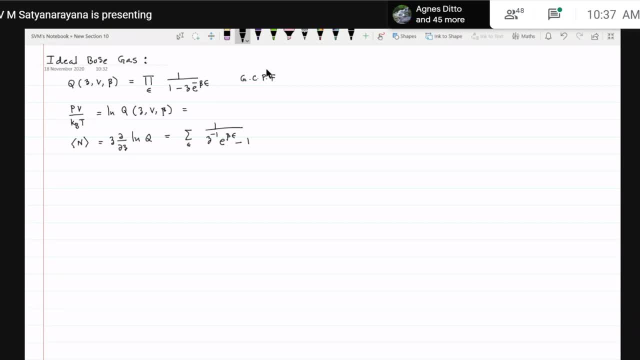 able, Kelvin by Kelvin related to mu of K, impossible. let us call it mu, whichever you. So this implies that 3D by 3DT can be written as minus one more single particle in the three levels, rather than one plus or one minus Z into the minus theta. 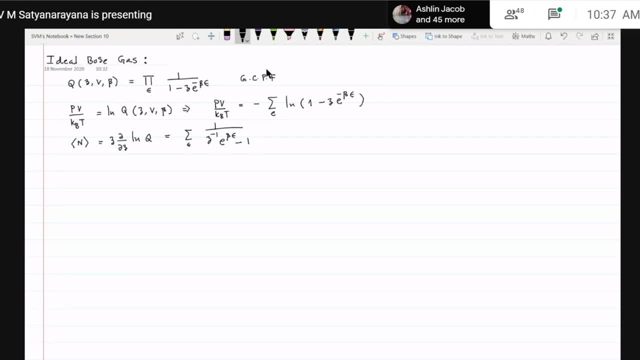 Okay, so these are our starting expressions, because this is something which we already saw in the last class for bosons, for this is grand canonical partition function for Bose, Einstein statistics, And from there we can get an expression for PV And notice that between these two equations there is a function for P and there is a 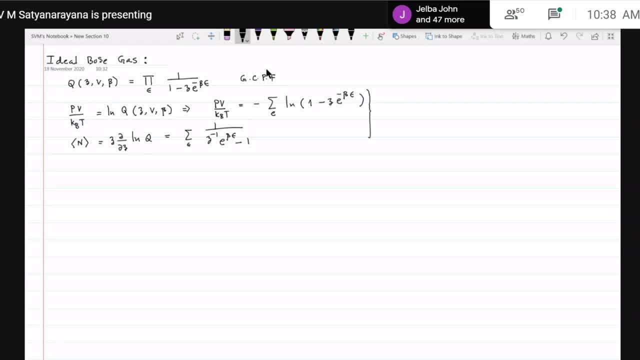 function for Z. Okay, so by eliminating, by eliminating the fugacity between these two equations, we get an equation of z. So last time, briefly, we discussed how to do this. It cannot be exactly done in many cases, so it has to be approximately done. 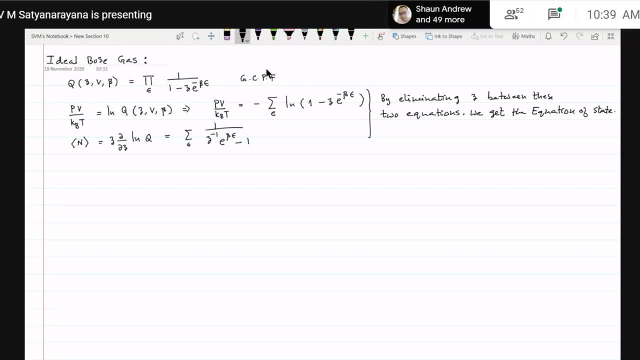 So this is just a procedure, how to get equations. Now we are interested in, So we are interested in, what is called a thermodynamic limit. so, since we are interested in thermodynamic limit which lets n tends to infinity, v tends to infinity, such that 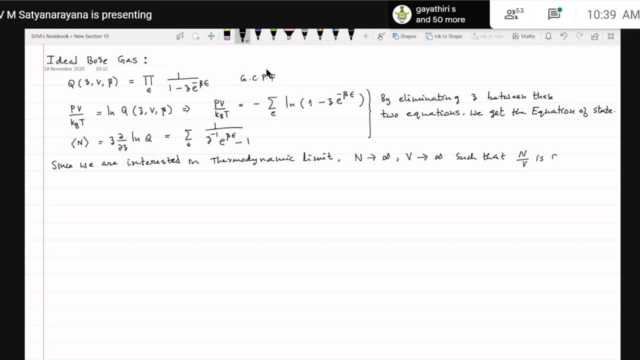 the density under density is finite And normally you can see that v dependence, v dependence, v comes to infinity. That is single particle energy. single particle energy, for example, as we have seen, for example, for a particle in a 3D box of volume, v allowed by use of energy. 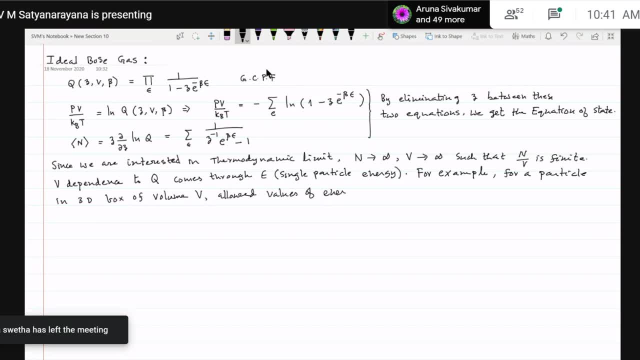 Okay, Allowed by use of energy, are given by h bar square, pi square into n1 square plus n2 square plus n3 square. These are three quantum numbers divided by twice n l square. but l square is basically v to the power 2.. 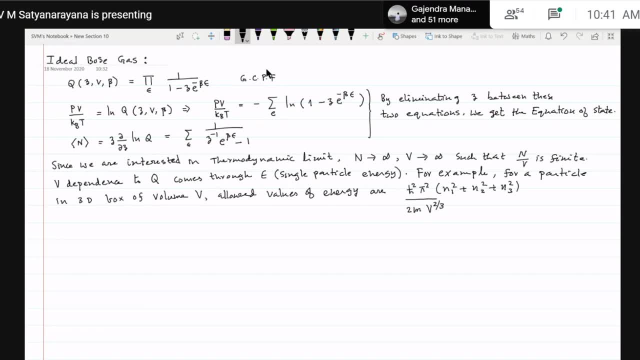 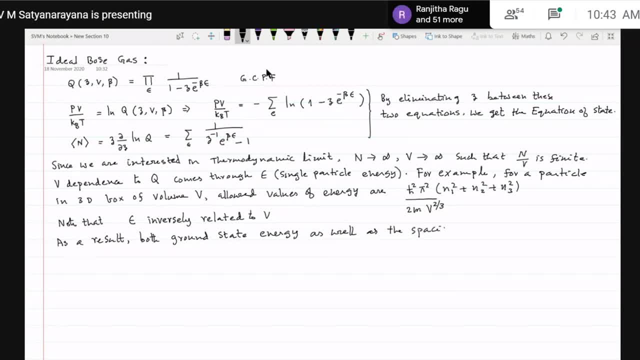 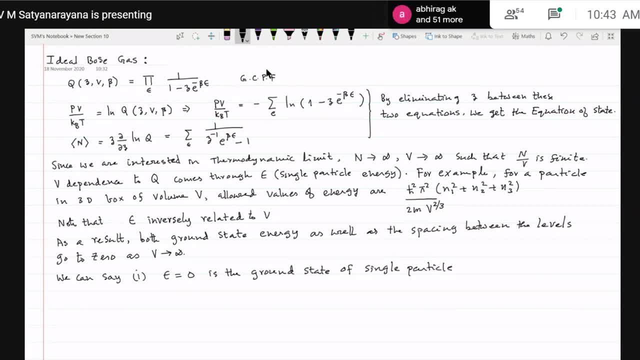 energy. Now the second thing that we can say is that since, since in thermodynamic limit energy spacing goes to 0, energy spacing goes to 0 implies some sums can be converted to integrals or integrals. So this is the number of integrals. 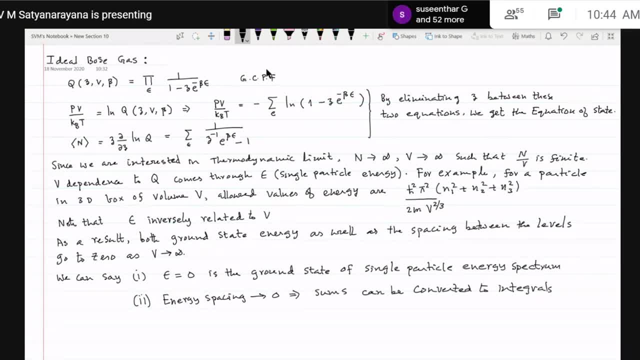 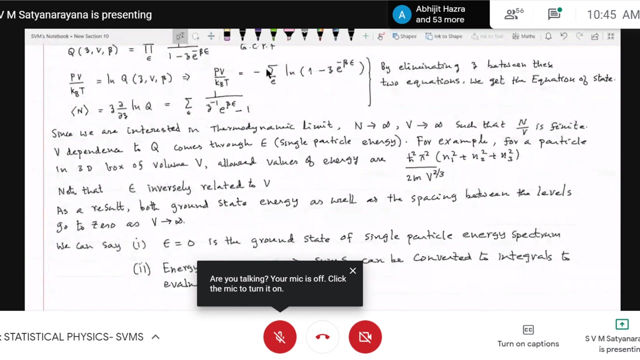 Okay, to evaluate proper. Now. this is important because integrals are easier to handle mathematically. So if we can convert these sums into integrals, then you can evaluate properties with ease. But there is- this part came for discussion earlier also- So whenever you have, let us. 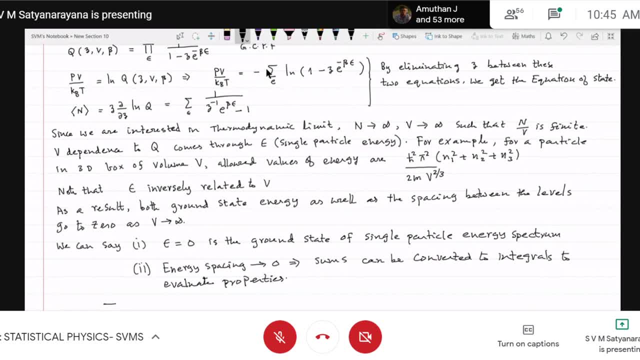 say sum over single particle energy, and then there is some expression here. whatever is the expression, Now this has to be converted into an integral. that means this has to be evaluated by integrating. So let us call that as some A of epsilon, and then same expression, and can write So: 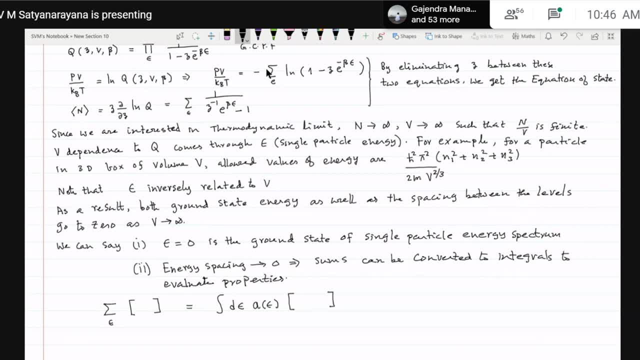 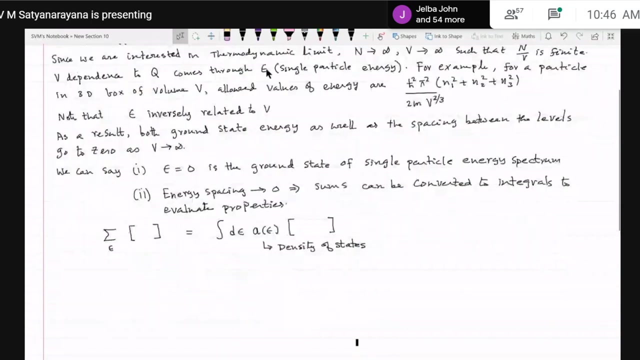 this is how we convert a summation into an integration using the density of space. So this is what is called density of space. Now, it is easy to define this. Suppose, let us say that you have certain energy levels in this fashion: I am drawing them like this. So I am drawing them like this. So let us. 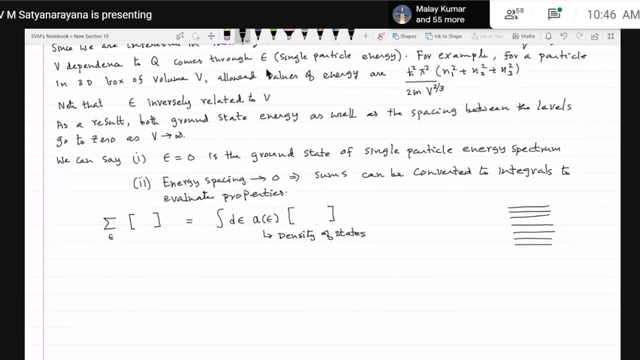 say that you can take this. So let us say that this is some kind of a energy E, and then you have a small window of energy E. So the shading is this. This is the epsilon. Now you can ask a question. 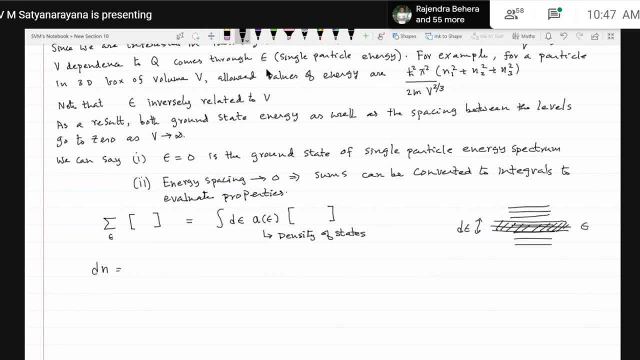 Let us define this dn to be number of energy levels or energy states in energy interval or energy range, whatever you call energy range d epsilon around epsilon. That is what I am going to define it as dn. Now you can. you can easily understand that this is equal to. 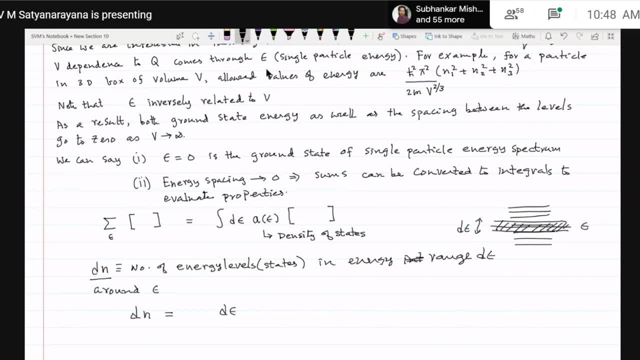 it should be proportional to d epsilon, Because you take bigger, smaller window, you get more levels. You get smaller window, you get less levels. But then this is also proportional to something which actually can change with energy. Okay, so that is what is called density of states. Like you know that, if you take, you take something. 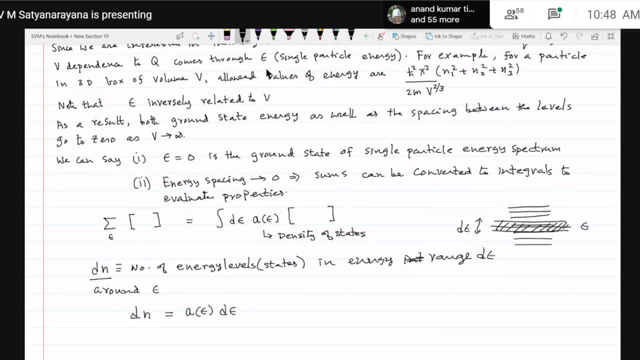 like hydrogen atom, initially ground state, first exited state. the spacing is more And as n is increasing the levels become crowded and crowded and crowded. So your A of epsilon will actually increase. That means as you go to same d e that that window is same size. 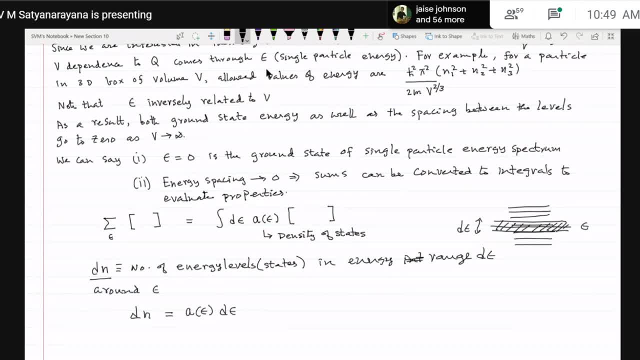 But if you are taking very close to ground state, you will have less number of levels in that window. If you go to higher value of n, you will have more and more states will be there. So that is what is your density of states. So we have given some more of. 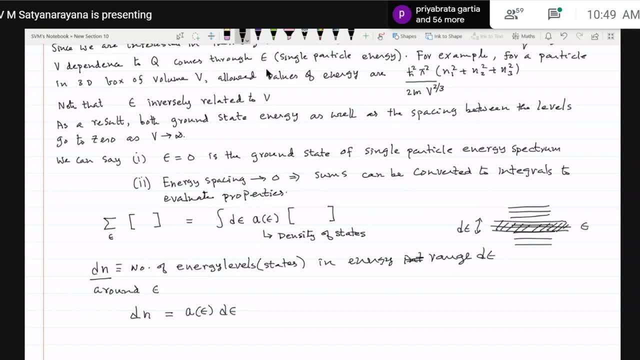 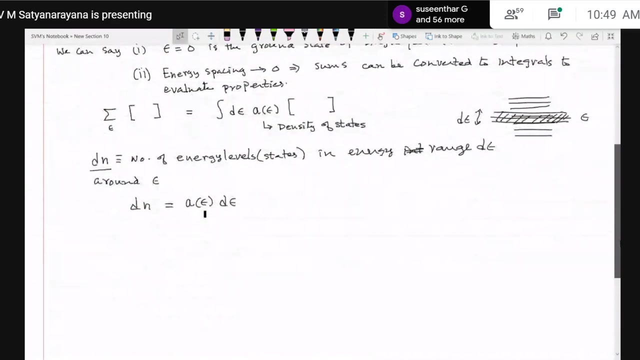 the values. So we have to evaluate this density of states in order to- in order to calculate these properties, because these properties we will calculate by converting the sums into integrals. So our first step now is to find out the density of states. okay, 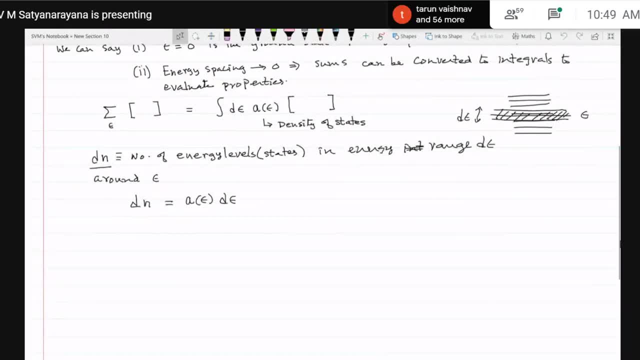 So we have- let us say this is our first step- density of states for Africa, because we are having an ideal gas, and ideal gas is the collection of people. Okay, So this is simple, or a free particle. The energy is given by h bar square, k square by 2, where h bar square, where k square is basically h bar square by 2m. 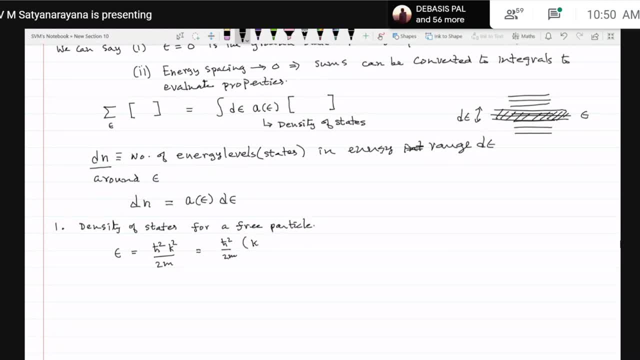 Okay, So in k square is you have three quantum numbers: kx square, ky square plus k dash square. Okay, So you notice that in k space, in k space, each, each point is equal to h bar square. 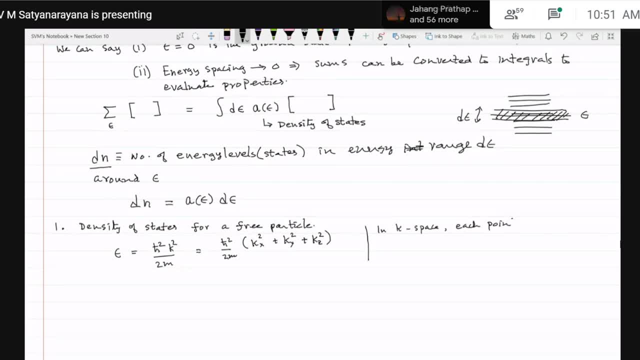 Okay. So in k space, each point is a state. Okay. So if you want to find out how many number of states are there or how many number of points are there it is, it is better to go to k space and then work out. 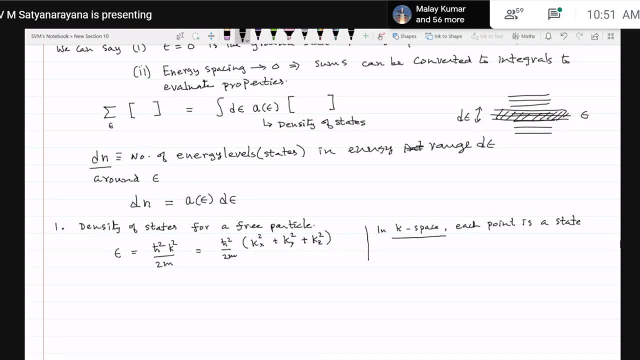 Since the energy depends only on the magnitude of k. so it is- it is easy to ask this question- that if you have in k space, let us say you have a sphere of radius k, Okay, So let us call this as a sphere of radius k. and then let us say you have another sphere of radius. this, this, this. 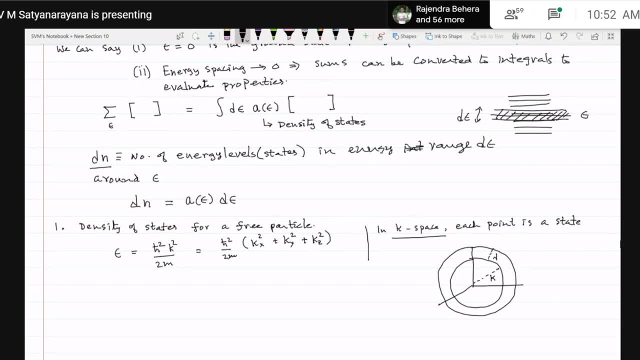 This is dk. So if you want to ask a question that what is dn? that is number of states. So this is proportional to dk, but then it is also proportional to let us call this as some g of k. Now I have to find out what this g of k is. 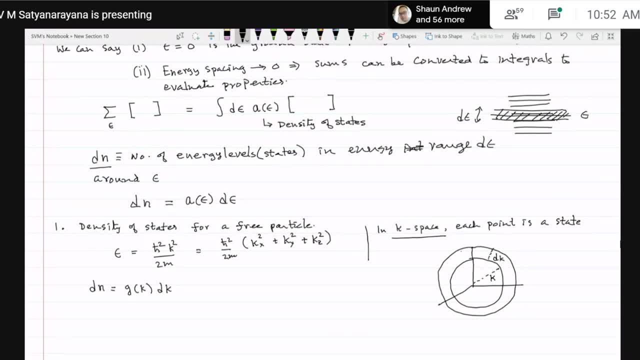 Now this g of k is essentially, you calculate the volume of this annular region. Okay, So this volume of the annular region, and so that is equal to 4 pi k square into dk. This is the volume, Okay. 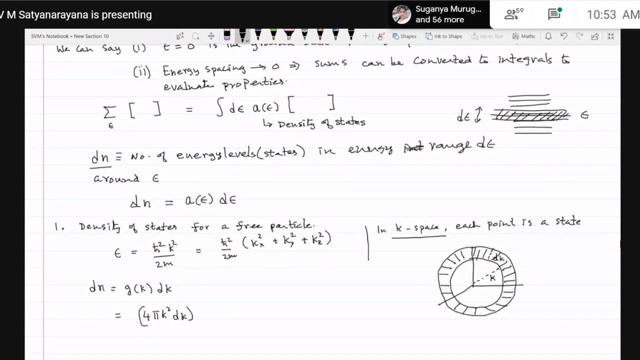 So if you have, if you have, so you know that if you have a point in the k space, the volume associated per point. Okay, So volume per, basically it is a k space volume. Let me call it k volume per state is given by 2 pi whole cube divided by d. 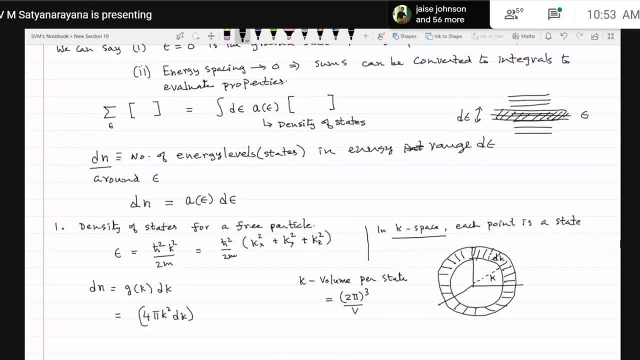 Basically it is 2 pi by L. L is the lattice constant and 2 pi by L is the whole cube. Or in other words, you ask number of states, Number of states per unit. k volume is just a reciprocal lattice 3 by 8 pi cube. 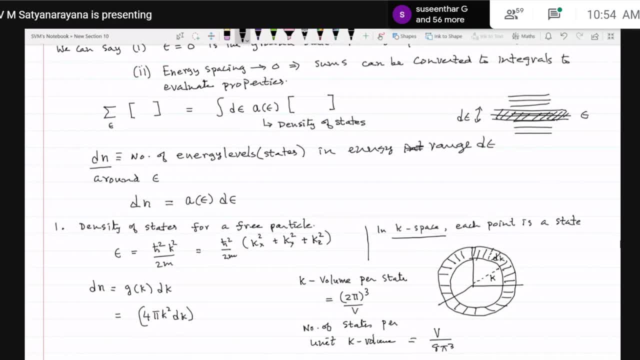 So this much is the, this much is the volume, and this is the number of states per unit volume. So you have, you have this, You have this expression, So your dn is equal to this, but this is not yet the density of states in terms of the energy. 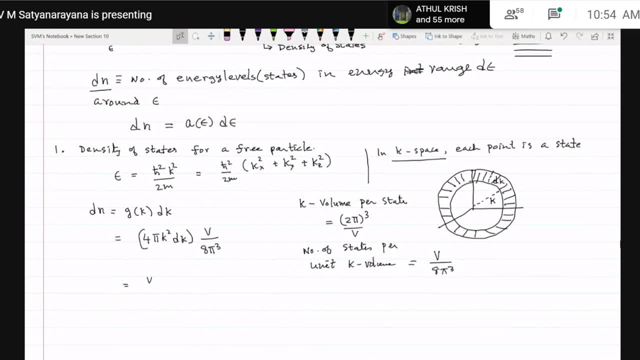 So this is equal to v divided by. So there is a 4 here and pi here. So v divided by 2, pi square into k, square into dk. But you know that energy is given by, energy is given by h bar square, k square by 2m. 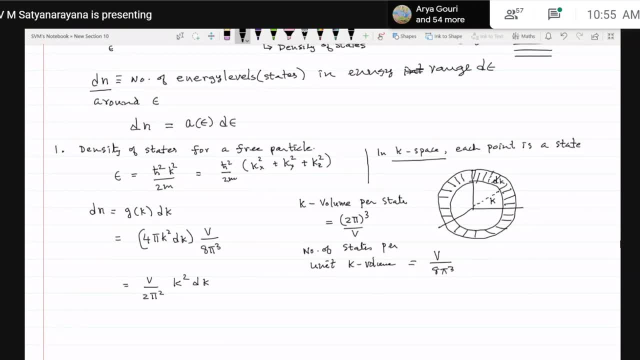 So k square is twice m by h bar square into epsilon. And what is dk? So k square is equal to twice m by h bar square into epsilon. Or your k is equal to square root of- Okay, Square root of twice m by h bar square into root of epsilon. 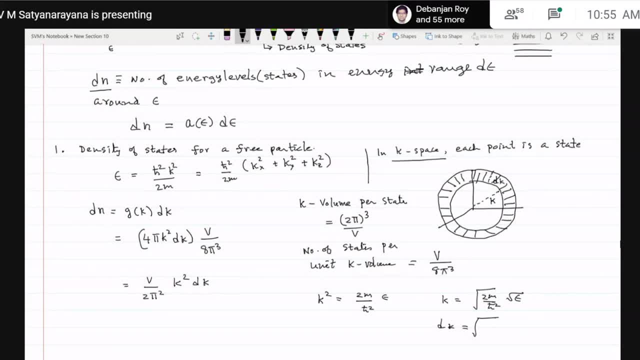 So dk will be equal to square root of twice m by h, bar square into 1 over 2 root e into b, epsilon. So if I substitute that one here I have v by 2, pi square into twice m by h, bar square to the power 3 by 2.. 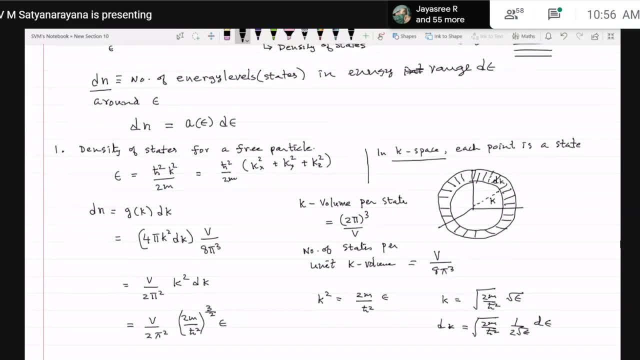 And you can class it k. k square is equal to 3.. But not twice m by h bar. square into twice m by 2. pi square into 1 over 2. pi square into 2 into b. Okay, So k square is equal to 1 by into k square into 1 over 2 pi square into 2, int 줄. 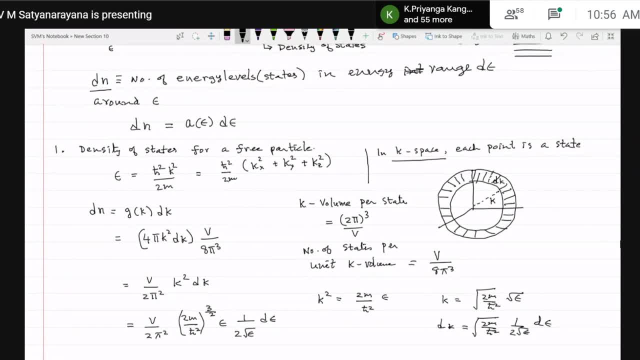 So 2 by 2 pi And 2 is equal to 3.. Okay, So eat a 2 by 1. And 2 by 2 times m by h bar square into 2, int 줄 Okay. 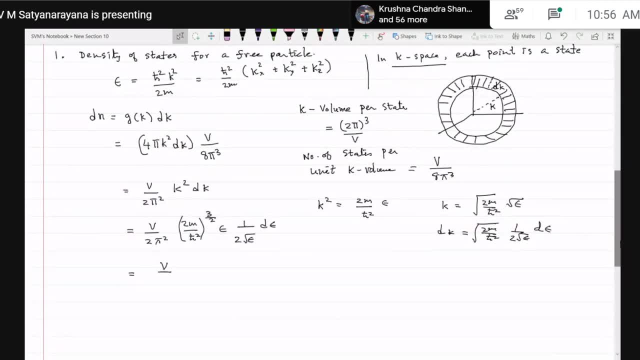 One over 2 pi. Ok, Now we have a sign here, So this has stopped here. It is the same number over here. This is the 2.. No, Because every SCSH actually gives the same number and number of m. 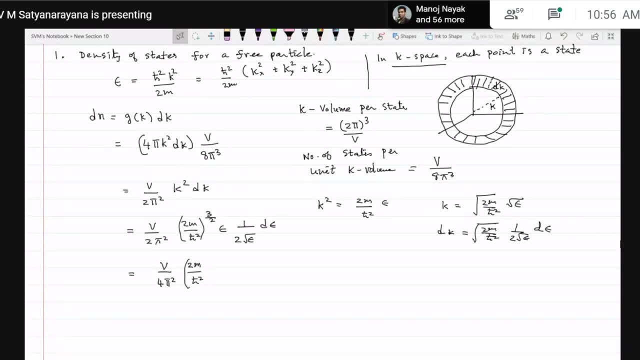 That is the same power, e by 2 into root epsilon, d epsilon. So you could have also written this as, or whatever I called as, k of epsilon into d epsilon. So from there I can read out: the density of states, k of epsilon is equal to e divided by 4 pi square, into twice m, by h bar square. 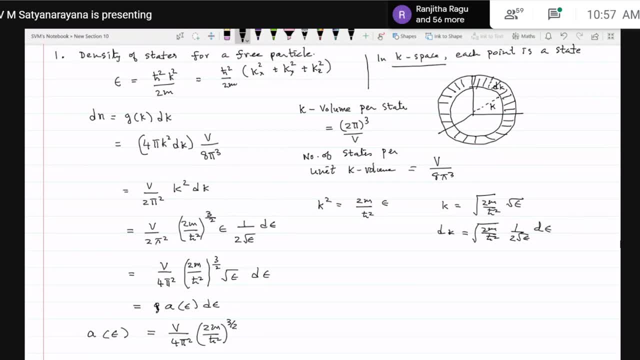 to the power 3 by 2 square. So this is the density of states of the three particle in three dimensions. So I must say that this is density of states in three. So I will not look at density of states in other dimensions. 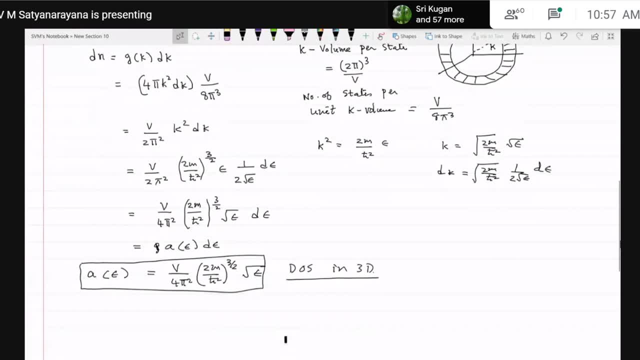 Today we can work, you can, you can see that eventually move it as an exercise, useful exercise. today We did so. a of epsilon. So let us call generally in d, dimension a of epsilon is equal to. you will have some constant which will depend on the dimension C, D and then 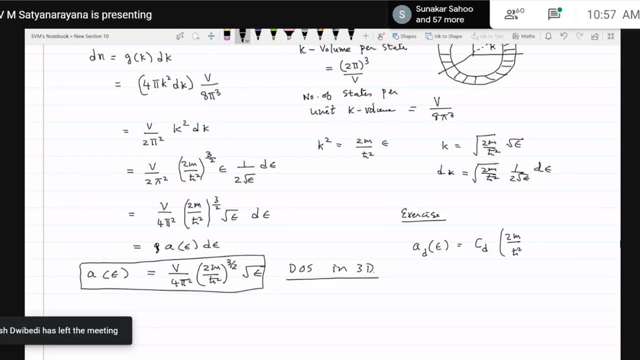 we have twice m by h bar, square by the power, d by 2 plus m by h bar square into d, epsilon, and we will have epsilon and e minus 2 by 2.. So this is the general expression. So in two dimension the density of stress will be independent of energy. In one dimension it 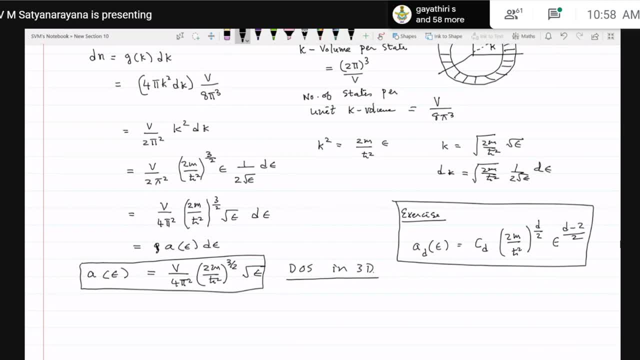 will be epsilon to the power minus half. So this is the general expression. but this is important. So I would recommend that you can try to, at least in two dimension and one dimension. it is easy to show, So from that you will be able to make a general expression. 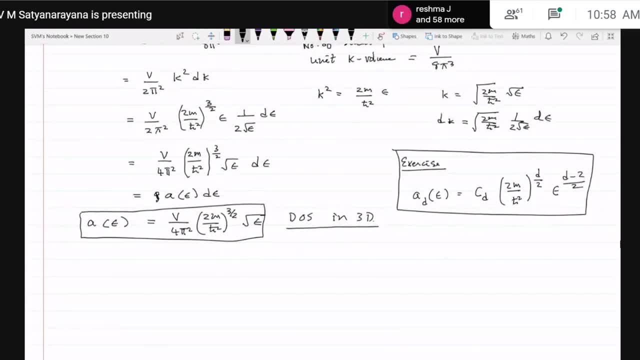 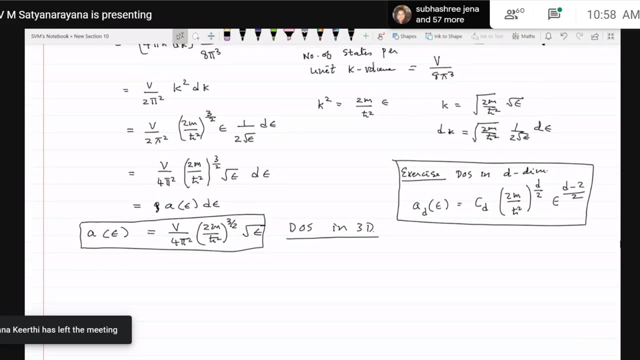 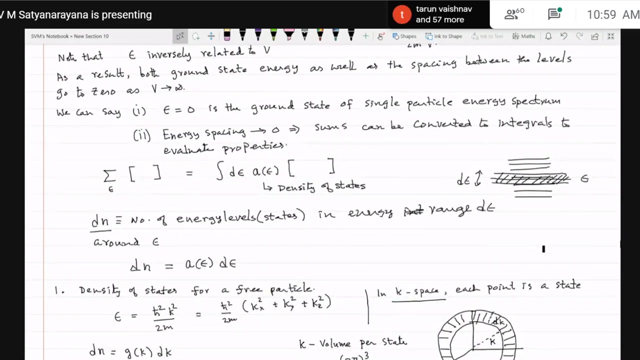 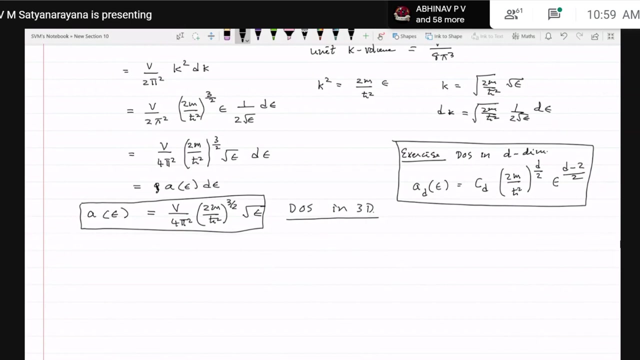 like this. So this is density of stress in two dimension, Okay, Okay, So we have this expression. Now we are ready to write down our expressions for n in terms of n and pv by kp in terms of it. So first let us look at so in the second part we will try to convert. 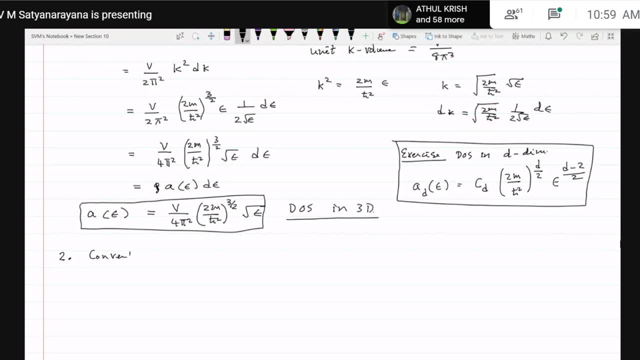 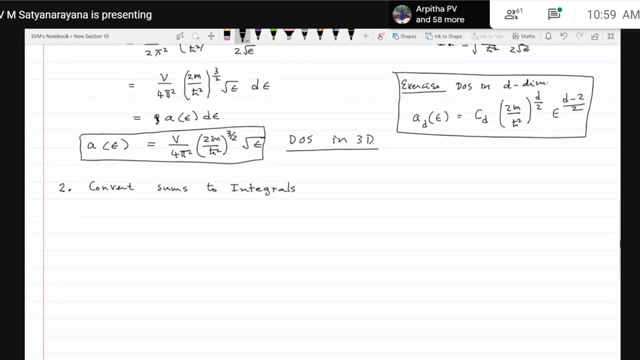 convert m, m, m, Which geschrieben? which row, which row, which row, tet, tet. So first let us try to convert its average number of particles. So we'll consider, consider, n, n, and, And do, dot, dot, dot, dot, dot. you know, average number of particles is equal to sum over single particle. 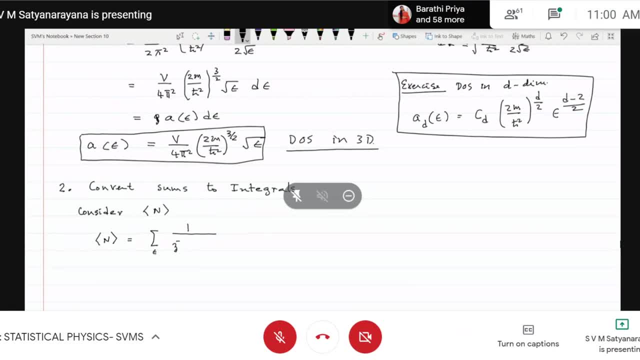 energies. 1 divided by z to the minus 1, e to the beta epsilon, which I would write it as integral. we are starting from 0 to infinity integral 0 to infinity b epsilon into I have this: a epsilon which is given by v divided by 4 pi square. 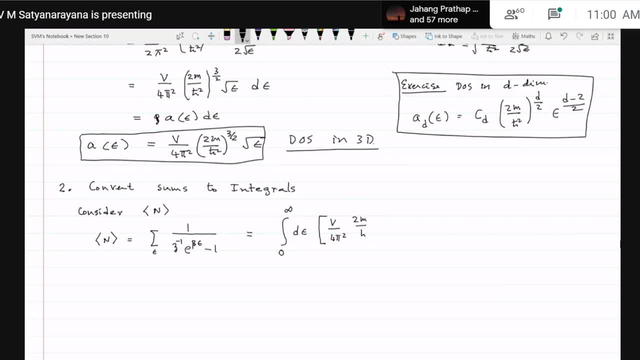 into twice m square to the power, 3 by 2 into root 1. this multiplied by z to the minus 1, e to the beta epsilon minus 1. okay, so now what happens? look at this carefully, look at this expression carefully. the argument- what I am going to present here is argument- is the following: that what happens to so 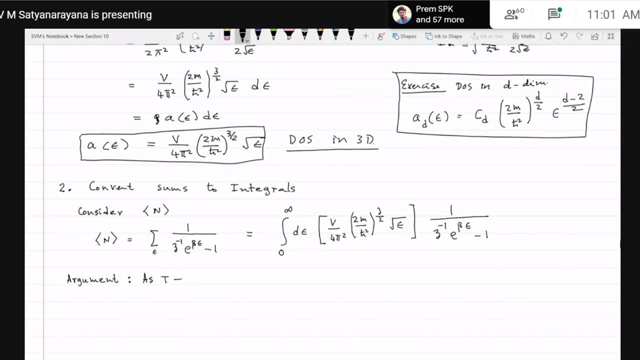 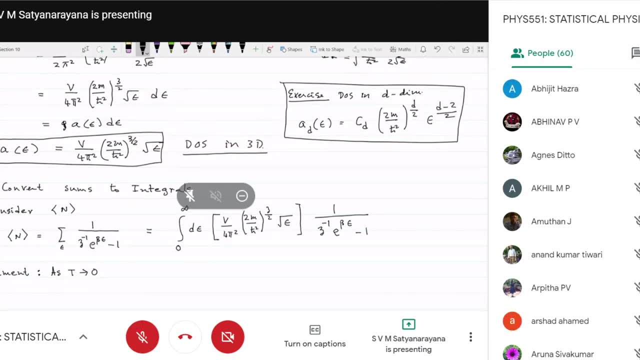 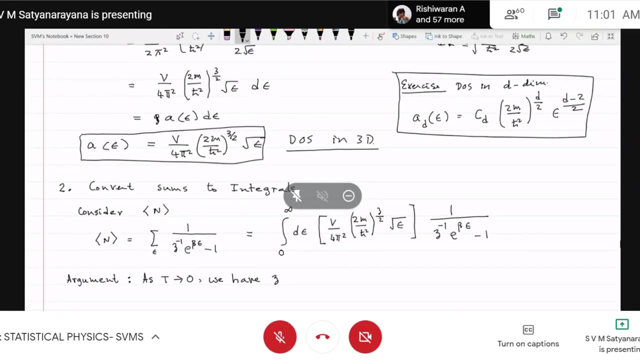 as, for example, t tends to 0. okay, I see. tends to 0, we have this fugacity: tends to 1, okay s. t tends to 0, you guys, t tends to 1. now, if you consider brown state, that is, the, the Epsilon is equal to 0, the ground state. 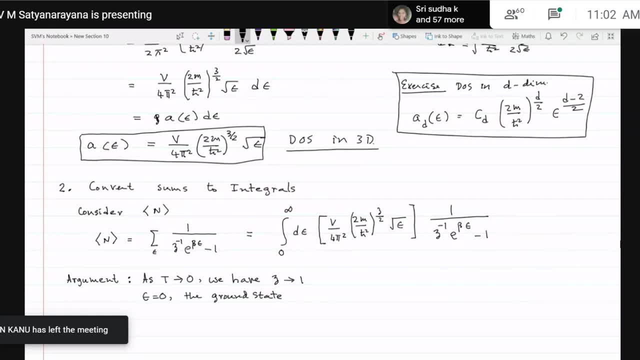 Okay, if you consider this, then this term 1 by e to the beta epsilon minus 1 is like 1 over 0. It goes to 1 over 0 because epsilon is equal to 0. So this is 1 minus 1, this is 1 over 0. 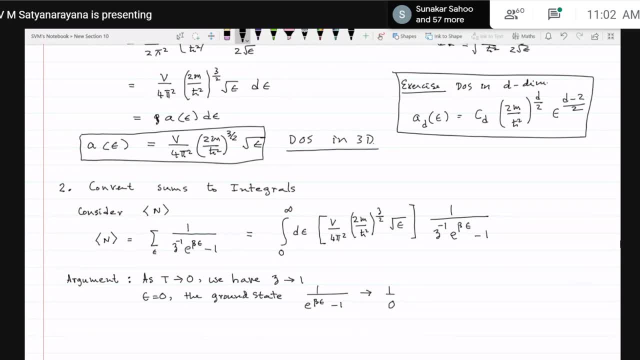 Whereas our root epsilon is also equal to 0. So, because of that, what happens For epsilon is equal to 0, that term We have an indeterminate form. We have something like 0 divided by 0. Okay, so this is a little inconsistency there in mathematics. 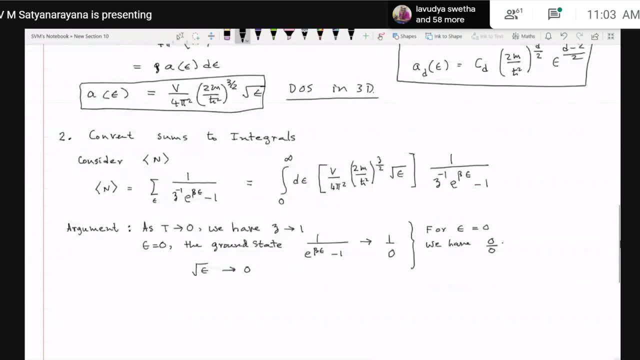 So what we can do is we will try to write it in the following fashion. We will write: let us rewrite: Okay, Let us rewrite this: n average value of n to be suppose, if I take epsilon, equal to 0. 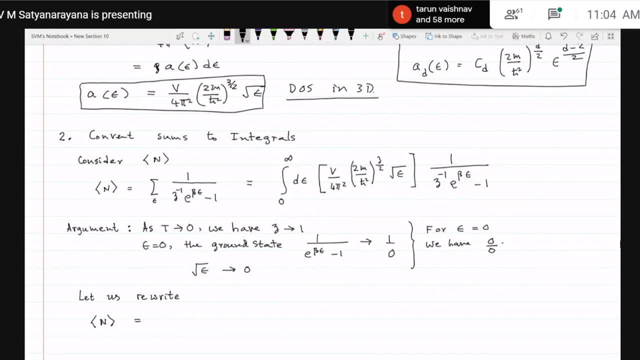 Okay, So then I will have that term. I will write separately. That is z divided by 1 minus z plus. Now I have Epsilon greater than 0 and the same term, The summation Statenffer's, using the beta epsilon. 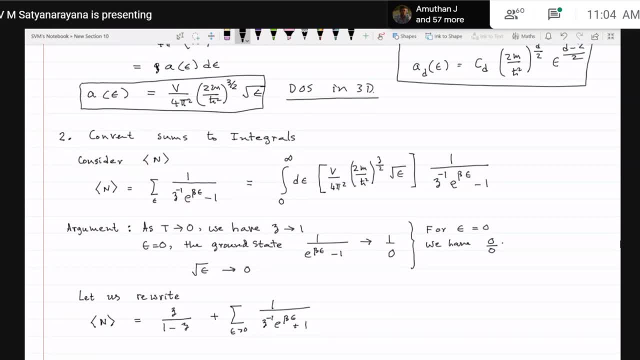 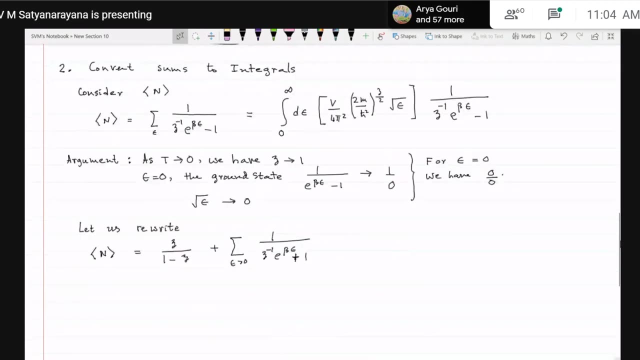 Okay, Now you can see that. You can see that the. You can see that the. So you leave this. So this is somewhat like this, Sir. Yes, Sir, why plus 1?? Sorry, minus 1.. 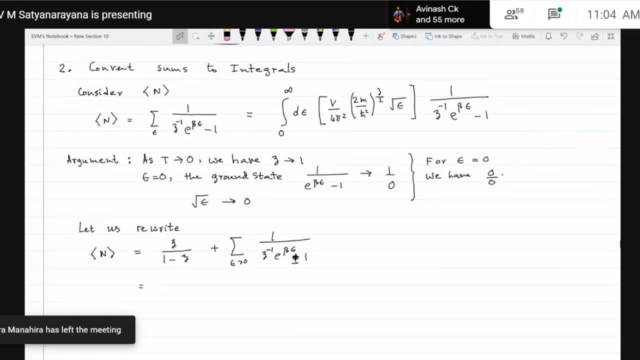 Minus 1.. So this is like saying that this term is the average occupancy of the ground state And this term is the average occupancy of all the excited states other than the ground state. Okay, So you can say this is average number of, average number of bosons in the ground state. 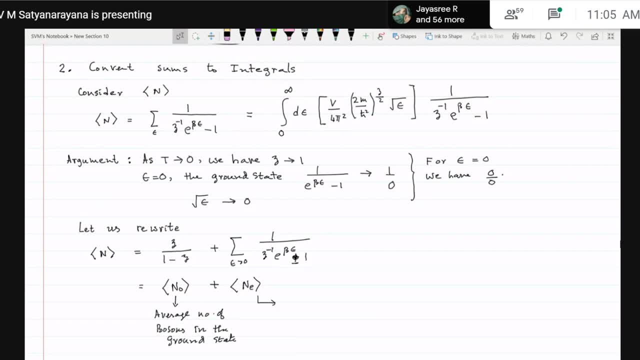 And this is average number of ions. So this is the average number of particles, number of bosons, in all the excited states. Okay, So this is kind of an interpretation that we can do to these terms. Now note this: that this term, that is 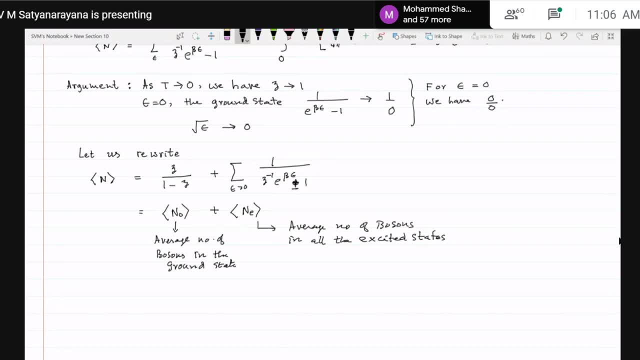 leaving this term, I can write average in E as sum over epsilon greater than 0 into 1 by t-inverse over the beta epsilon minus 1.. This I can now write it as VB. So VB by 4 pi squared into twice m by h-squared squared to the power 3 by 2. 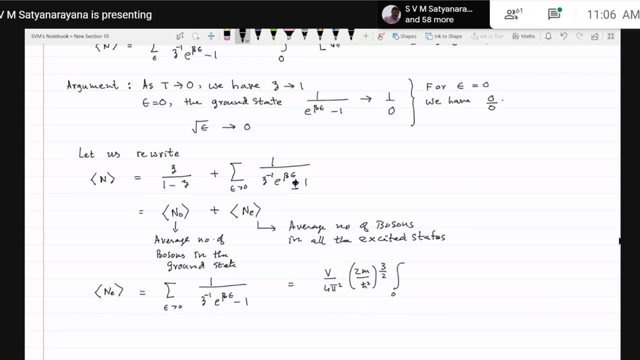 and integral 0 to infinity of E epsilon by root of epsilon to get to the minus 1 into the beta epsilon. Okay, Okay, Now I can still keep this. I can still keep this limit from 0 to infinity, because now this epsilon the energy level. 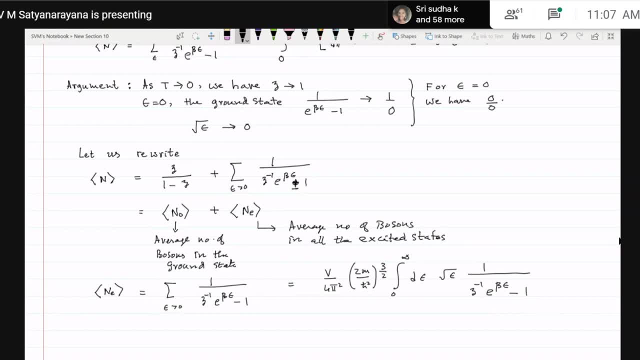 is every other level other than the ground state. But even if I include, however, closer energies, this density of states is going to be very small for that, So it will make a negligible contribution. So what I am trying to say is, if you plot, if you plot A of epsilon versus epsilon, 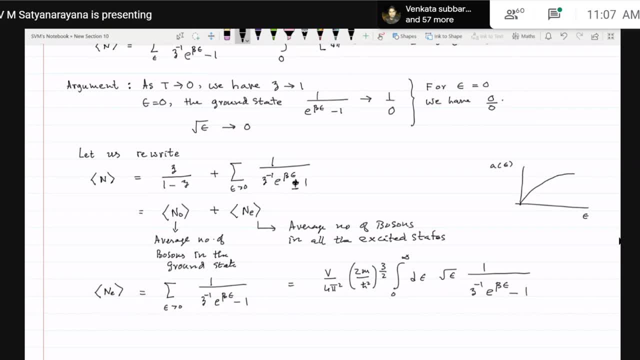 this is something like this right, which is basically square root of epsilon, So very close to energy level. the A of epsilon is very close to 0.. And hence, if I, even if I put this limit to be 0, I will not really make much of a. 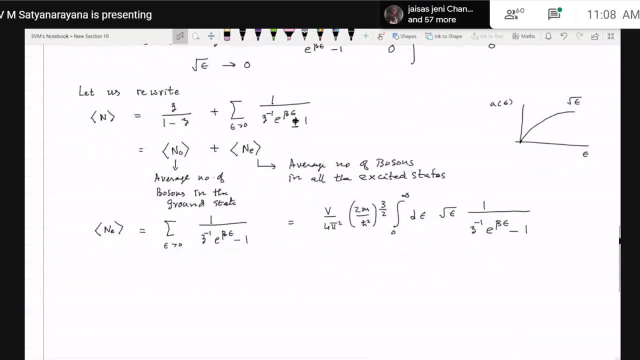 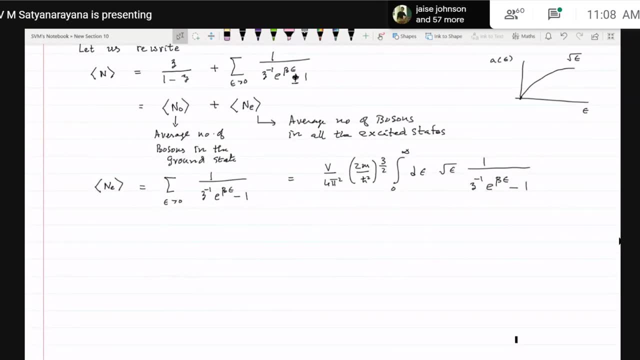 contribution for this integral. Now, this is the integral that I have to evaluate, So now I can write. I can write the integral in the following fashion: So let us say that substitute, substitute beta into epsilon to be equal to, so this: 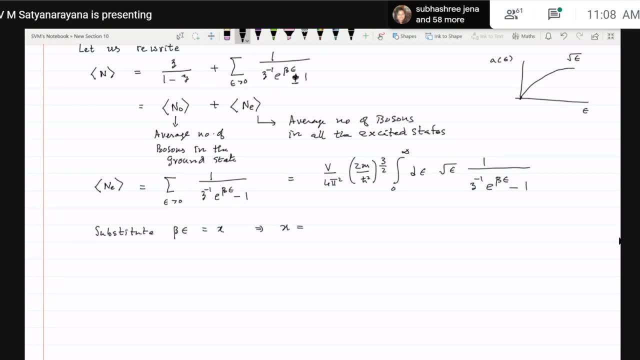 implies x is equal to. I mean epsilon is equal to, So x by beta and d epsilon is d x by d t and root epsilon is root x by d t. So now you can see in terms of this, this m e is equal to v by 4 pi square. 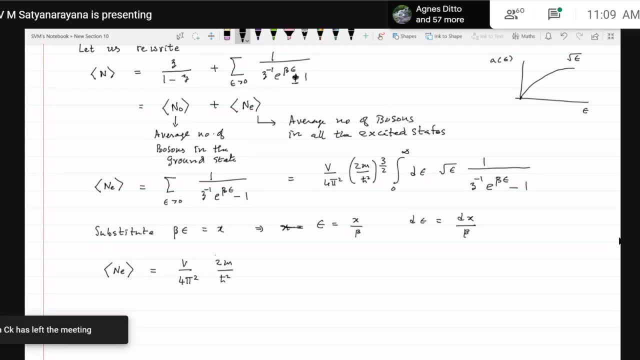 twice m by h, square, square to the power 3 by 2.. And so I get 1 beta from d epsilon, 1 by root beta from here. So that is equal to 1 over beta to the power 3 by 2.. 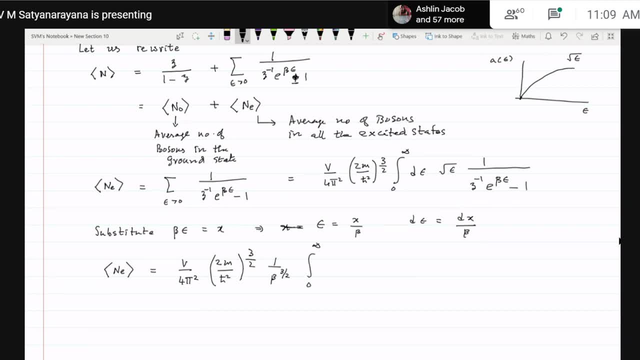 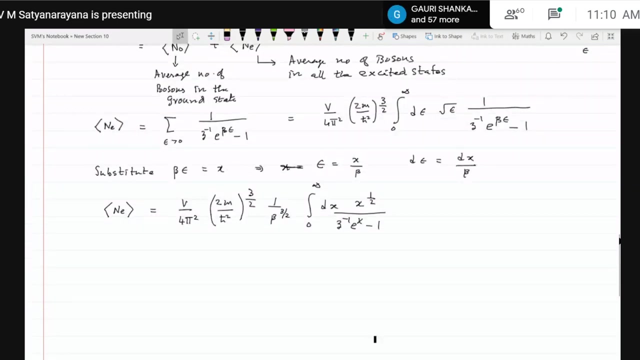 And the limits don't change: dm x into x to the power half divided by z, inverse e to the x minus 1.. Okay, So now you can. you can see that we will be able to define a class of functions called 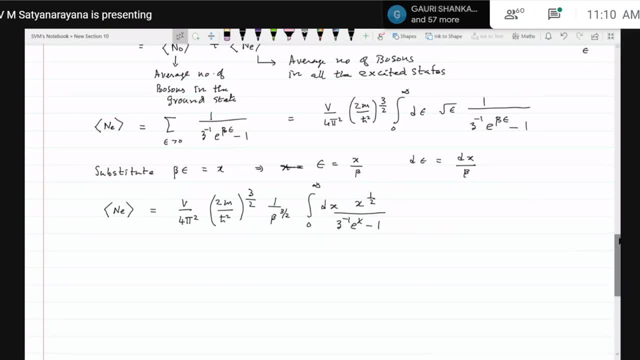 Bose-Einstein functions. So let us define, define the class of functions which I will call it as g? mu of x. So this g? mu of x is defined by the state, the state hat, which I have defined in my. 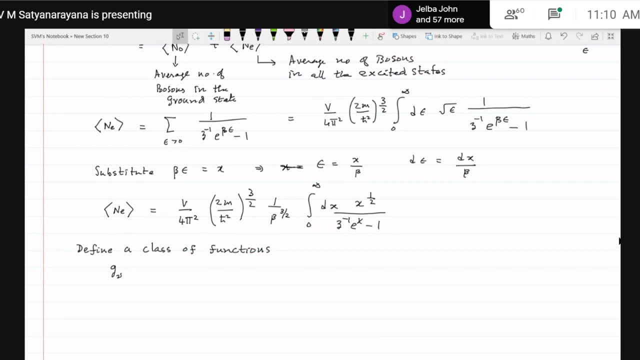 two previous suppliers, the five krijumasum These words. They are called kline Right. So the kline, the state hat defined like this: 1 by gamma of mu, integral 0 to infinity x to the mu minus 1 dx divided by: 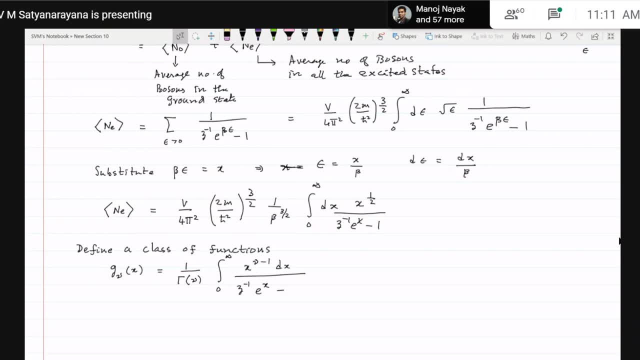 z inverse e to the x minus 1.. So, as you can see that this is a general, for every mu there is a function. So let us define these functions and see whether we can write. it looks like we can write this in terms of these functions, So for that, let us try to. 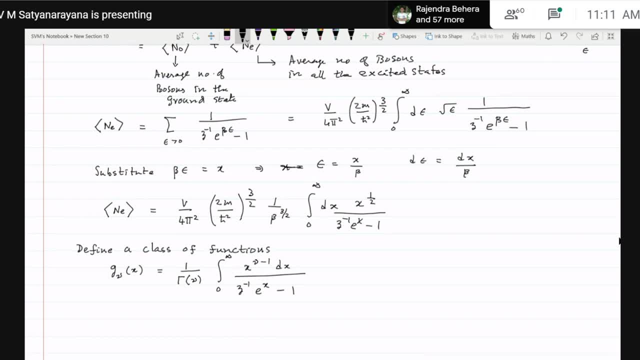 write this coefficients at once, Once we should expand them and then see what kind of form they go to. So let us write this average n. The average number of particles in all the excited states is v divided by 4 pi square. And then I will write this as twice m to the power 3 by p. And we know this: h bar is h. 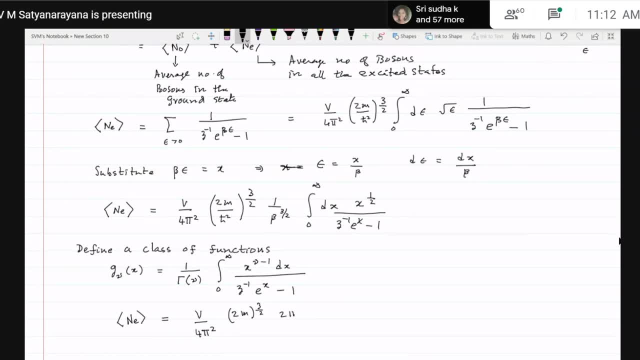 So there is a, 2, pi by h to the power, 3 by 2, and this is basically a, b, c to the power 3 by h, And then we have this integral: 0 to infinity, dx, x to the power. I will write it in this: 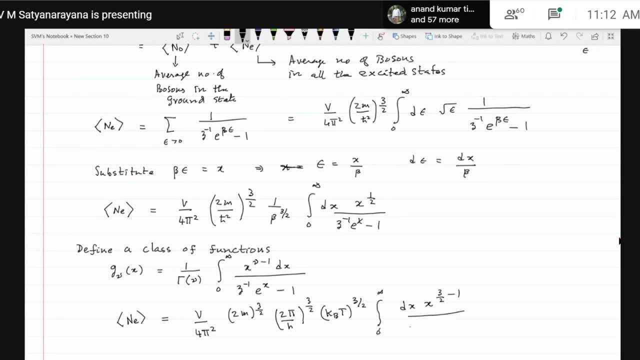 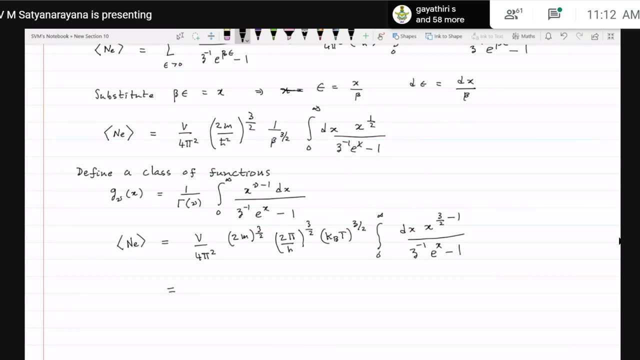 fashion: 3 by 2 minus 1, divided by z inverse e to the x minus 1.. So now my idea is that this is 2 pi to the power 3 by 2, and I have a 2 pi here, and so 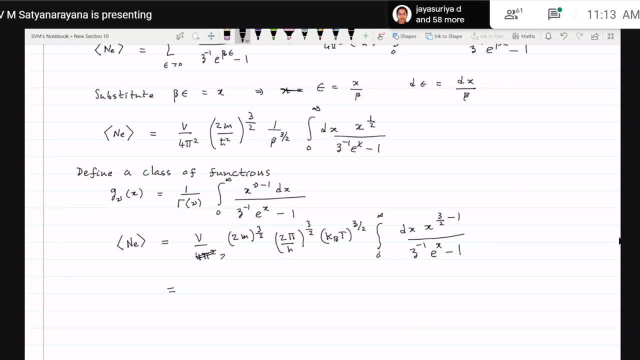 this is like 2 pi the whole square, correct? Let me write it as 2 pi the whole square, So that will be 3 by 2 minus, or I can write 2 pi. so let us keep this. so I want to write. 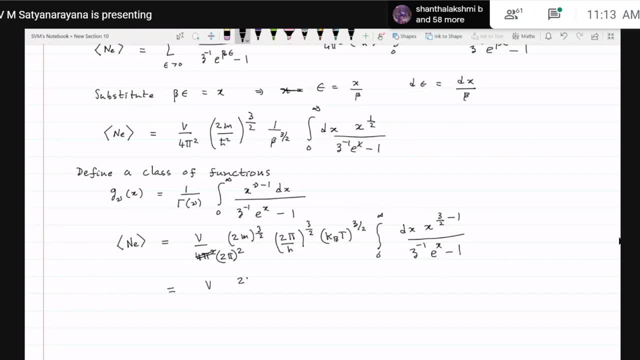 b into 2 pi m k b t. 2 pi m k b t. So there is a 2 pi here, k b t here and the m here. so 2 pi m k b t by. this is h square. 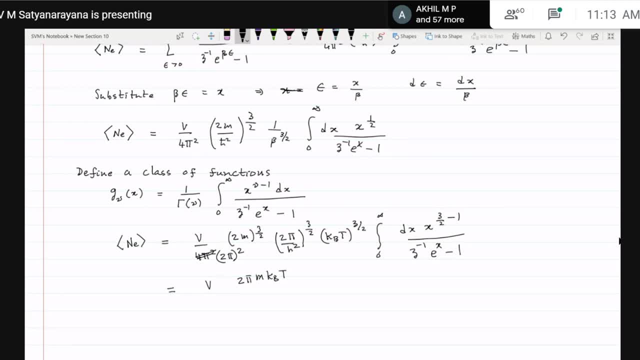 right, Yeah, that means this is h square and this 2 pi the square. okay, by h square to the power 3 by 2.. Okay, Now what is remaining Is I have from here- I have taken only m, so there is 2. power 3 by 2 is there and there. 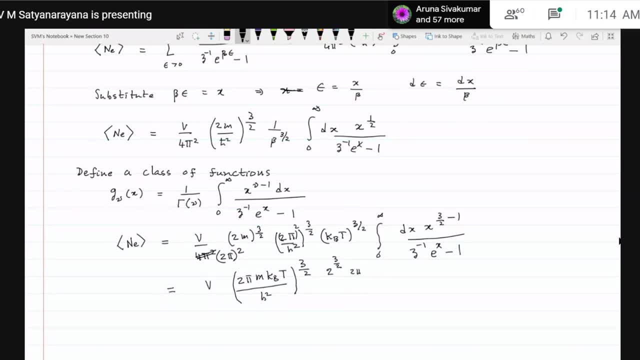 is one another 2 pi to the power, 3 by 2 is there and I have 2 pi the whole square. okay, So that means into this integral, So let me not write it. So this is equal to, but what is this one? 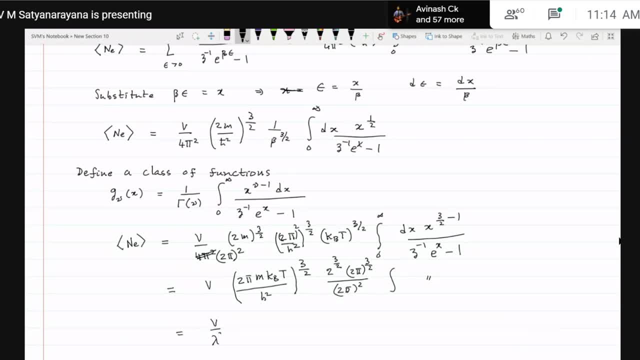 This is v divided by lambda cube. this is thermal deep gravity wavelength. So v divided by lambda cube and 2 power 3 by 2, 2 power 3 by 2, that is 2 power 3, and then I have 2 square. that means there is 2 there and pi power 3 by 2 by pi square. 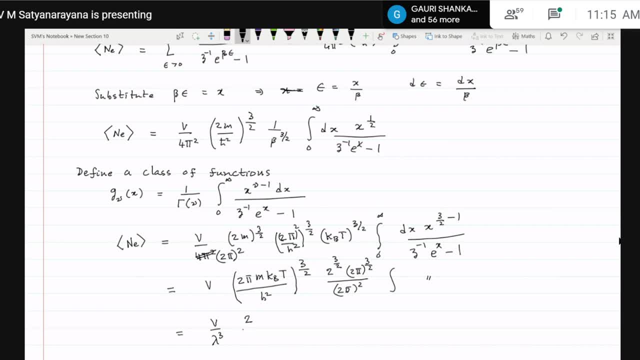 So if I bring that to the denominator, this will be 2 pi the whole square. Okay, So 2 pi root pi into 0 to infinity, dx, x to the power, 3 by 2 minus 1 divided by z inverse. 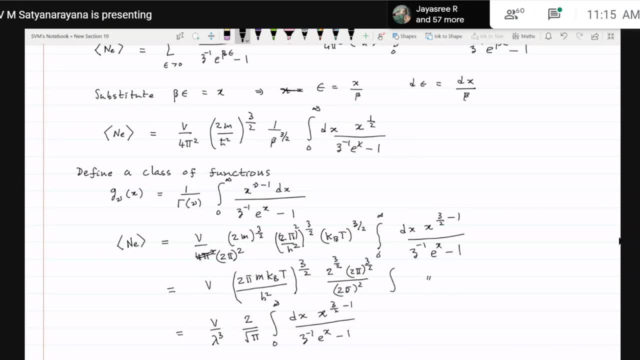 e to the x minus 1.. Okay, Now you see that your gamma of 3 by 2 is equal to 2 pi by 2.. Okay, So this 2 pi root pi can be written as half, gamma of half, so which is equal to root pi. 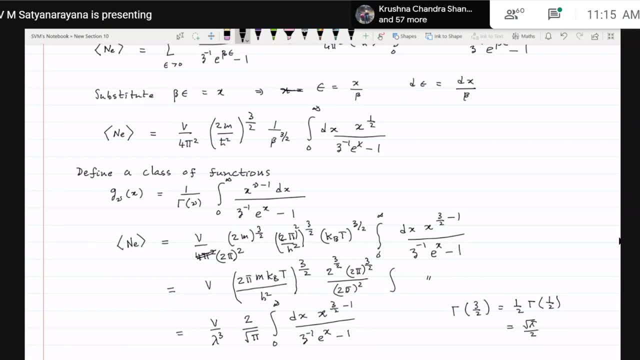 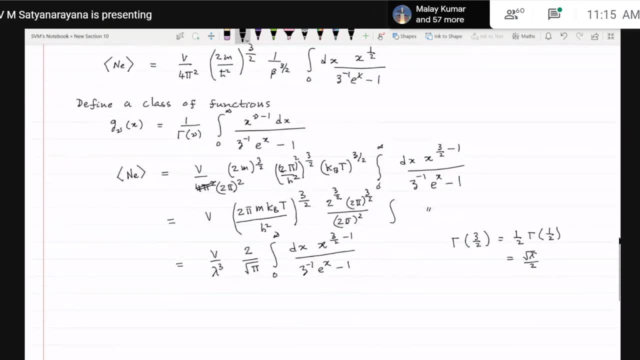 by 2.. So this 2 by root pi is like 1 by gamma of 3 by 2.. So this expression gives us, in terms of, in terms of the Poisson's 10 functions defined: So n, e is equal to v divided by z, inverse e to the power 3 by 2.. 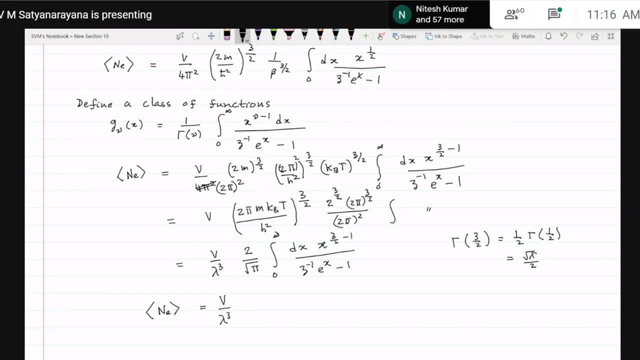 Okay, So v divided by lambda cube, v divided by lambda cube into g, 3 by 2 half. So I am sorry, I must write this as a function of z, because x is anyway getting integrated. So this is a function of the fugacity. 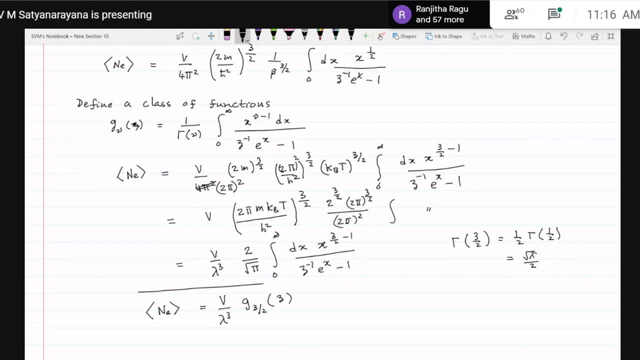 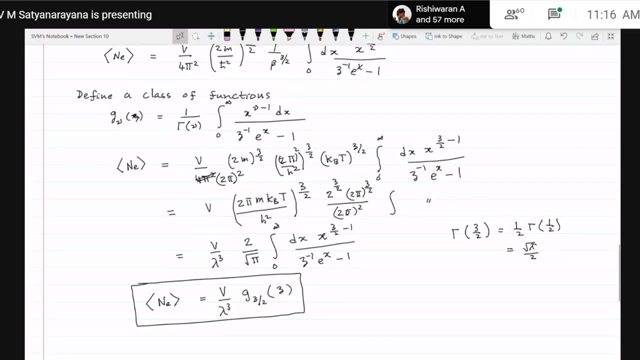 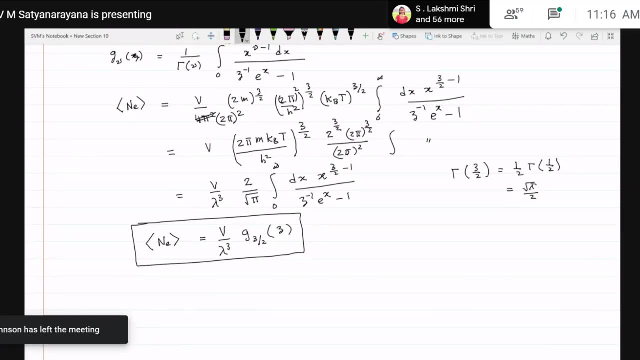 So this is the expression. So we have to do this once, but then we will remember Whenever we are doing problems, we will directly start from here. So n is related to this. So now let me just- okay, so we also go back to this expression- that p v over k t, p v over. 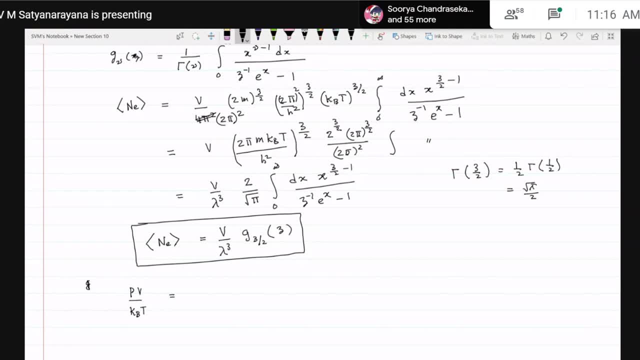 k, t is equal to sum over: Okay, Okay, Okay. So even have apow this little hello. Oh, no wonder someone scrolling toная toaff allow this to begin. what you do notify. So what are the following problems you are verifying? 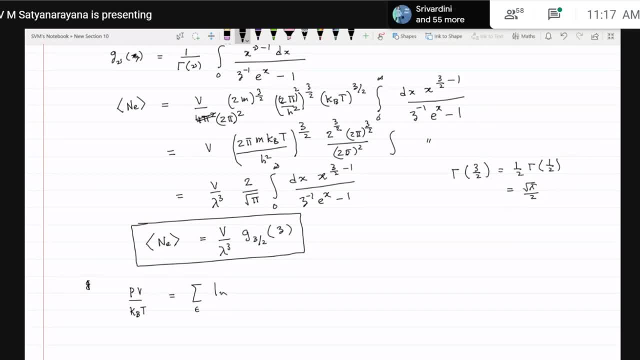 If you are having problem you need an example. Okay, So whatever you have have to be used. say you get e to the power of 2 by 2 into over k T, that then you have plus of k T into e to the power of 2 by 2 minus f return. 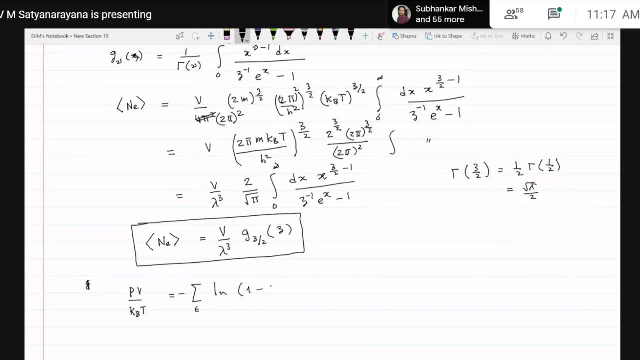 on plus e to the power of 0.. Okay, Now let us see the expression of this expression of okay, this example. So how do we get the explanation? essentially, we need to think of it in general: drug expression: okay. 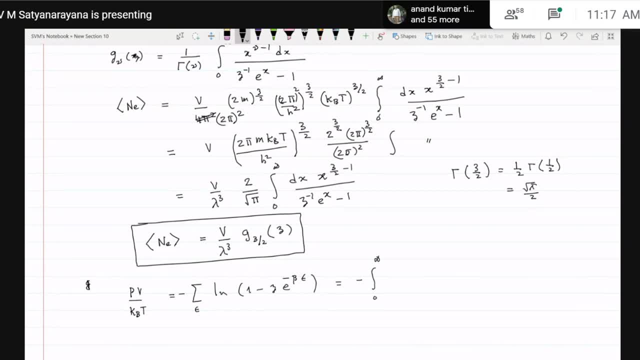 Okay, So there is. this powerful Good devel was written in one, consuming dozens of visuals, et cetera, et cetera. So you have the same density of states, 3 by 4 pi square, twice m by h bar square to. 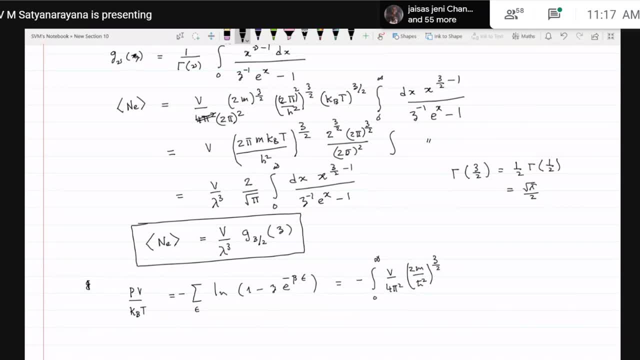 the power 3 by 3 and root of epsilon. so there is a d epsilon, which is density of states, into you have a logarithm of 1 minus 70 to the minus beta x. So I want you to do this, so let me just leave this as an exercise. So first thing is do an integration by parts. 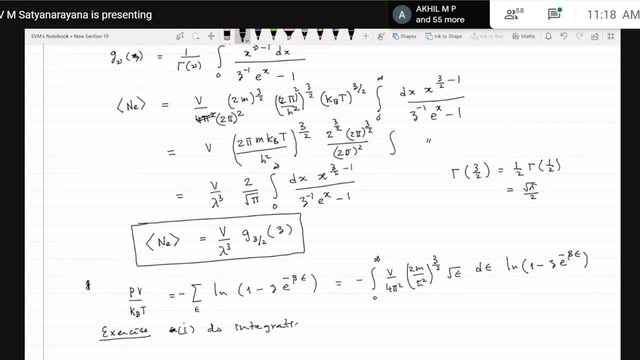 integration By parts to this above integral, where you are going to consider, u is equal to root epsilon and rest of the term to be d? v and d? u is equal to 1 minus z to the minus beta x. So I think you should consider d? v equal to this and u is equal to beta epsilon. 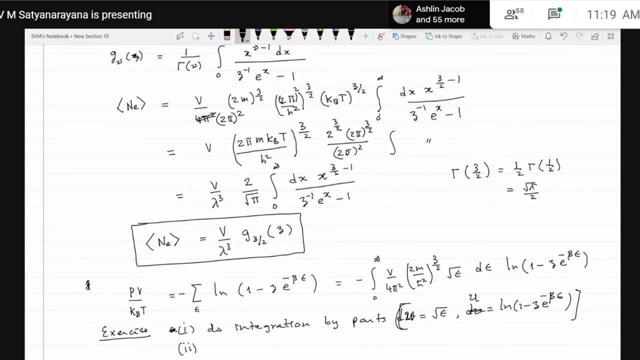 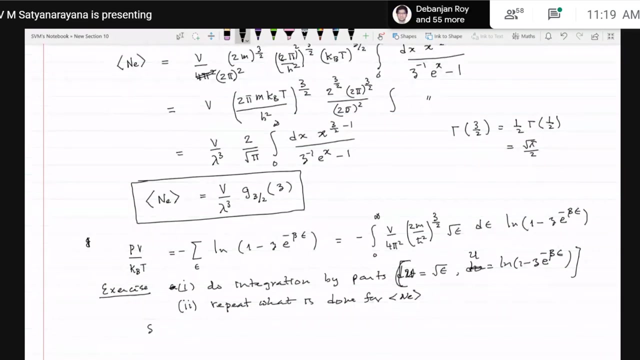 And then repeat whatever I have done, repeat what is done for what is done for average n above, and then you will be able to show that for that P by KB okay, so that the PV by capability that we will cancel on both sides, P by KB T is nothing but 1 by. 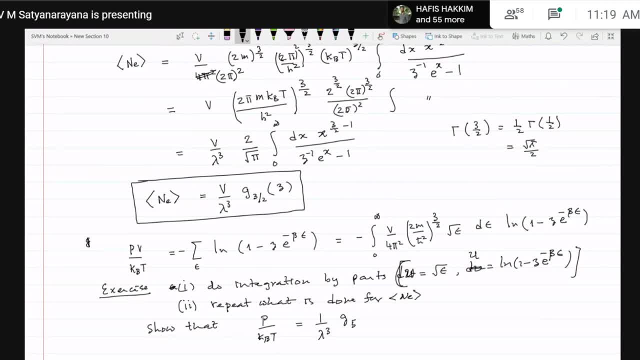 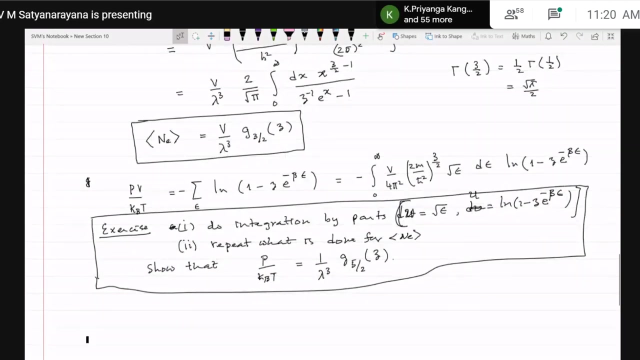 lambda Q into T pi by 2. so this I will leave it for you, okay. so now what we have done is we are, we have, we have managed to write this in terms of some general Bose, Einstein class of functions. now we will try to understand the nature of these functions. okay, so that will help. 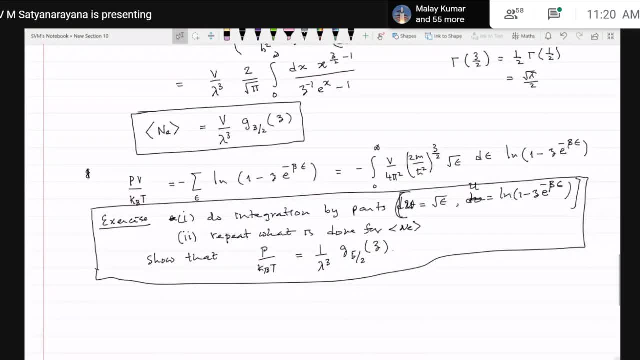 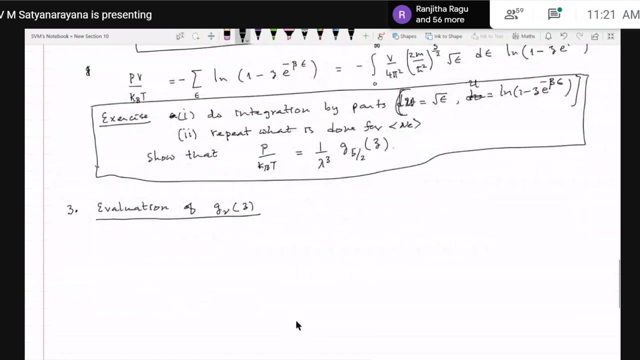 us to get an idea of what happens for an ideal process. so third is evaluation of evaluation of post, definite of Så how to evaluate this? remember, this is an integral at an integral, so we have to actually integrate. okay, so the integration is some thing like this: we have mu of t is equal to 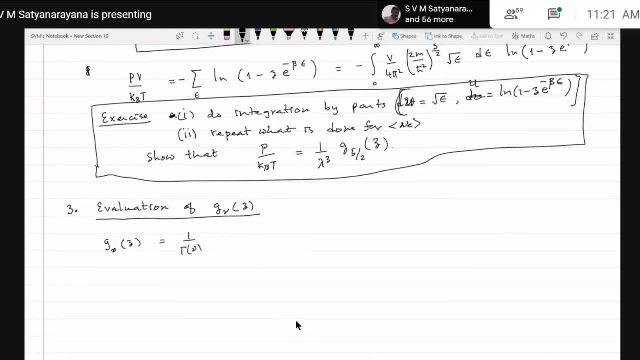 1 over gamma of mu. it is in the integration part. so integration, we have a mu of t. you see its, the calculation part come. so, and paraphrasing once again, inequality, you will calculate it. well, that is can be done. first vision, okay, except that never mind, ok, and then we will. 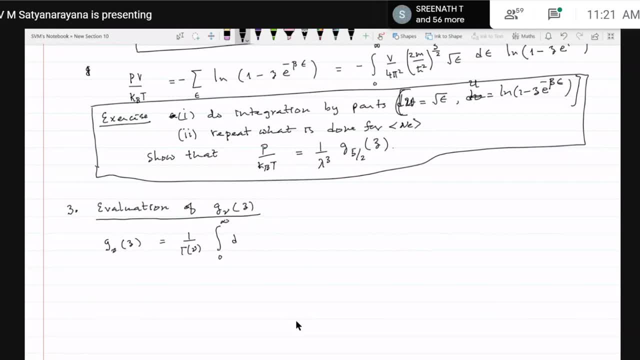 see that motherboard. you have any integration you do. you can see that it will integrate this first version. we started backwards and then we don't have chopper. you have hope this migrate integral 0 to infinity, dx, x to the power minus 1 into. so I will write this as: e to the power. 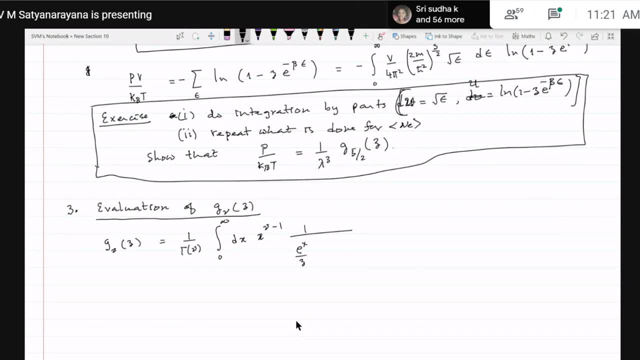 x divided by z, and that's what it is right. So I pull this out. that means e to the x by z. that becomes z into e to the minus x, right e to the minus x. So this can be written. 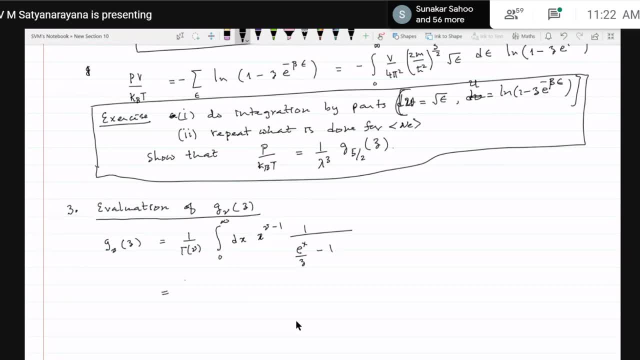 as I am actually doing some things which are not very difficult, but they are x to the minus 1 and I have z into e to the minus x into, I can write it as 1 minus z into e to the minus x, to the power minus 1.. So I pull out. 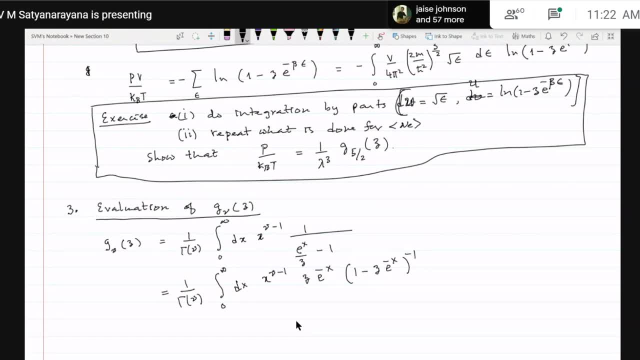 this factor. and then I have this. Now, this is something which I am going to write as e to the minus x. So I am going to write it as 1 minus z into e to the minus x, to the power minus 1.. So I pull out this. factor we have integral 0, I am going to write it as 0, I can write it as z to the minus x to the power minus 1.. That is one thing. you are going to see that this can be campoed with the help of case study. So let us try again, so to solve this problem. you are having to bring it to to the wall. So you have two consistencies of age. so let us use theseולםine podéis. So approximately you have the solutions for kg to the 오늘도 condition of extendable baseе, which you can expand in binomial series. 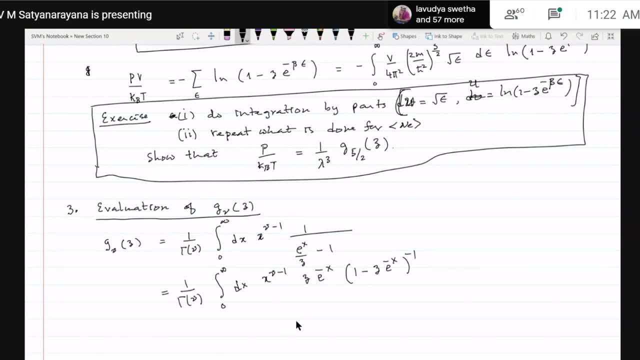 So you have an infinite series. So there are infinite series of integrals. Okay, so let us try to look at that one That is equal to 1 over gamma of mu, integral 0 to infinity, dxx to the meanwhile 1, and then you have plus 1 over, because some integration becomes. 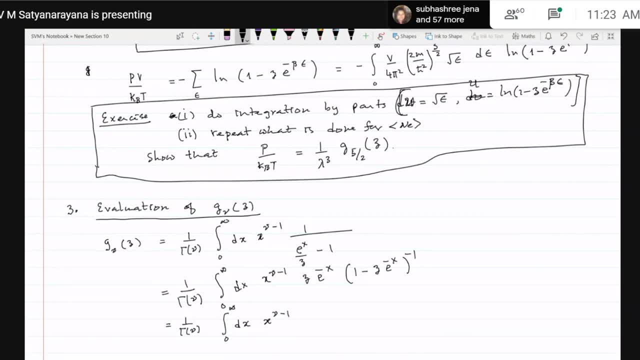 less significant. Then I have this: is like 1 plus x plus x, square, like that. so that is z into e to the minus x, plus z into e to the minus x to the square, plus z into e to the minus x cube, and so on. 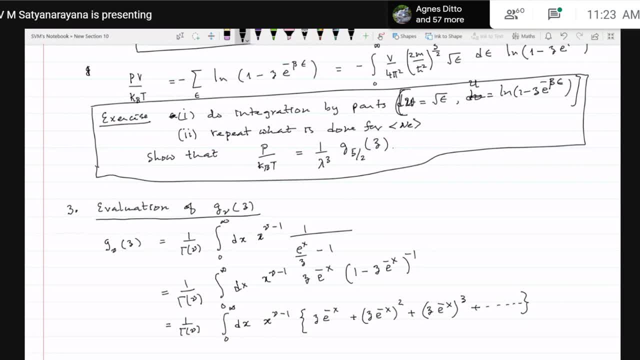 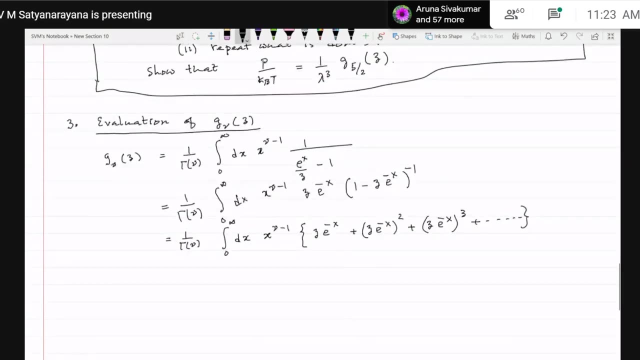 Now this is f of integral and planet integral. Now the integration is over, the integration is over x. so now I can pull that out and try to write this as: let me write it as: 1 over gamma of e into integral, 0 to infinity, e, x, x to the negative, e to the minus, x to 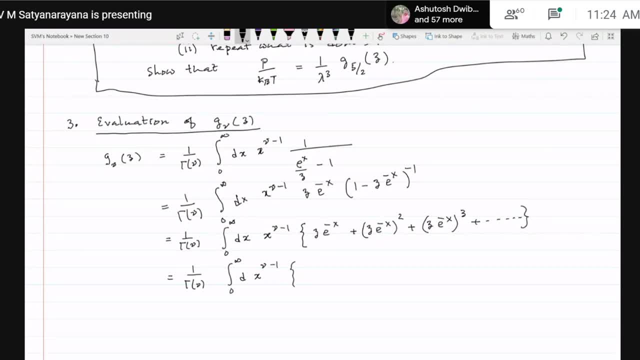 the n, the integral e to the minus x to the n to the minus x cube into integral x to the be minus 1.. And what I have in this bracket, I will write it as some: r is equal to 1 to infinity, z e to the minus x raised to the power. So that is what is there in the bracket. 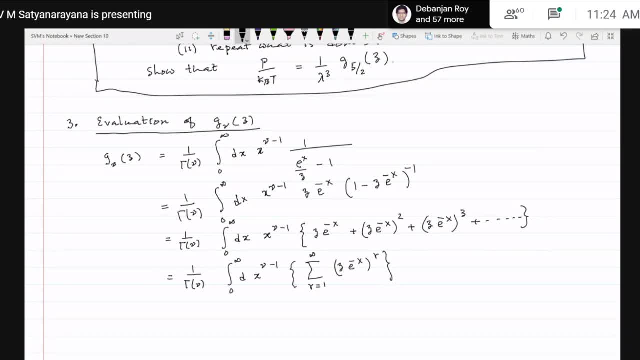 Now, since summation and integration are on two different indices, I can interchange them So I can write: sum over r is equal to 1 to infinity. Whatever is not depending on x, I will pull that out. That is, I have z to the power r and 1 by gamma of mu into integral 0 to. 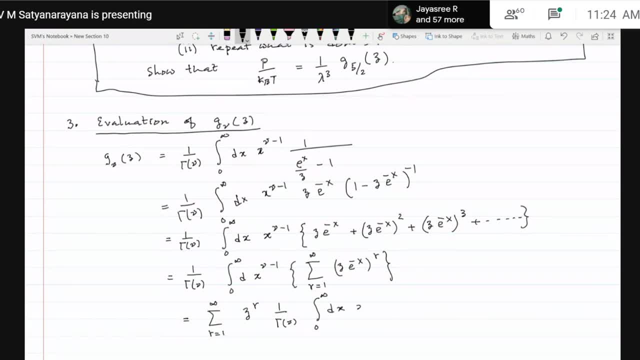 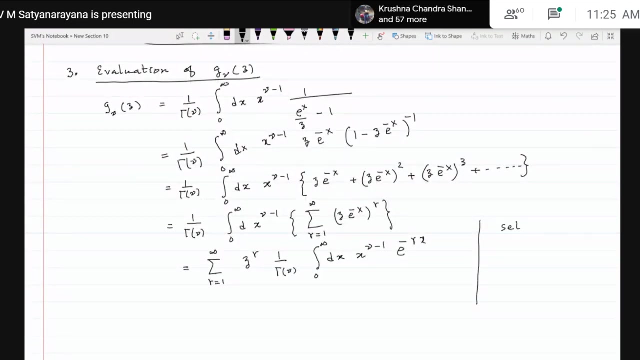 infinity dx, x to the mu minus 1 into e to the minus r x. This integration I have to perform And this integration is rather straightforward. So to do this integration, let us set r into x as some p, then x becomes p divided by r, and dx is equal to e to t by r. 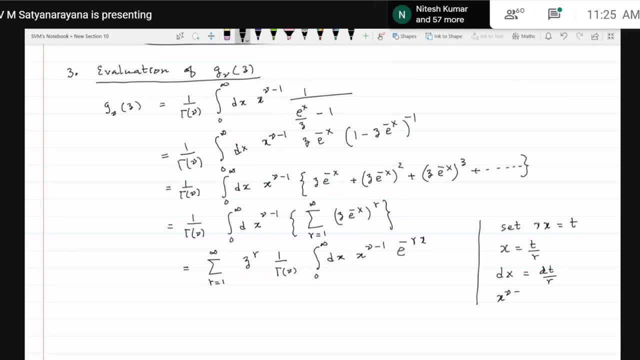 So x to the power mu minus 1 becomes t by r to the power mu minus 1.. So if I use all this substitution here, I have r is equal to 1 to infinity z to the power r, and you see I have r to the power mu coming out. 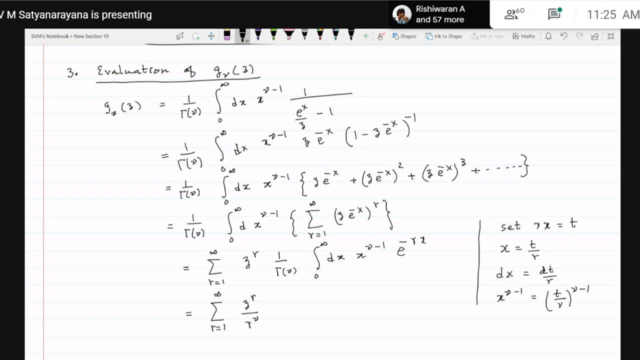 Because r to the power mu minus 1 from this term and 1 by r from this term, so that will become r to the power mu into 1 by gamma of mu, integral 0 to infinity limits. do not change. I have dt e to the mu minus 1, e to the minus 2.. 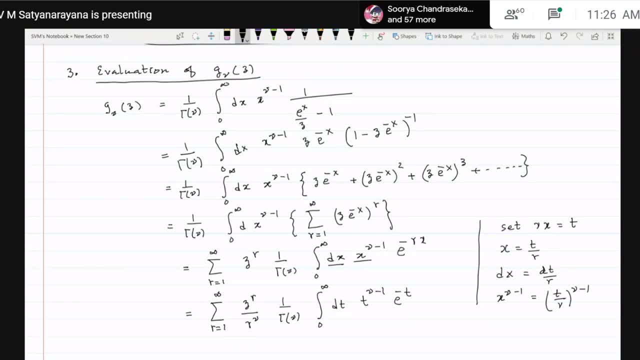 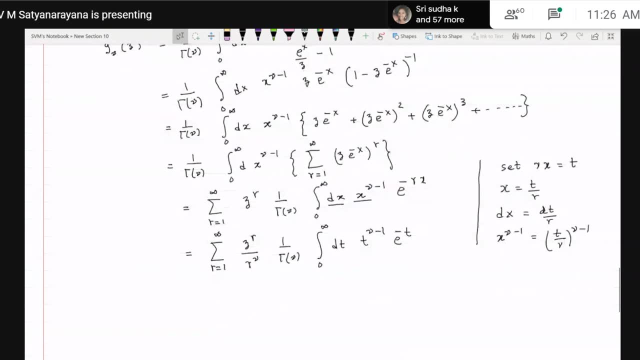 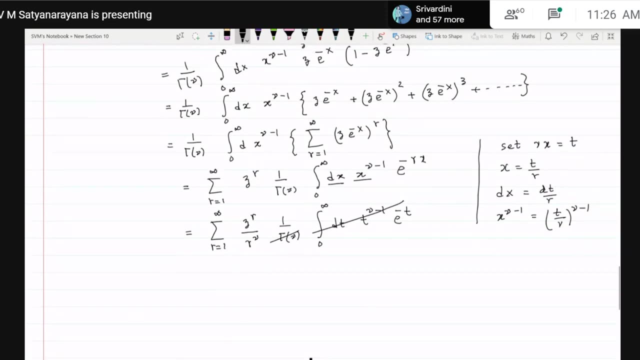 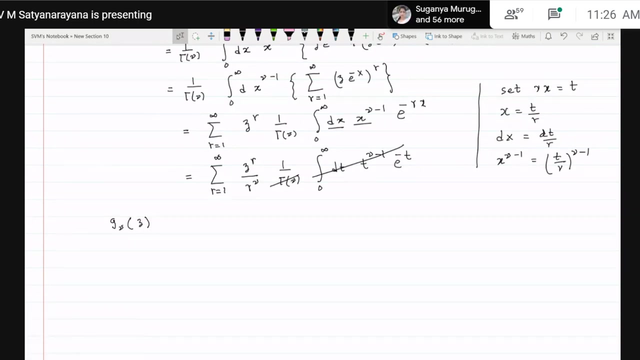 Now, if you know the definition of gamma function, this is gamma function. So whatever is this integral is gamma of mu. So you can see that this gamma of mu and this integral will cancel. So the Bose Einstein function I have now evaluated as g, mu of z, as. so that is so. 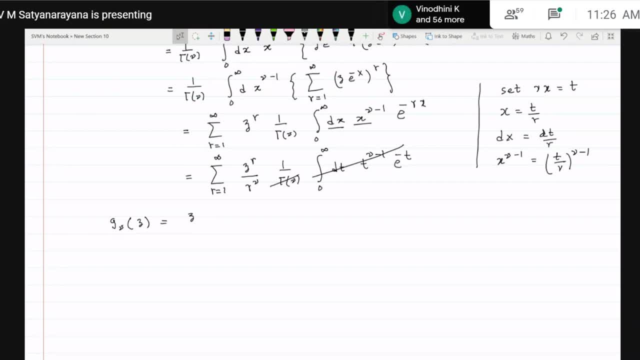 this is g mu of z plus g mu of z, square by 2 to the mu, plus g cube by 3 to the mu, and so on. There is an infinite series like this. So this is not a closed form expression, but then you can always evaluate to whatever. 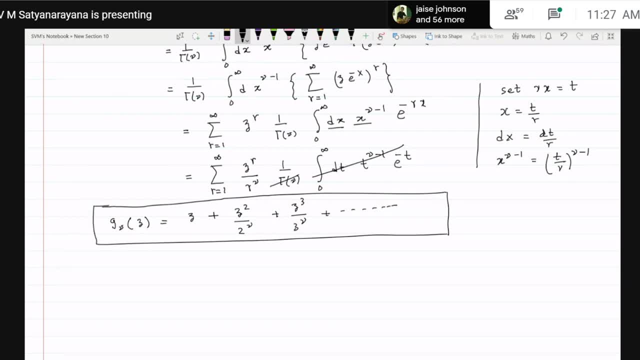 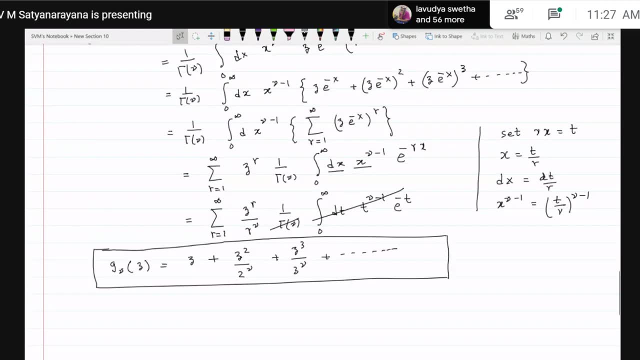 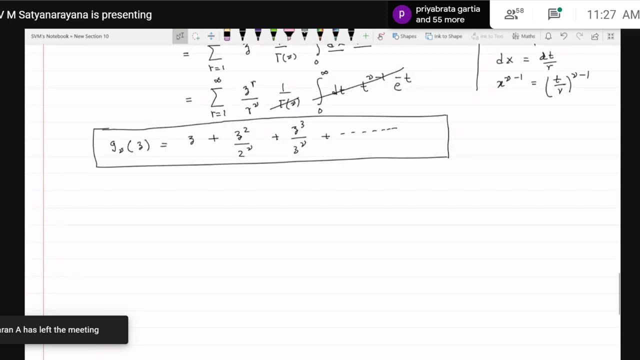 accuracy that you want. So I would consider this as reasonable evaluation of this, because we have at least obtained this as a function of, in terms of infinity. But then let us try to understand the nature of this function, So the nature of g, mu, of z. 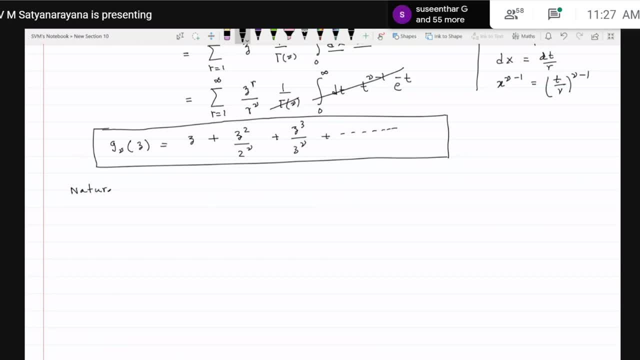 Now remember for bosons. for bosons, the highest value that mu can take is the ground state energy, and that is equal to 0. So mu actually is equal to 0. It is the highest value, Which means the highest value of z is plus 1.. 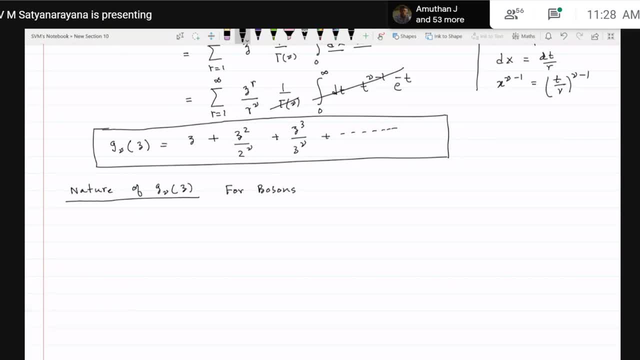 So for bosons, remember that 0 is less than or equal to, z is less than or equal to 1. Or equivalently. equivalently, we have minus infinity less than mu, less than or equal to mu. So that is the range of chemical potential, and 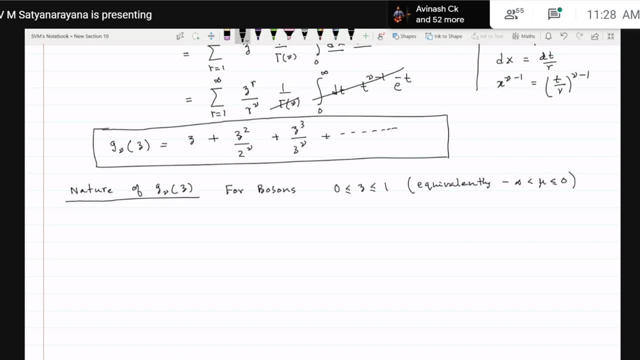 So that means in this range, you notice that…. So for 0, less than or equal to z, less than or equal to 1, notice that g, mu of z is a monotonically increasing öğ, Is the energy function. what does that mean? that means, if you have some, that line is greater. 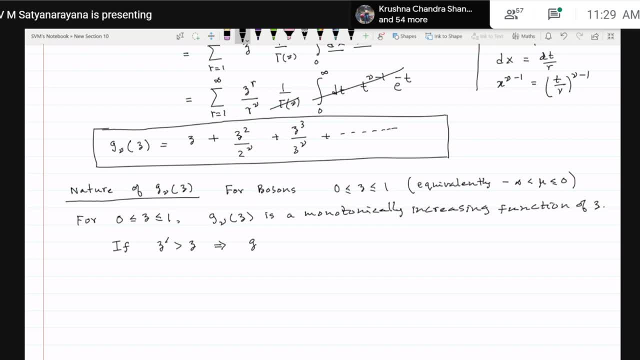 than z. that implies e mu of z prime is greater than e mu of z, and this is true for all, whatever is your mu, this is true. now, this is an important criteria, or this is an important property of this g mu of z, which you can notice. of course, this is true if you have a g mu of. 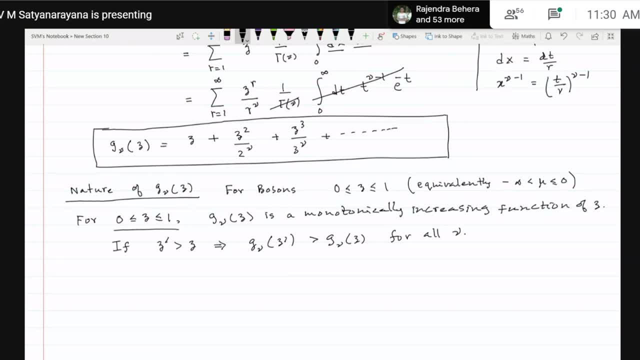 z is positive, and for our situation z is. if it is not positive, then all r terms will become a negative sign, and then this monotonically increasing condition will not be satisfied. but since here the fugacity is a positive quantity, this g mu of z is the monotonically 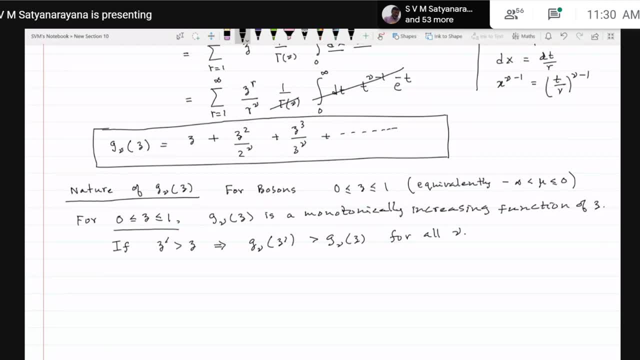 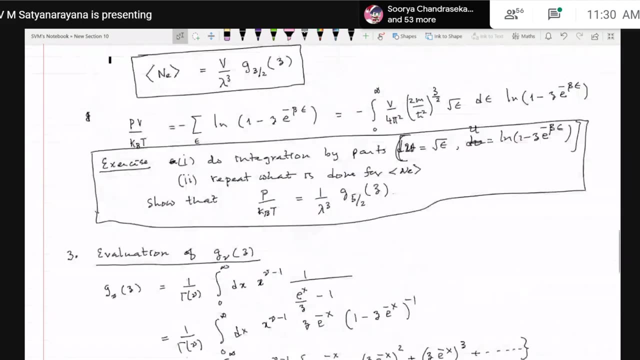 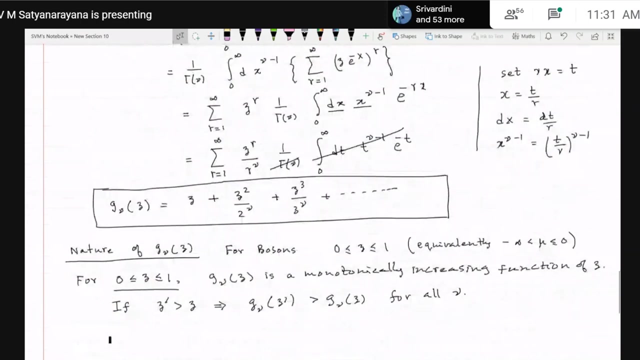 an increasing function of z. okay, so, so far, so good. so we have the nature of this g mu of z. so once we have this, then we go back to our problem, where we have obtained an expression for the average number of particles occupying all the excited states in terms of one of. 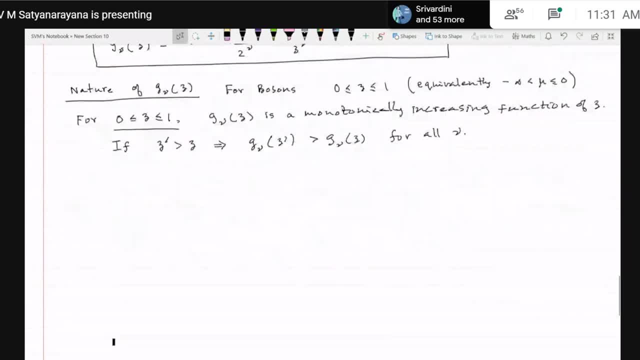 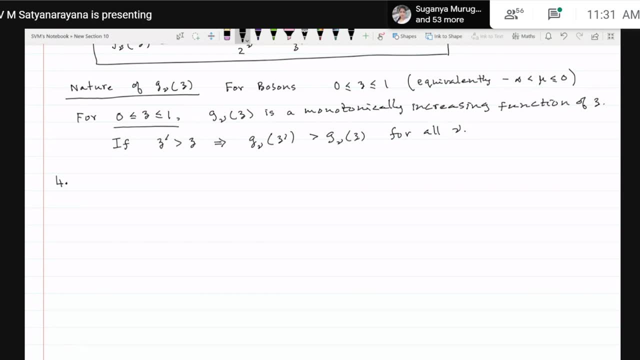 these functions. so let us look at the analysis. now let us take a look at the analysis of the g, mu of z. okay, So we have. we have: average number of particles is equal to v divided by lambda 2 into p. p by 2 half. 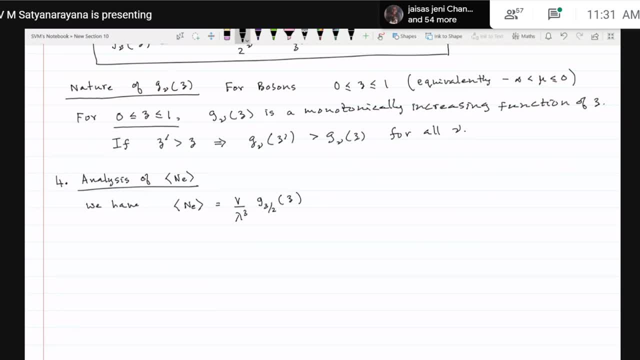 So this is the g? mu of z. So this is the g? mu of z Now. so here, here is where an important physical result, that that we will be showing to please pay attention. So now, what I am trying to say is that so, maximum value of z. okay, so maximum value of. 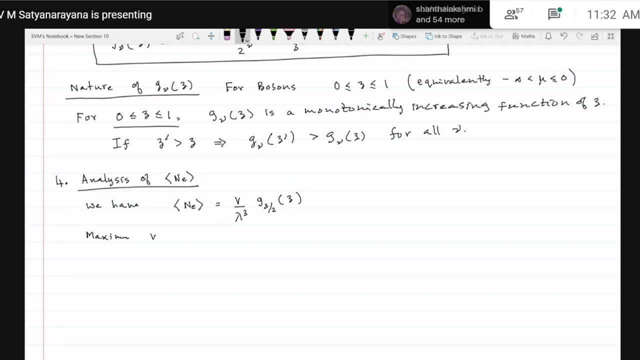 z is that is equal to 1.. That means we can say that g 3 by 2 of z is less than g 3 by 2 of 1.. Why? Because this is a monotonically increasing function. Maximum value of z is 1, so g 3 by 2 of z is less than g 3 by 2 of 1. correct this much. 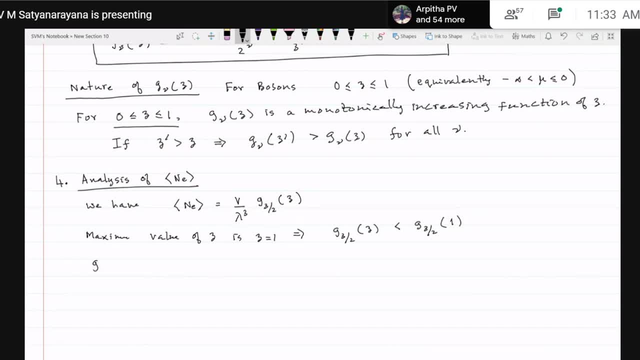 is clear. So what is g 3 by 2 of 1? g 3 by 2 of 1 is- we have already evaluated that that is equal to 1 plus 1 by 2, to the power 3 by 2.. 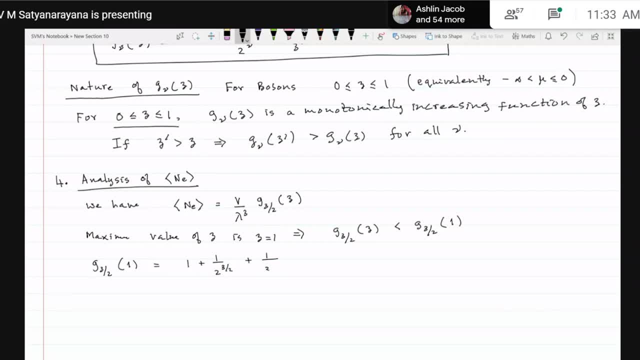 Okay, So g 3 by 2 of 1 plus 1 by 2 to the power 3 by 2 plus 1 by 4 to the power 3 by 2 and 4.. So this is what is called. sum over a is equal to 1 to infinity. 1 by a to the power 3 by. 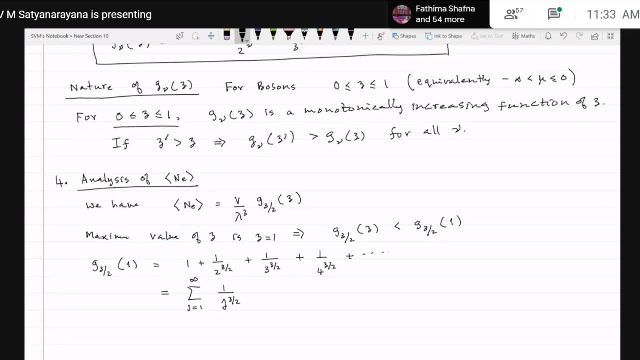 2. And you should provide a였, as anytime, So I we should give a each shines attached to the power. 3 by 2 plus one, plus one to the four. Well then, what is the g? 3 by 2?. 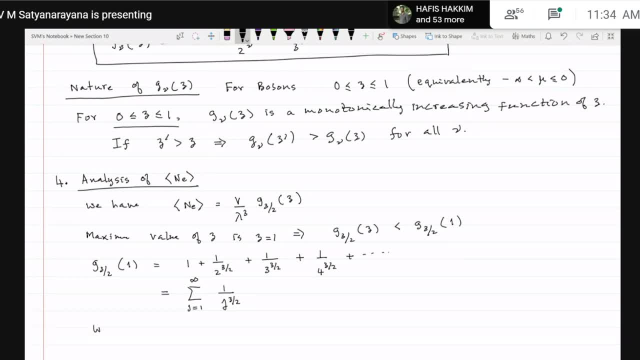 So g 3 by 2 of 1 plus 0 to the power 0.. So what are g 3 of 1? g 3 of 1 plus 1 plus g t is equal to g 3 of 2 plus 1 plus 425 of g and mH will be equal. 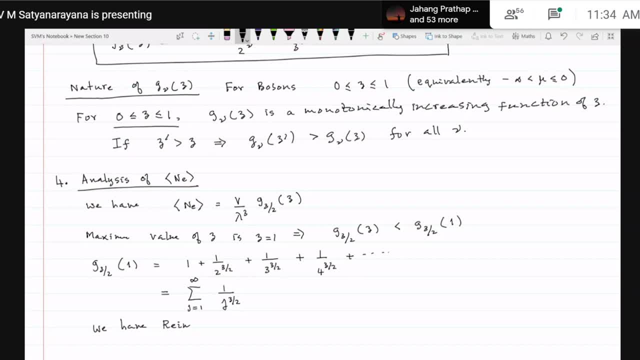 to 1hington, it is equal to 0.. Why Look this? Thanks, Great zeta is. zeta looks like this. So zeta of alpha is defined as: sum over j is equal to 1 to infinity, 1 by j to the power alpha. This is called Riemann Zeta. function Now essentially: 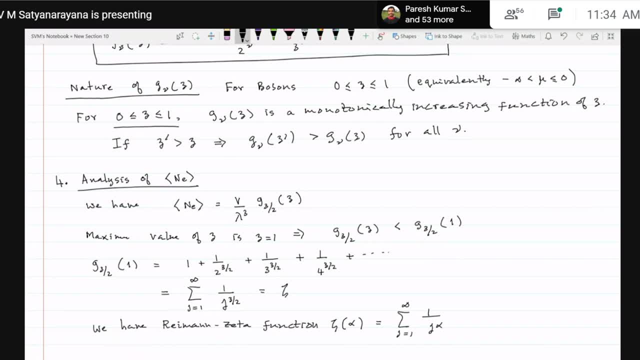 what is this one? This is basically a Riemann Zeta function of argument 3 by 2.. And this infinite series will converge. So we know that this Riemann Zeta function of 3 by 2 will converge to a value of 2.612. 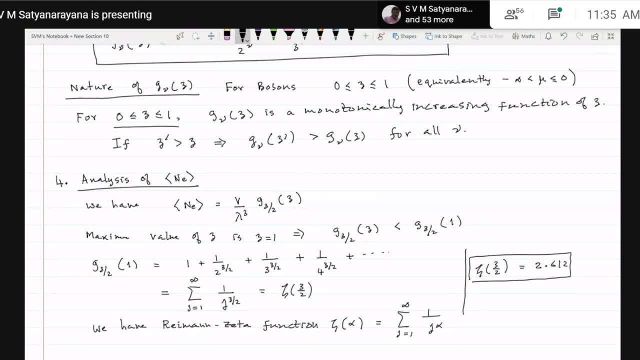 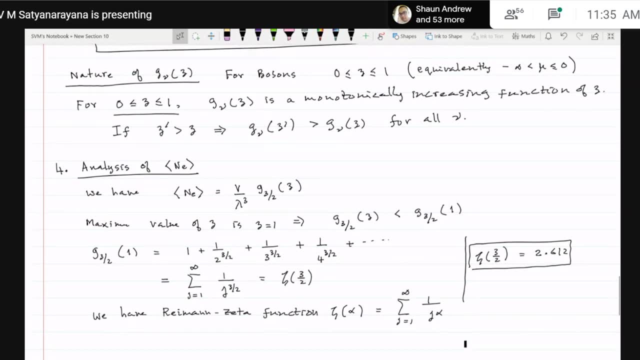 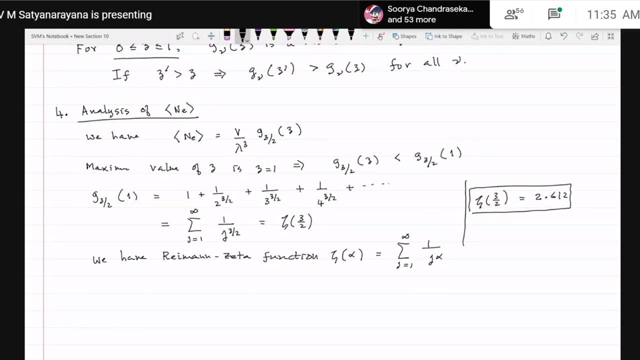 Yes, this will converge the value like this, So that that? what does that mean? That means that whatever is your, whatever is your z, the average number of particles that occupy all the excited states cannot exceed, which will be less than or equal to. 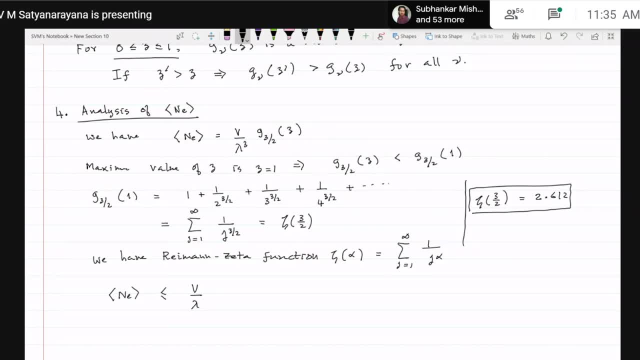 V is a positive, its not. So that is it. You can see the zero or the non-zero, and the positive Now we will becomes couldnot exceed to value. So love the value Now I am generating certain by lambda cube into zeta of theta. So whatever is there on the right hand side here this: 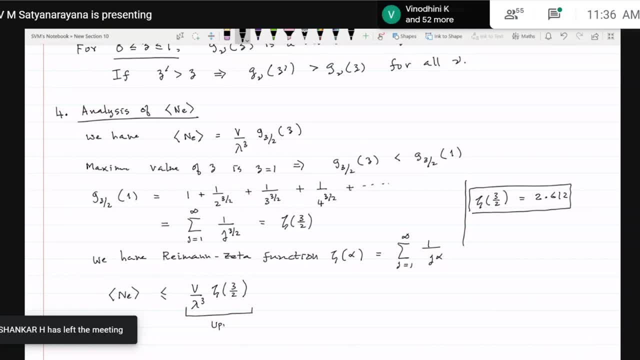 serves as an upper bound, an upper bound on the average number of particles of bosons, all excited states which apparently are, which are in finite limit. So this is kind of intriguing result: of bosons There are infinitely many states, but they cannot hold infinitely many particles There. 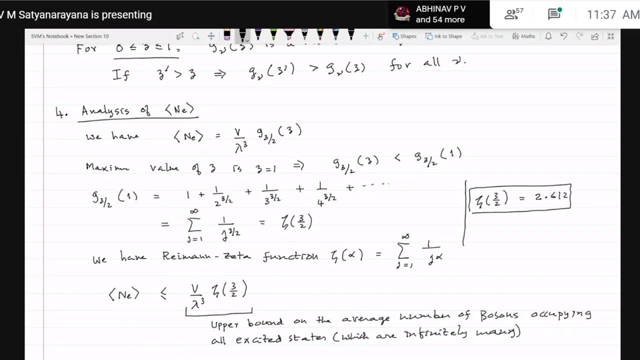 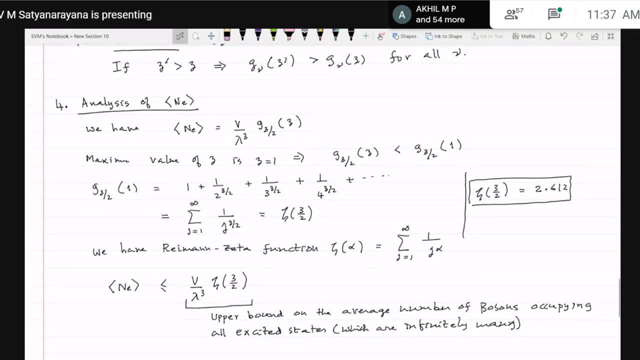 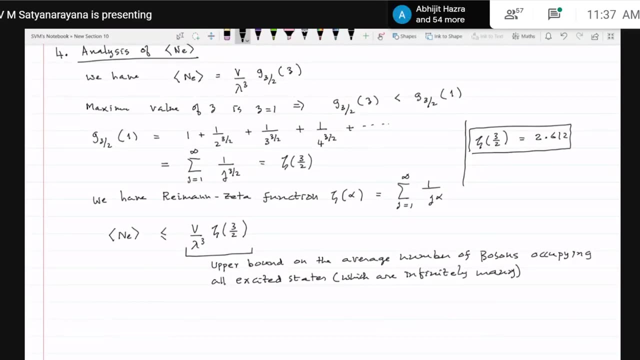 is kind of a upper bound on the average number of particles that all the excited states together can hold. Okay, so I do not know if you find it very intriguing, but this is something which is what the cases are the nature of. So now we can think of, let me, let us say that I have, so let us say that I am so imagine. 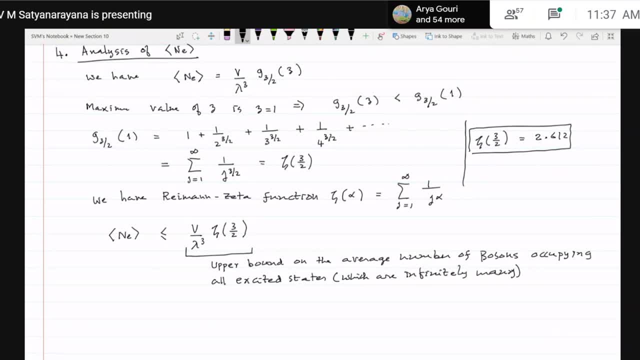 that you are doing an experiment like this. Okay, so let us discuss the test case one, Okay. Okay, let us say we have n particles, Yes, So there are n bosons, such that n is less than this value. e to the lambda cube into. 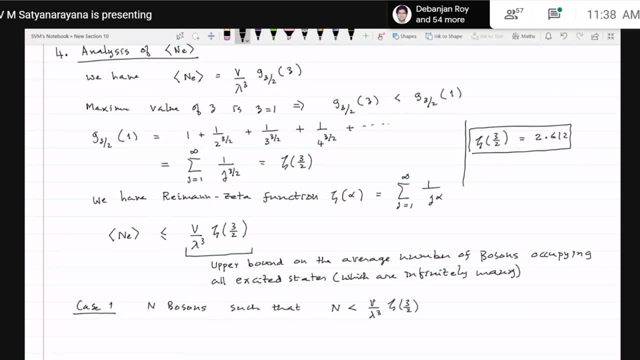 zeta of e to the lambda. Then what happens? Nothing much happens. So all states have some occupancy consistent with what we have discussed so far. But what happens? imagine what happens. What happens If you go on increasing your n, if you add more and more particles or bosons to the system? 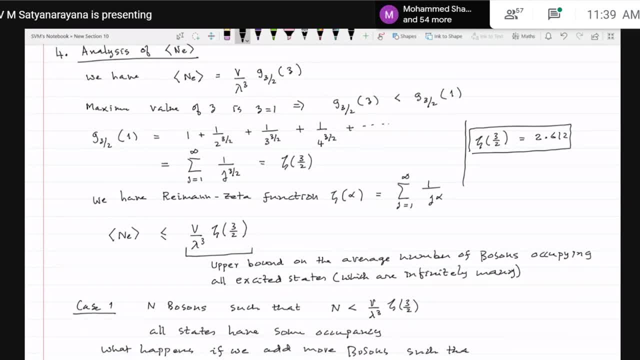 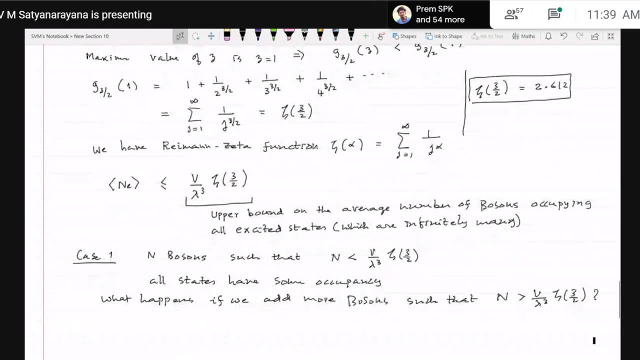 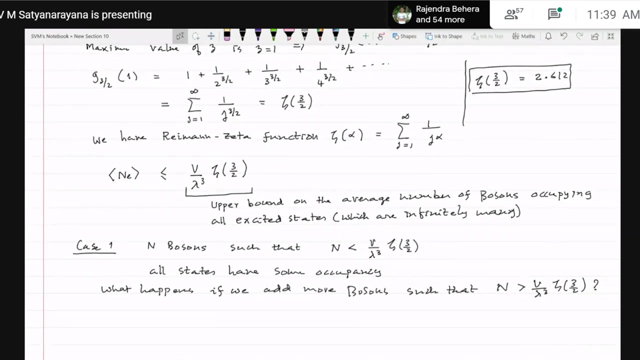 such that now this n becomes larger than e by lambda cube into zeta of e to the lambda. What happens? The extra particles that we are adding? they cannot be accommodated in the excited states because excited state occupancy has an upper bound. So what will happen? that all these particles? so that means so this n minus e by lambda. 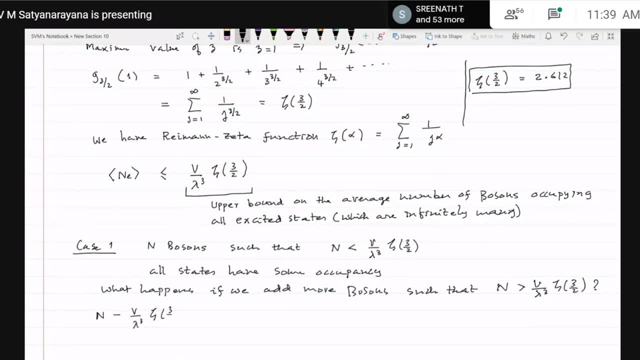 cube into zeta of e to the lambda. Okay, This is r 3 by 2.. Okay, So these many particles, they go to ground state And there is no limit on the ground state, occupancy, ground state. That means ground state. as many of them, how many over the particles one take and 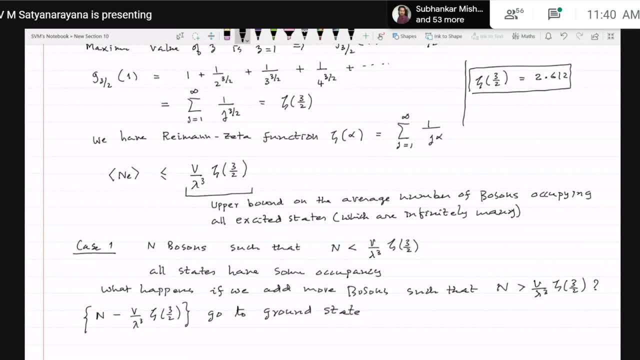 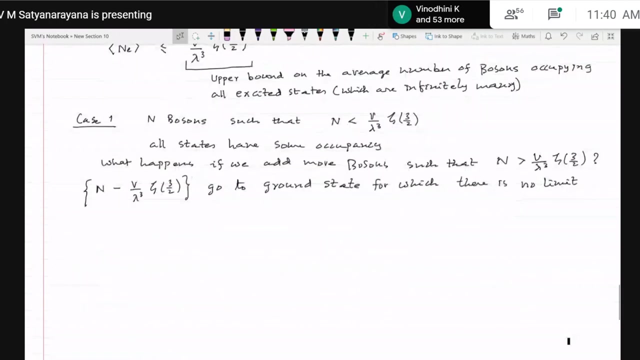 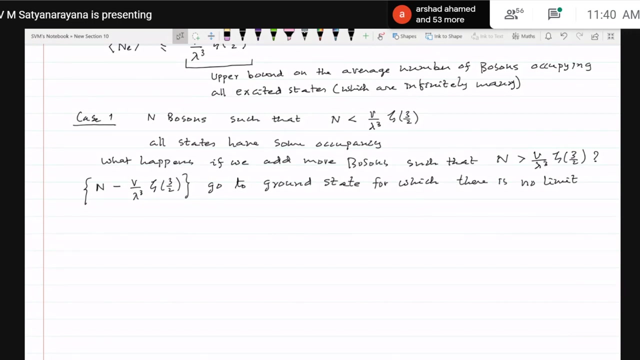 go to ground state. There is an upper limit only on the excited states. go to ground state for which there is no limit. there is only one state, but you can have any number of particles, so there is a macroscopic occupation of the ground state. that is possible when your number of 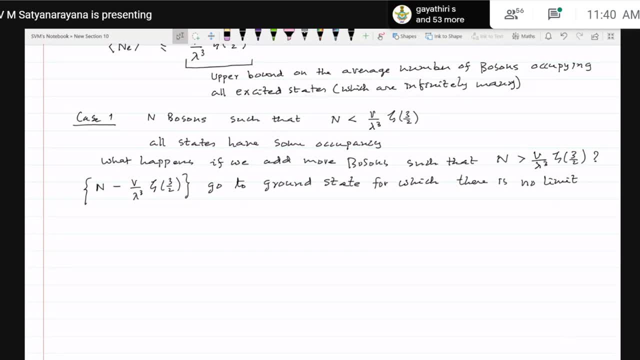 particles is larger than the upper limit. upper limit is what we have derived as v by lambda 2 into zeta of t beta. this is a. this is one case. we could also see it in a different way, that is, let's say, let's look at case. 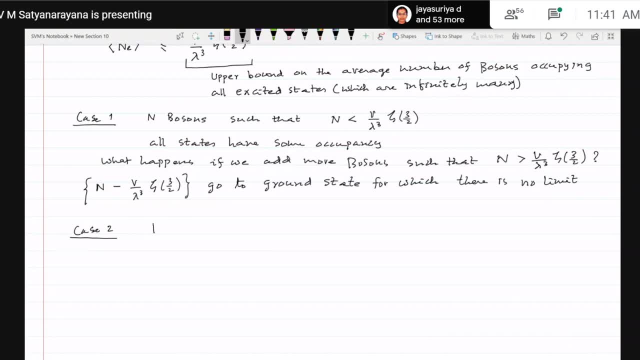 two. so in this case, let us try to fix our number of particles, fix n and fix v. okay, let's fix n and v, okay. so maybe it is such that, so such that that n is less than v by lambda q to theta. okay, now notice that. 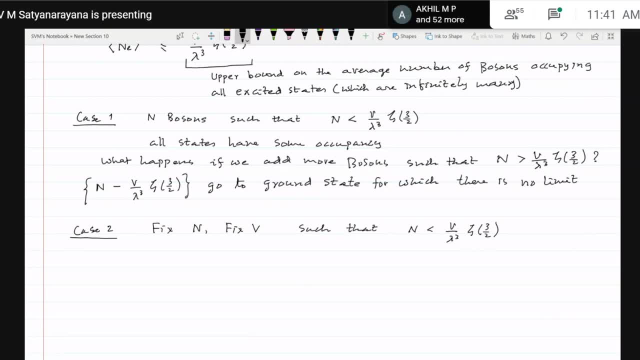 so now there is no problem there. that means all of them are occupied. all the states are occupied. this is like normal application. now notice that this, notice that that the upper bound, upper bound, is a function of temperature, is a function of temperature. where is the temperature? the temperature is there in this lambda q. 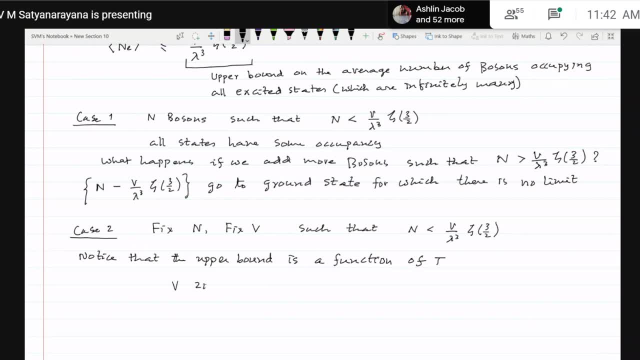 that is, you have v into 2, pi, m, a, b, t by h bar square, h square to the power, 3 by 2 into zeta of 3 by 2. so this is a temperature dependence comes from here. now, uh, for a given number of particles, the upper bound of the ground state is: 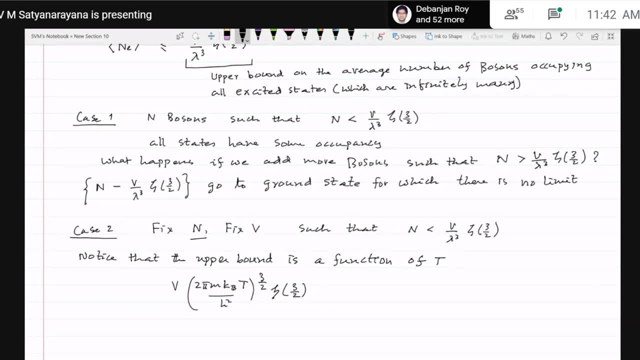 is such that the number of particles is less than that upper bound, but i can make this upper one smaller by reducing the temperature, okay, so the upper bound, upper bound, uh, upper bound, on average number of excited state of particles can be reduced by increasing- sorry, by decreasing. 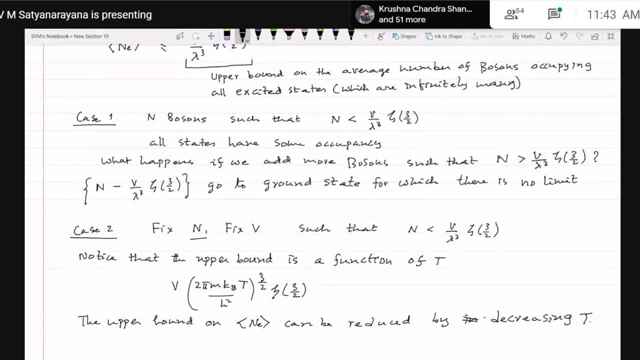 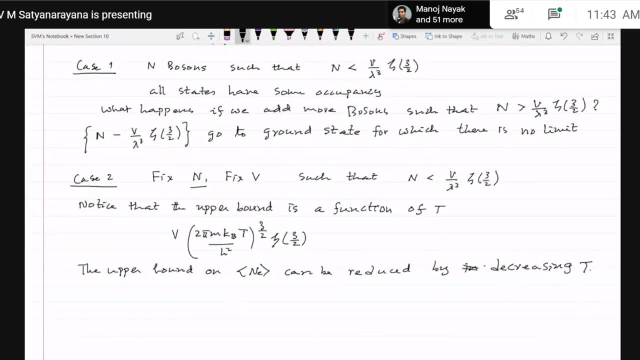 by decreasing temperature. so what happens is that if you go on decreasing the temperature, so there exists a temperature, okay, for which this n is equal to this, okay, so i am going on decreasing this. so For some temperature, which I will call it as E c, we have n. the number of particles. 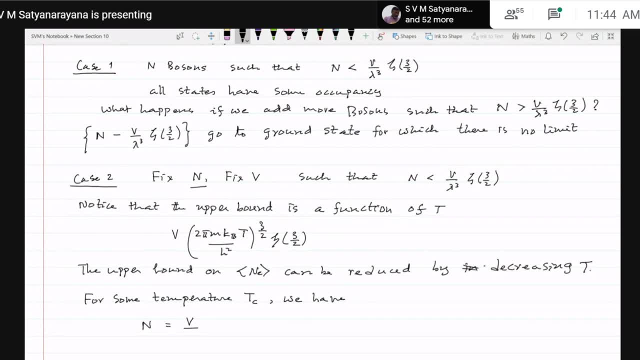 is equal to v divided by so v. let me write it like this: v times 2, pi, m, A, b, E, c divided by h, square to the power 3 by 2 into beta of theta. Okay, so we can revert this relation and then write an expression for: 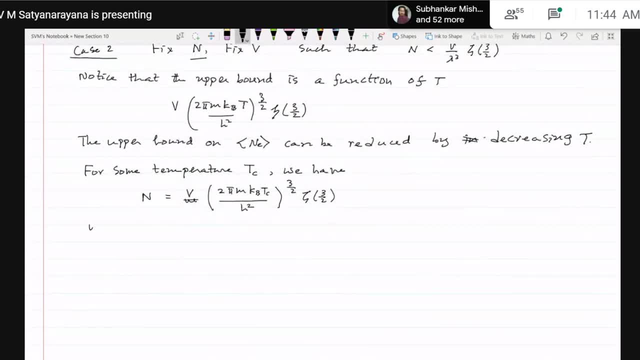 we can write this: T c is equal to h bar h square divided by 2, pi m k B into n divided by p, into zeta of 3 by 2.. Okay, Okay, We can write: the temperature at which exactly this upper bound is equal to the number of. 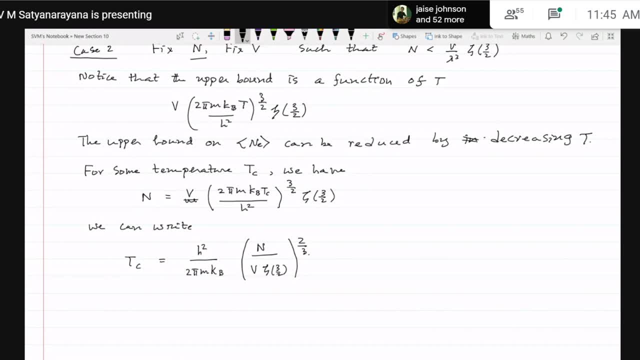 particles. Okay, Okay, Then it is easy to understand. It is now easy to see: For T less than T c, that means you are further decreasing the temperature beyond this. then what happens? the number of particles will be much more than the upper bound. 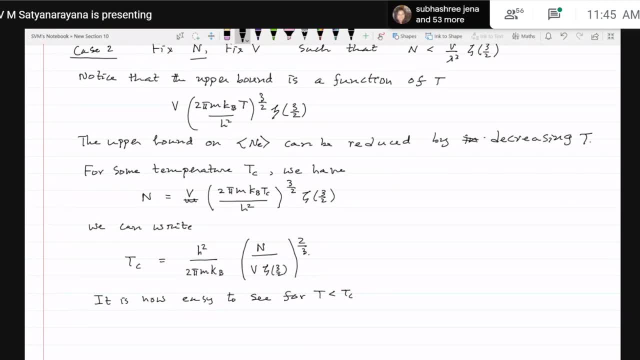 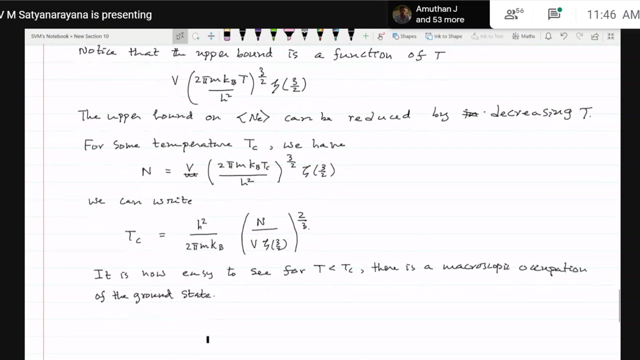 So all those additional particles have to now jump to ground state. See that for T less than T c there is, there is a macroscopic occupation. Okay, A macroscopic occupation, occupation of the ground state, Okay. So this phenomenon is what we call as Bose. Einstein, Condensation is what is called Bose. 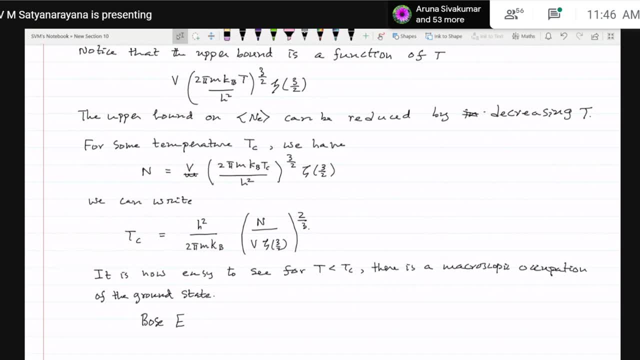 Сondensation, Condensation, Condensation, Condensation, Condensation, Condensation, Condensation. So this is a kind of phase transition from ideal Bose gas. so this is the phase transition From ideal Bose gas to Bose Einstein formula. so BEC is one of the very interesting state. 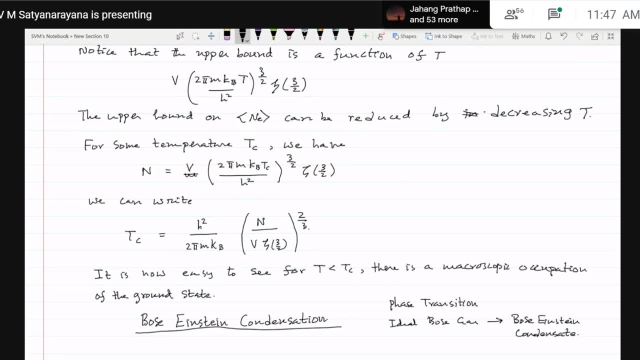 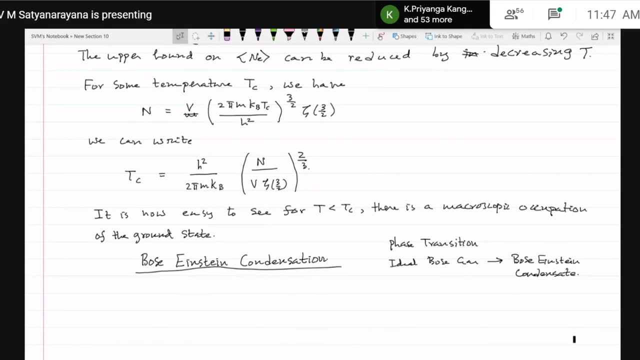 of matter, And there is lot of, even though Einstein had predicted this in 1925 and 1924, but it has been experimentally. Bose-Einstein condensation was experimentally observed in mid-90s, 95 or so. 2001 Nobel Prize was given for people who experimentally observed. 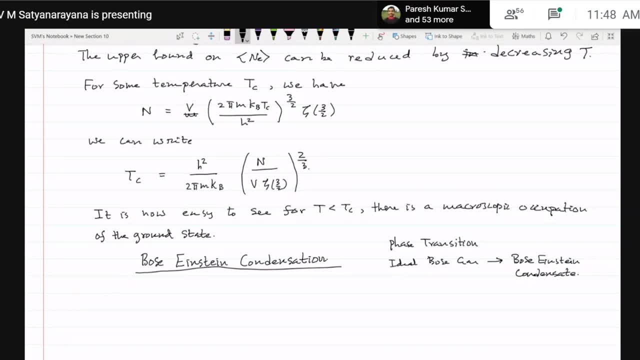 Bose-Einstein condensation at very, very low temperatures. for example, for ideal Bose gas the Tc is of the order of nano Kelvin temperature. That means it is something like 10 to the minus 9 Kelvin temperature. At such temperatures you will see that the ideal Bose gas will become Bose-Einstein. 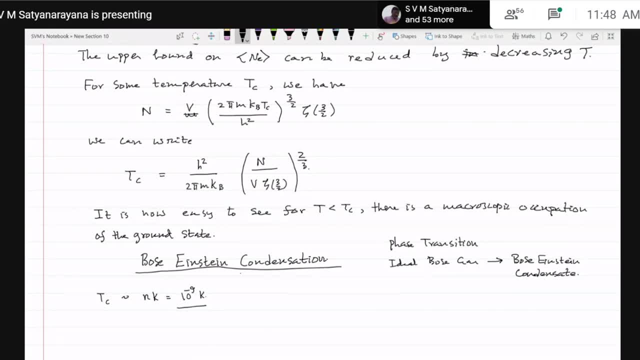 Now, even though this word condensation is useful, We have to understand there are important differences. It is not like gas condensing to liquid, Because gas condensing to liquid, that is gas condensing to liquid. This happens in real space. And second thing is that 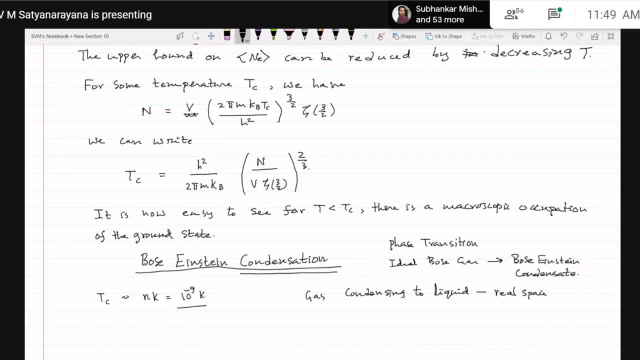 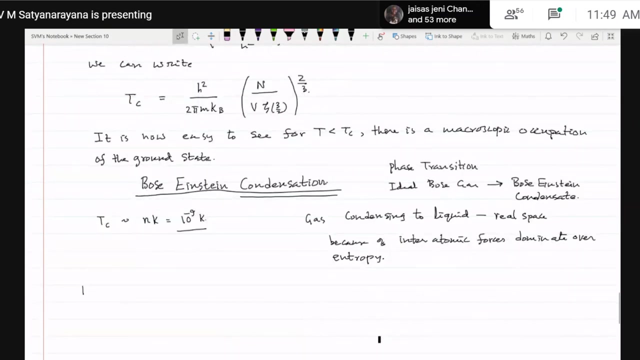 This happens because. so, this happens because of intermolecular forces or interatomic intermolecular forces, forces dominate over thermal disorder or over entropy. Okay Now, Bose-Einstein condensation is very unique type of an example where this BEC BEC happens. 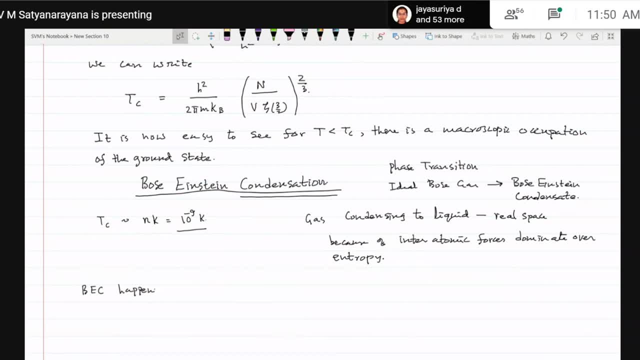 happens, or what is called the origin of this BEC, This quantum mechanically, completely quantum mechanically. Essentially, that means that due to, due to wave function, there are no interactions. So this is essentially because of the. So this is essentially because of the. 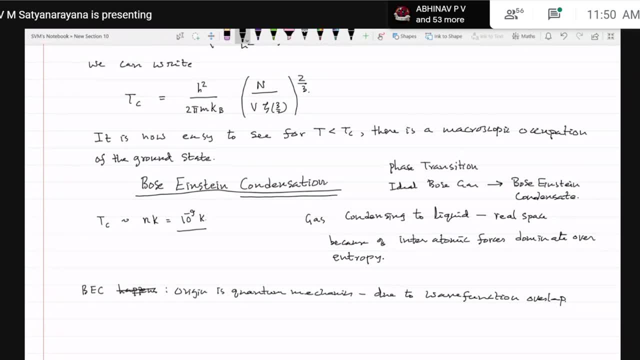 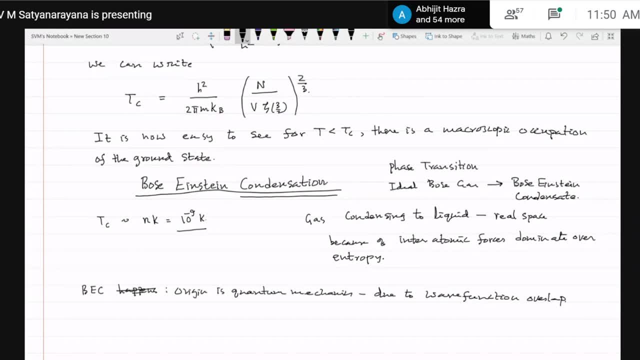 There are no interactions And the condensation condensation is not in the real space, but it is in the momentum space. Okay, what does that mean? that means these are free particles, so your epsilon is equal to H bar square, K square by 2m. these are free particle energies, so epsilon is: 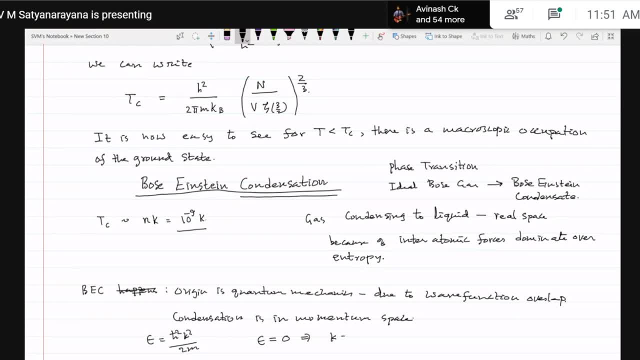 equal to zero. this implies K is equal to zero. so if you imagine that you have, you have a lot of these energy levels like this and each one of them are also having a particular value of momentum because it's a free particle. so maybe this particle is here. this particle is here. this particle is here, some other? 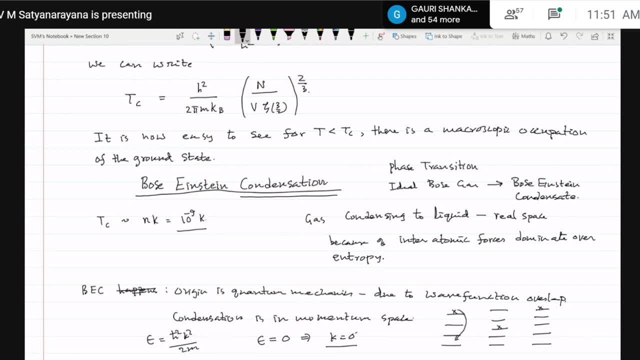 particles somewhere and what happens is that all of them will come to down state at P less than Tc. So this kind of a G gerund module will give you a Greening疫이라고. numbers is even less than now staid y. 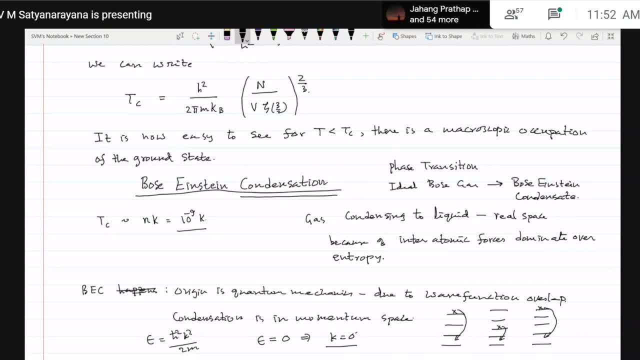 p less than pc. jumping is not that like. if you have a gas filling the entire chamber and it becomes liquid, then it will settle on to the bottom of the chamber, right, that is how gas liquid condensation takes place, or it will be settling on to the walls of the. 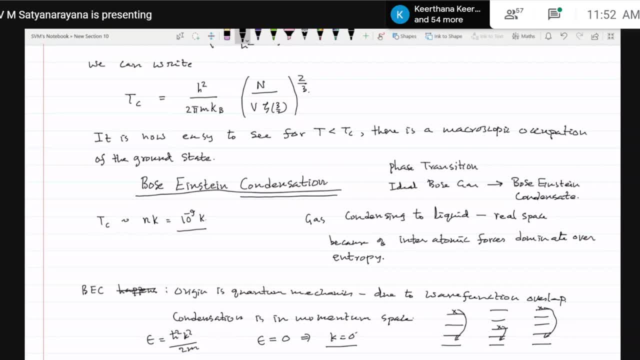 container. so, like that, there is no physical space condensation. wherever particles are there, they will be there, but they will simply stop moving, or simply they just be. their momentum becomes zero. so this is what is called the condensation in the momentum space. so that is what is the difference between. 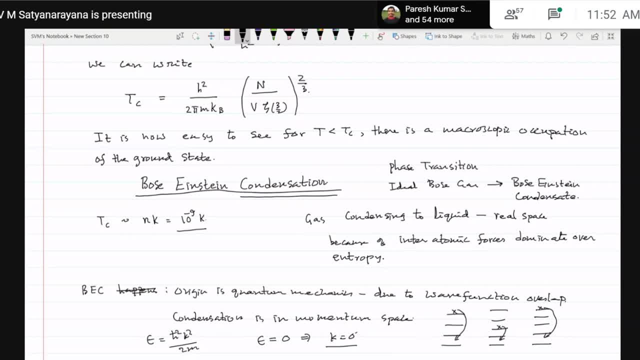 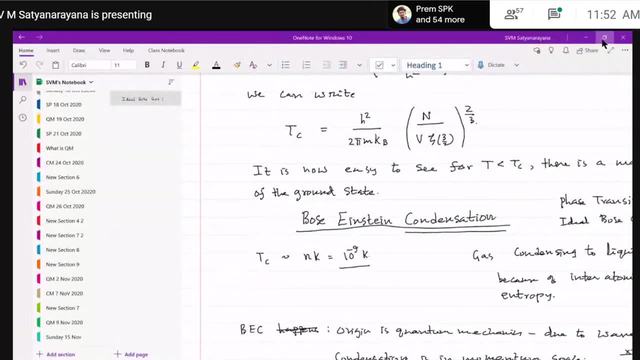 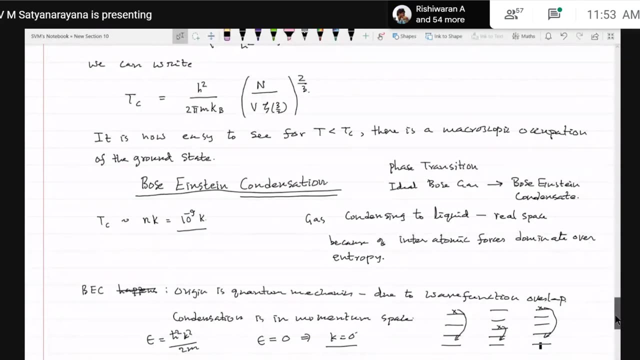 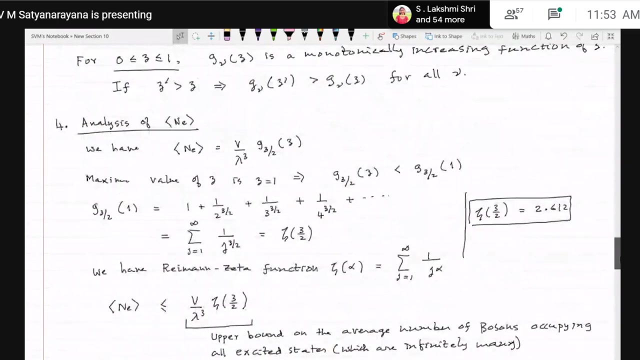 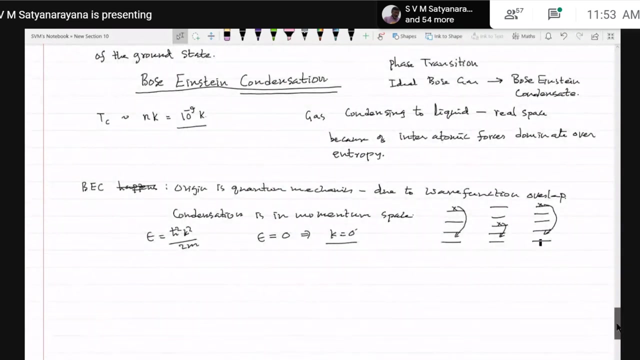 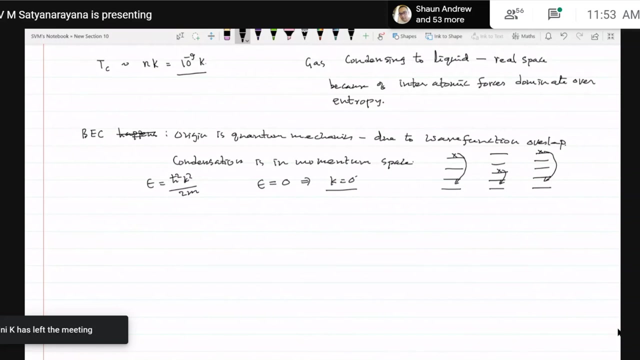 this Bose-Einstein condensation and other phase condensation that we are familiar with. so this is the nature of this transition and you can see that you can ask, we can ask a question- whether this Bose-Einstein Condensation is yeah, so we can ask some simple questions like this. 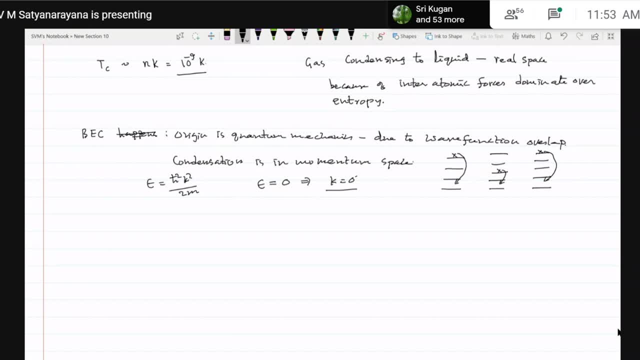 Like, for example, if you, as I told you, that, if you consider this density of states for the other dimensions, like I told you that I did not ask you to do it but let me write, it is equal to some c times d- I mean cd- some constant twice n by n power square to. 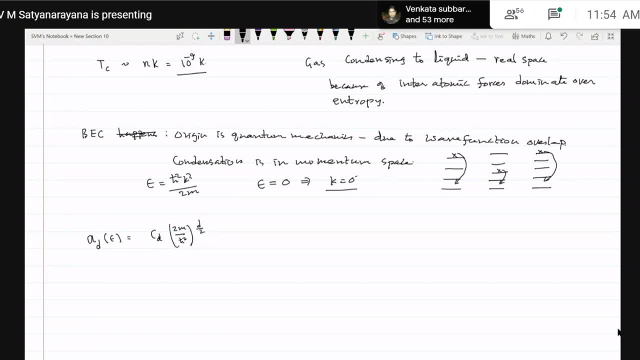 the d by 2.. So I am talking about d we see in other dimensions. okay, in other dimensions. So then we have epsilon to the power d minus 2.. Okay, so now let us look at two dimension. 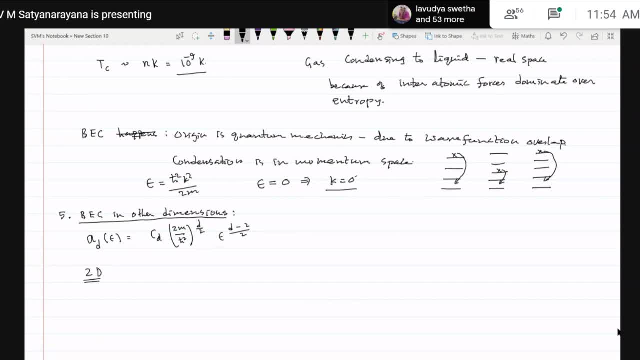 let us look at d. So I just want to say that it is two dimension. this is independent of this proportion of epsilon. ok, So I want to argue in a. so your m e average value of m e. okay, so I will not write all. 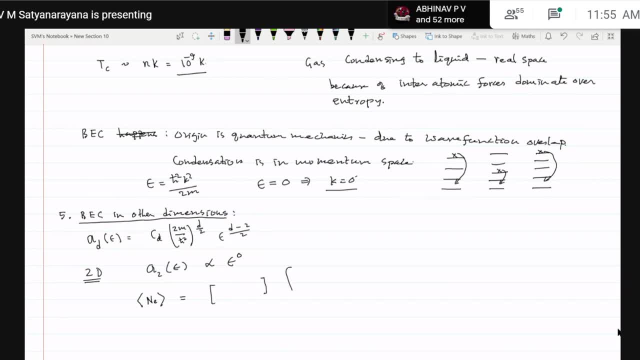 these constants, but it will be something like 0 to infinity. I do not have epsilon, because epsilon to the power 0, so but I can write this as epsilon to the power 1 minus 1 and z inverse e to the beta epsilon minus 1, so you can see that this n of e in this. 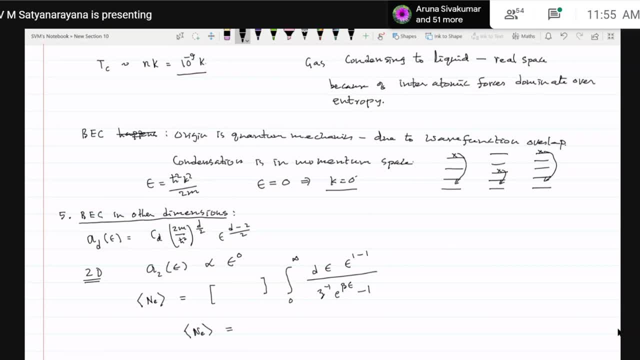 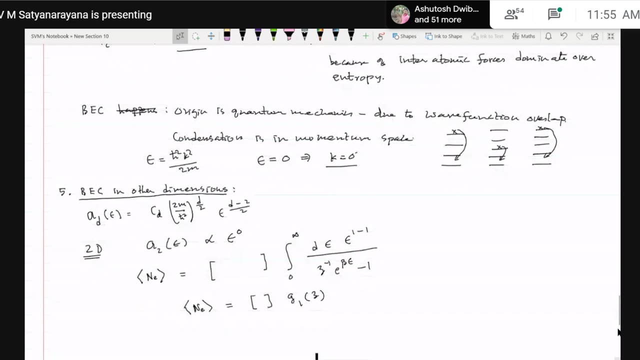 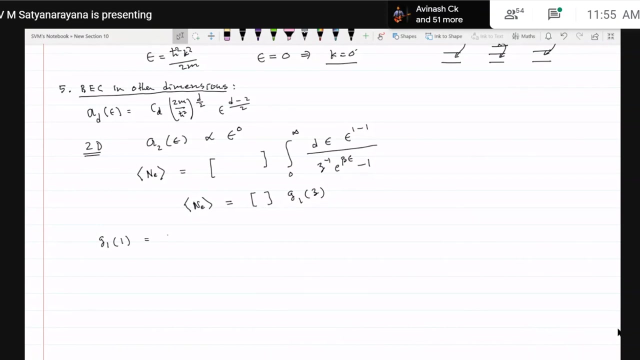 case can be written as some constant into g 1 of z. Now g 1 of z is g 1 of 1. is equal to 1 plus 1 by 2 plus 1 by 3 plus 1 by 4.. Now this: 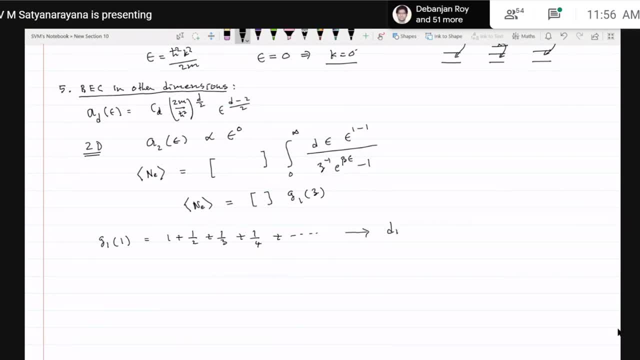 series is divergent. series Diverges to, however, very slow divergence, but this is nevertheless divergent. So we have, in fact, this is the famous logarithmic divergence- diverges to infinity. So there exists no value to which this converges. okay, unlike. unlike the case of g. 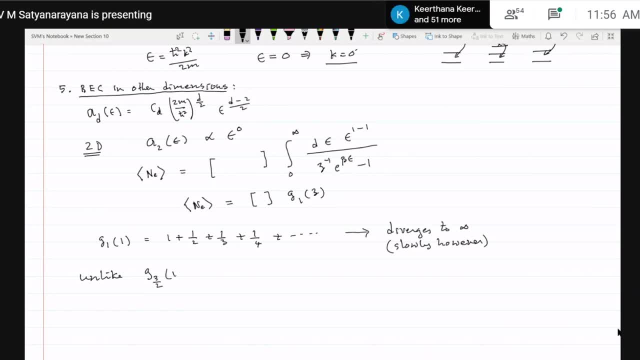 Now this converges to 2 point whatever, or this converges to a value. So this divergence, this divergence means there is no, there is no upper limit. there is no upper limit on n. That simply implies that there is no, no b in 2 dimension. Now you can also argue: the 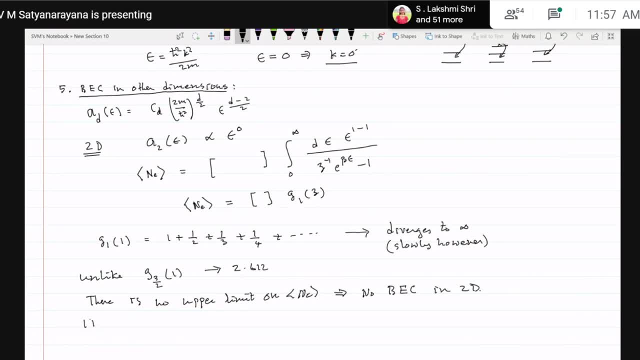 same thing with 1 dimension, because if you take 1 b, your a 1 of epsilon will be will be proportional to h times the power minus 1.. Okay, So this simply implies that your average n? e is actually equal to some constant into. 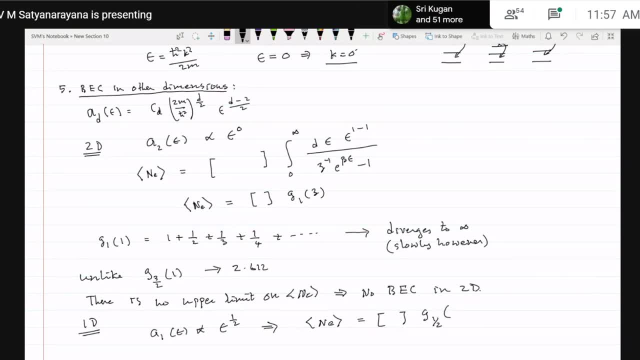 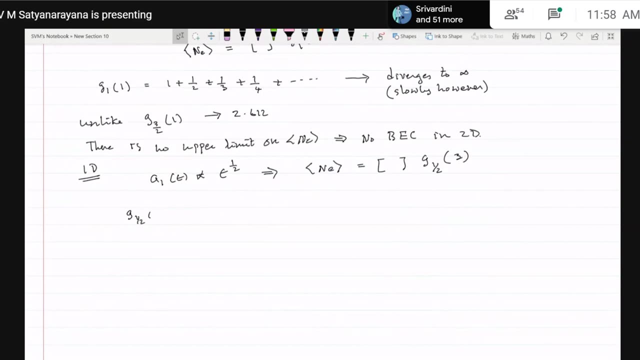 g to the power half into g to the power half of z. So this also diverges. this definitely diverges much faster than the logarithmic divergence, because g half of 1 is 1 plus 1 by 2.. Okay, 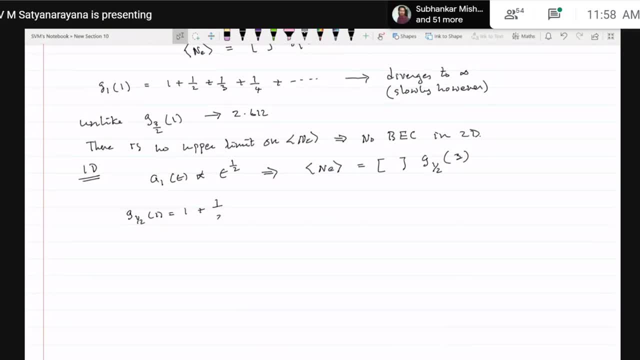 So this simply implies that your average n e is actually equal to some constant into 1 plus 1 by 2 to the power half of z, plus 1 by 3 to the power half of z, plus 1 by 3 to the power half of z. 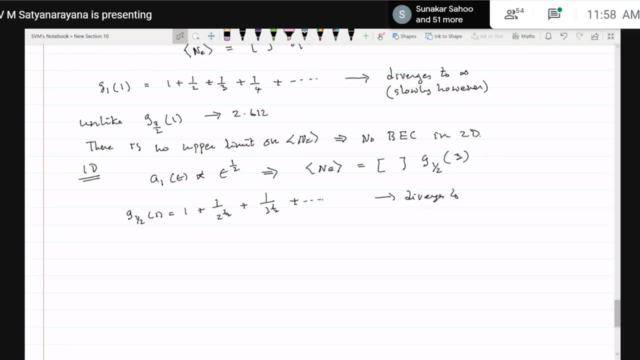 Okay, But it diverges In fact in here gives something such as minus 1 over new r, equal to 1 by a over s by 1.. I will, Let me see here. Let us see this once again. Here is what we have in. 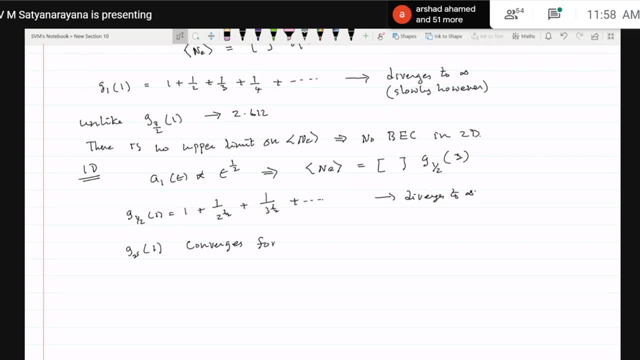 Let us see what this produces. This is a very, very complex dissertation. mu greater than 1 and diverges for mu less than or equal to 1.. So because of this, there is no cosine function conversation involved And it is easy to understand that if you have some these dimensions I am just discussing. 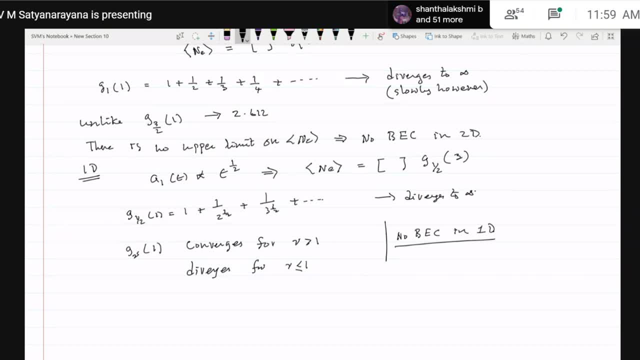 because these dimensions are, one can experimentally check. but you know, if you have 4 dimensions, 5 dimensions, you know boson, constant communication is possible because there is an upper limit, because those for mu greater than 1, they will all converge and hence there is a possibility. 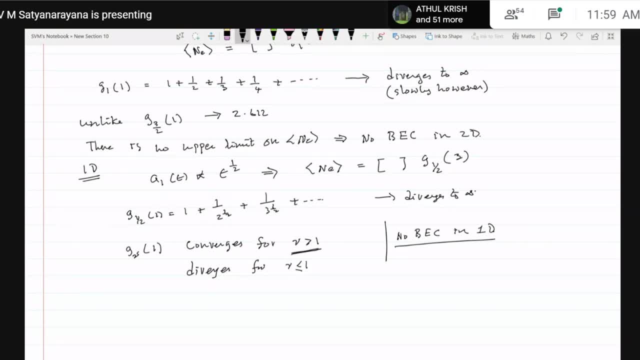 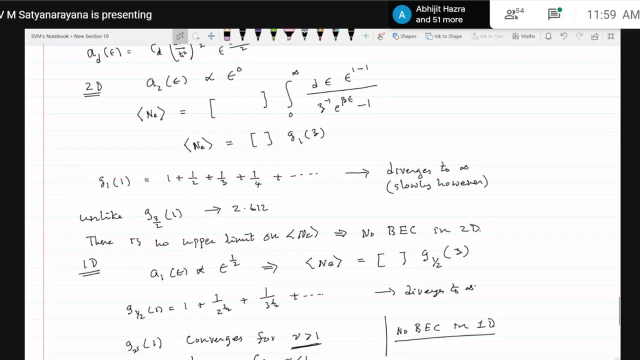 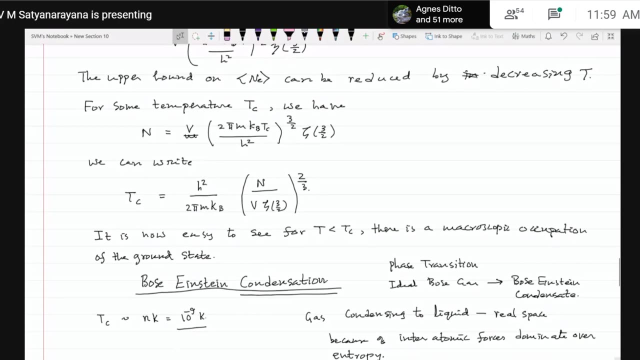 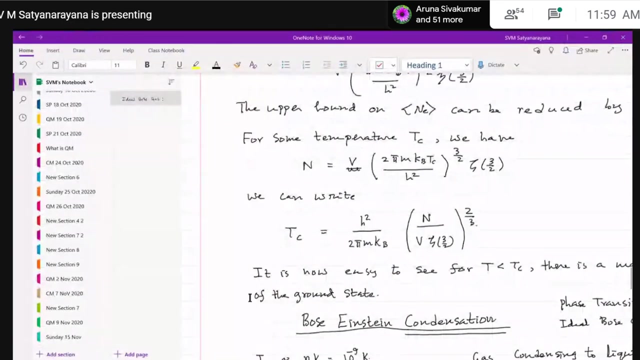 of boson constant communication. So this is as far as The situation in other dimensions less than 3 dimensions. So any questions at this point? Have you understood this one? Okay, Okay, Okay, Thank you, Thank you, Thank you. 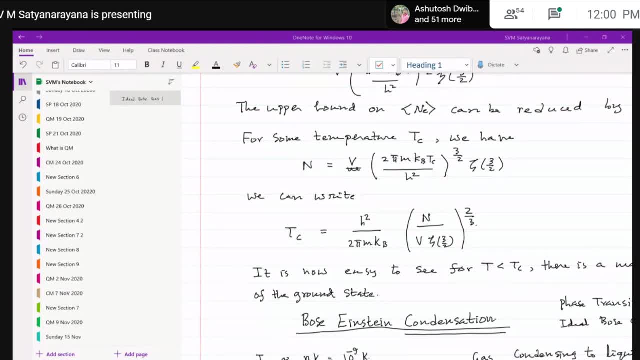 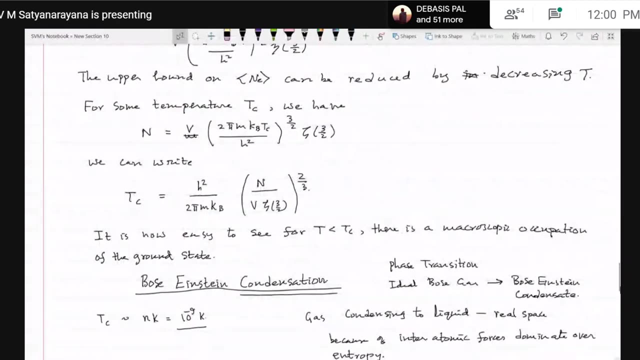 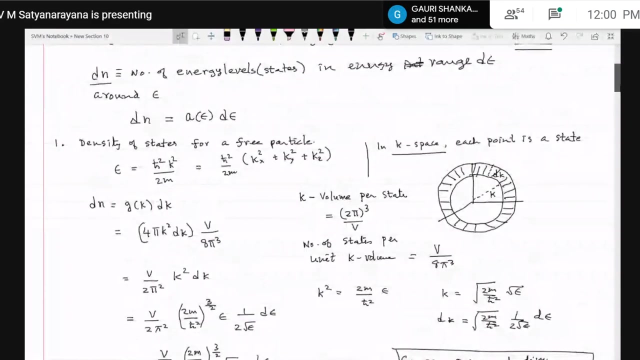 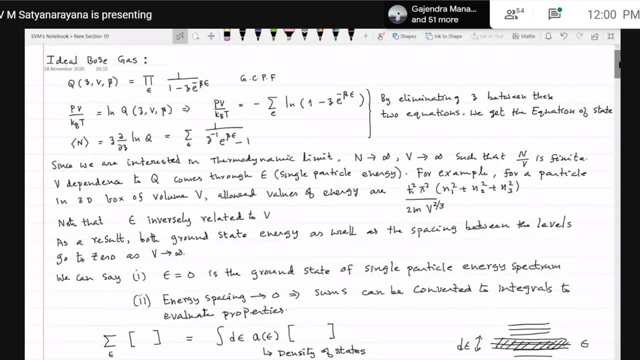 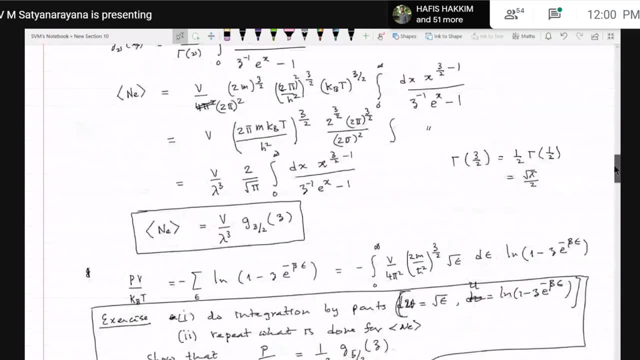 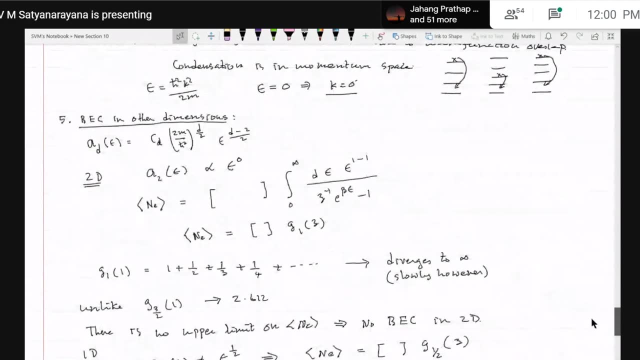 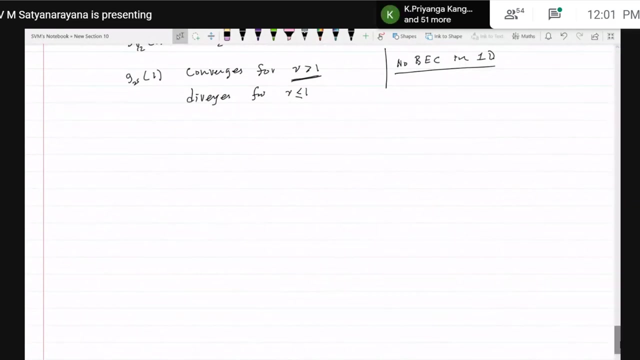 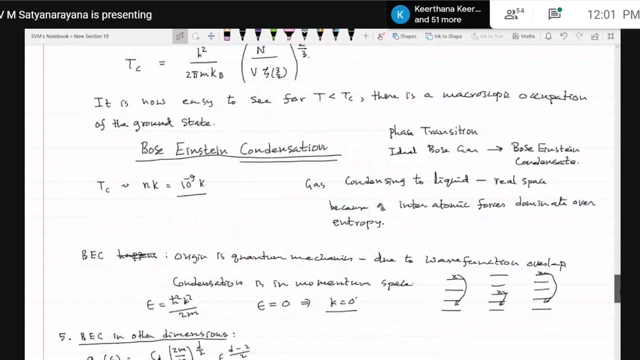 Whatever I have discussed today, it has arguments which are a combination of maths and physics. So if there is any question or if you have not understood something, you can ask. So one small doubt, like since the Bose instant condensate is not significant in the real state, like only in the momentum space it is considered right. 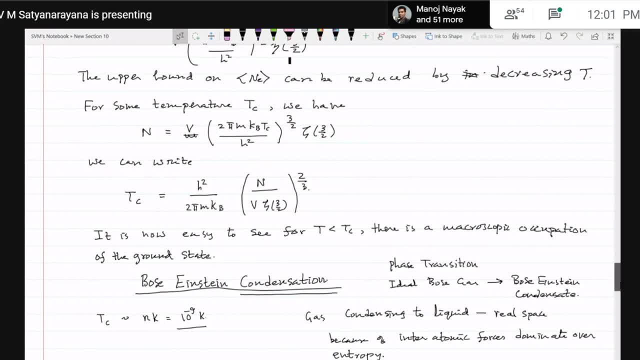 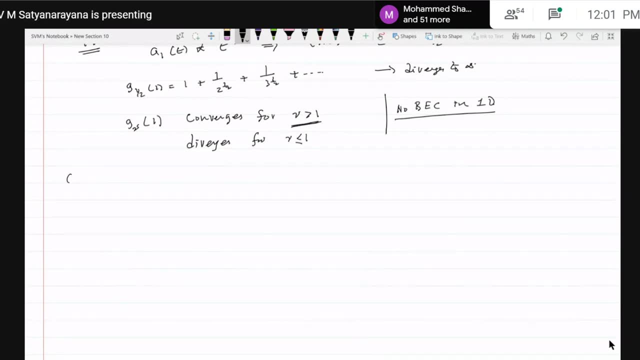 No, what I am trying to say is that suppose, let us say that you have. I am trying to distinguish between gas and liquid. This is also called condensation. So what I am trying to say is that if you have some kind of a volume, and then the gas molecules are there everywhere, like this, okay, they are there after the entire volume. 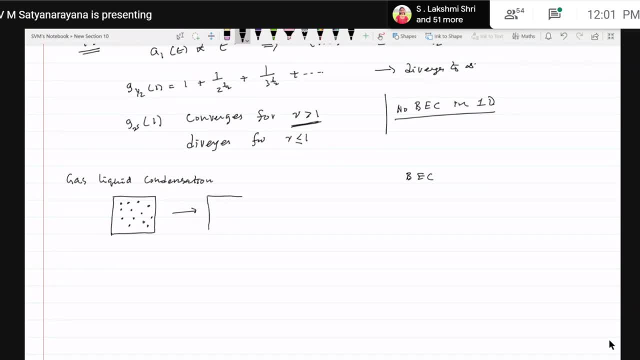 And when the condensation takes place, what happens is all these molecules will be somewhere on the bottom, Okay, And the liquid will be here, Okay. So this is gas and this is liquid. So this is how the gas and liquid condensation happens, because this condensation means condensation means just grouping together in some small volume, and that happens in the real space. 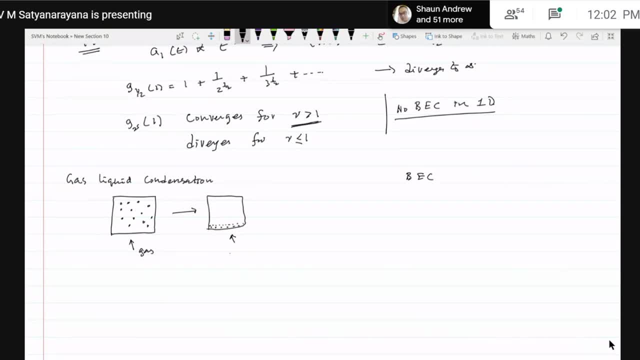 Now, in Bose Einstein condensation, what happens is that all these particles which are in the sealed state of the atmosphere lose their value. And in the case of the Bose Einstein condensation, what happens is that, you know, in the state, of the atmosphere, you might have a little bit of a diffusion. Okay, So if you are, you know a small amount of volume and you say you know you are moving to the other side, you might have a little bit of a diffusion. 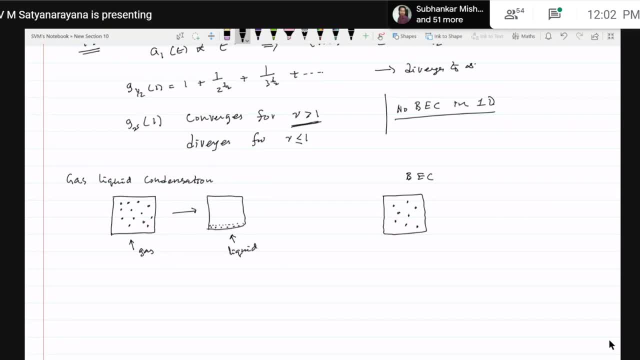 which are everywhere. So now I have to say that these guys are moving, This is moving with this momentum, This is moving with this momentum, This is moving with this momentum. So there is, that thing is also there for the gas here also, But it is not very important. 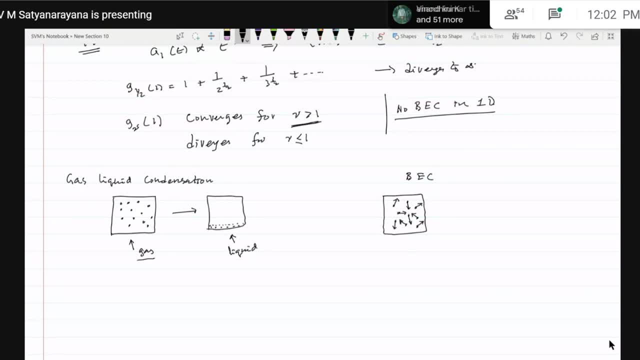 because there the dramatic thing that happens is in the real space. Now they are moving like this. Now, when Bose, Einstein condensation takes place, what happens is that these particles will be there only These particles will be there only, But they do not have arrows. That 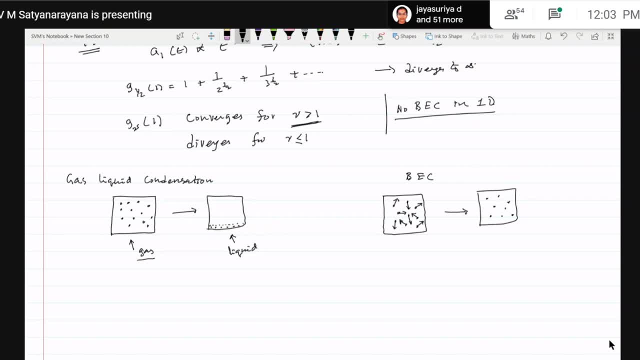 means their momentum has become zero. That means they are not moving. So there is no real space condensation here. But in the momentum space they all went to zero. Okay, So you still see that the gas has gas only, But now this gas looks as if it is. 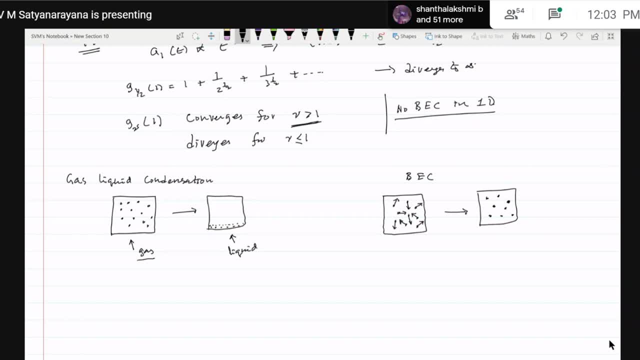 stuck, Okay, So the momentum will become zero. So you can say: this is your ideal Bose gas. Now, interestingly, why does this happen? is because of the overlap of the waveforms. Now, interestingly, why does this happen? is because of the overlap of the waveforms. 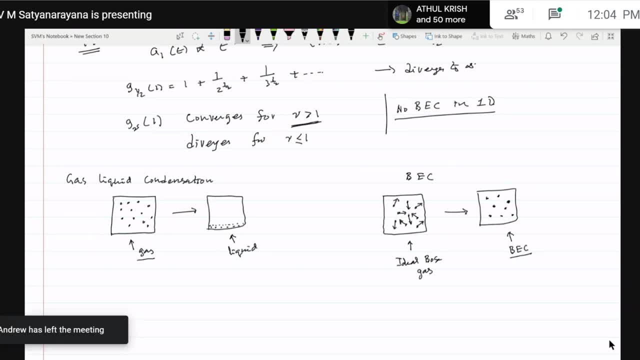 Now, interestingly, why does this happen? is because of the overlap of the waveforms. In this particular case, when it is in the case of ideal Bose gas, they are still different. Each one is moving independently of the other. There may be some correlation, but they are. 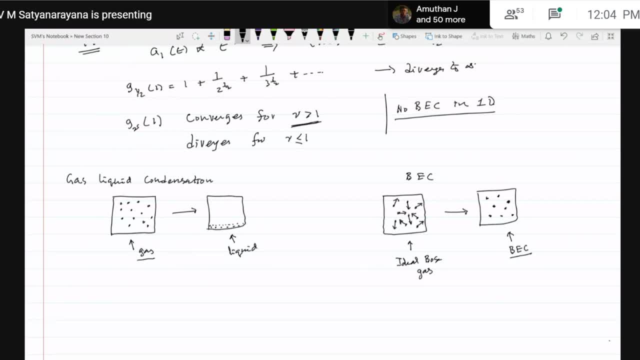 more or less they have. their independent particle status is there, But once Bose Einstein condensation happens, there is no independent status. All these particles are a part of some particle wave function. Okay, That is the difference. So in one dimension and two dimension this Bose Einstein condensation is known. Can you? 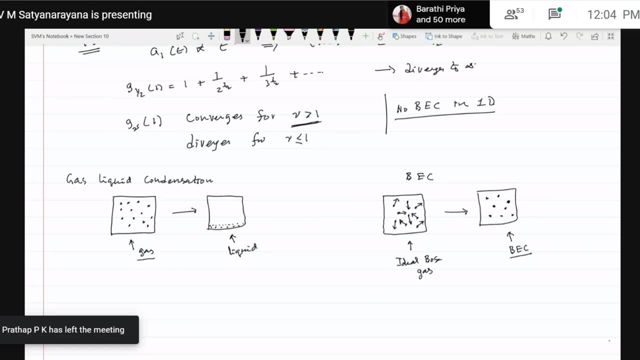 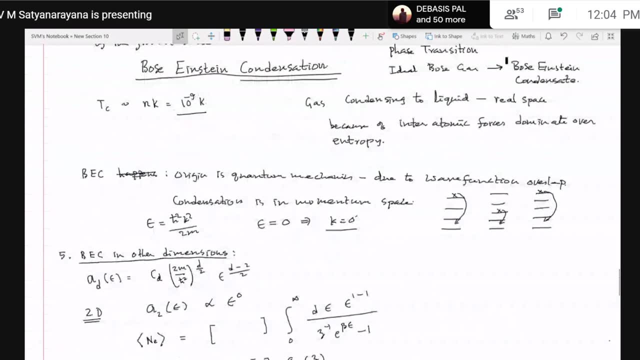 say that reason once more. I have just given a reason. mathematically, Yeah, Because the reason why there is a Bose Einstein condensation in three dimension is that there exists an upper limit on the, on the, on the occupation number of the excited state, average occupation number of the excited states And. 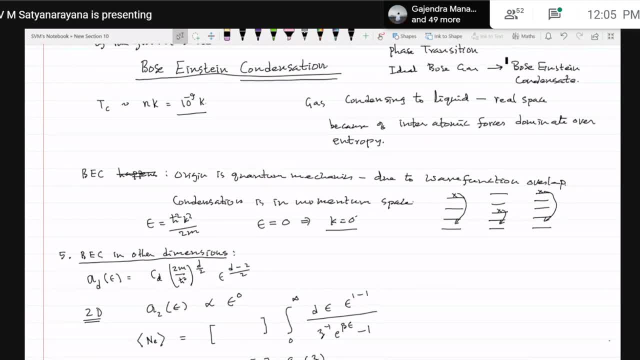 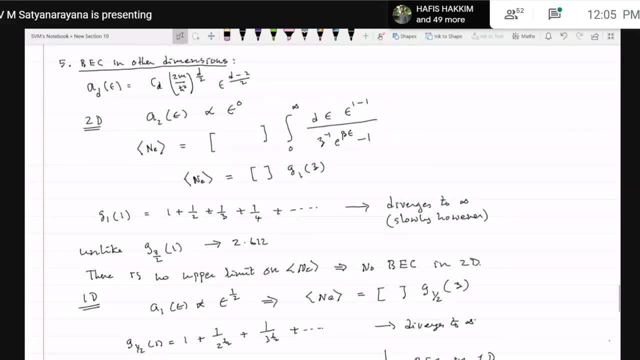 that upper limit is coming because of the convergence of this Bose- Einstein function to a particular value, But in this case it's because of the dependence of the density of states on the energy. you have this different Bose Einstein condensation In this case. 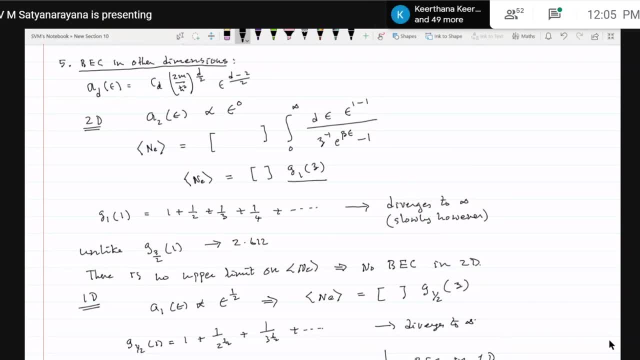 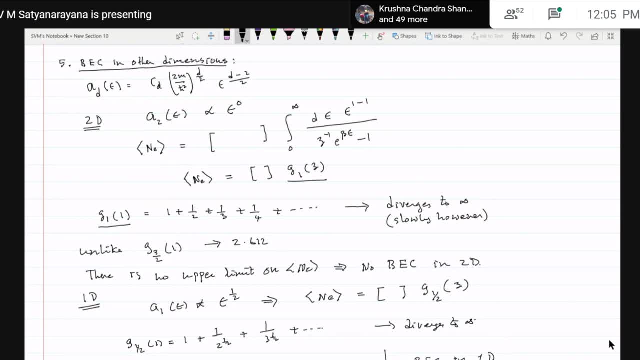 greater than all z right. So monotonic increasing function of z is valid mathematically for this function. So this is diverging. That means there is no upper limit. The upper limit is infinity. That means you go on adding particles. then there is no macroscopic accuracy. 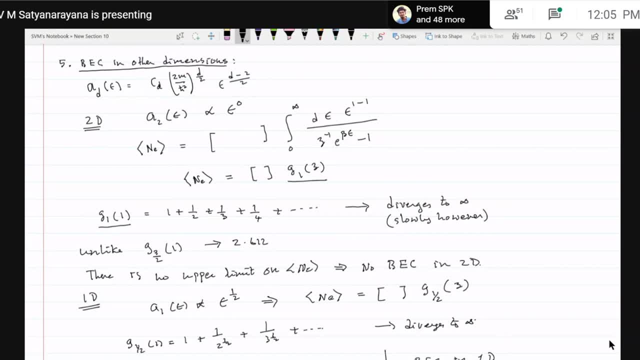 of the ground state, both in 1-D and 2-D. Okay, sir, But I think it is an interesting question to ask and think about, Because when you think and think, what does it physically mean? yes, sir, exactly an interesting question to think. 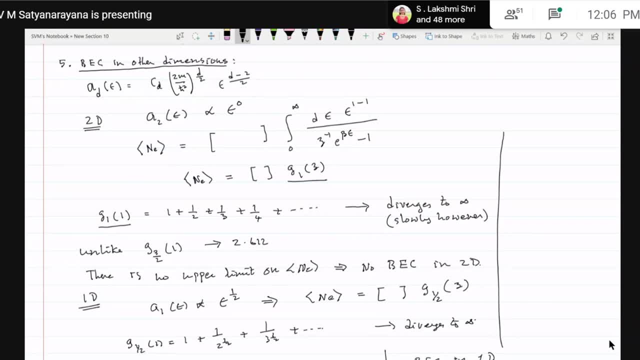 and i encourage you to think about it. so what does that mean physically? and this? this is another, another instance where how deeply physics and mathematics are interconnected, because i i just argue from the mathematical property of a function and that determines, uh, the physics. that means the intimate connection between mathematics and 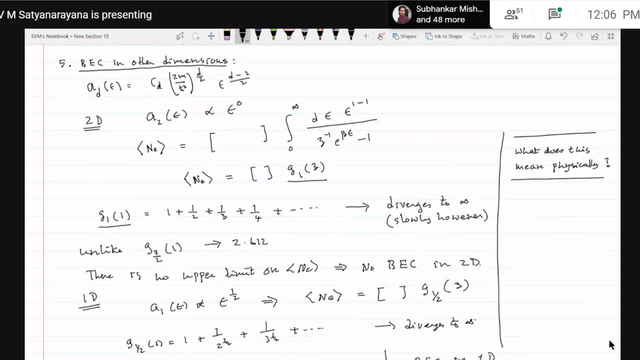 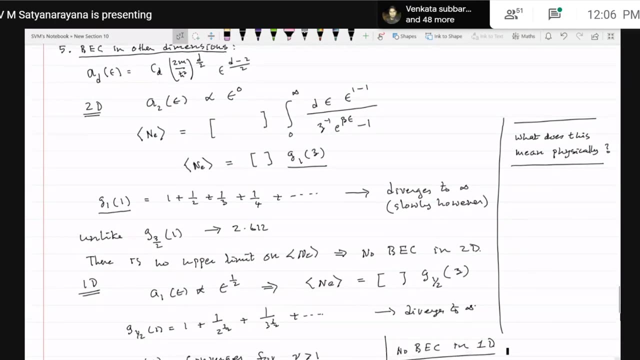 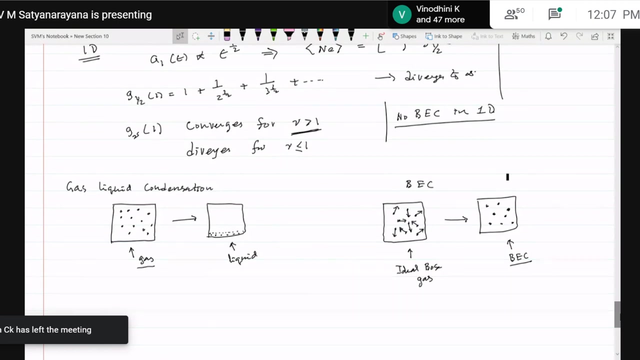 physics as nature- uh, nature- obeys, is something which is very, very promising and very exciting here. so, of course, this is a good question to ask and i will encourage you to think about it and we can come back to the question after you, after you sufficiently think about it, okay, so thank you. 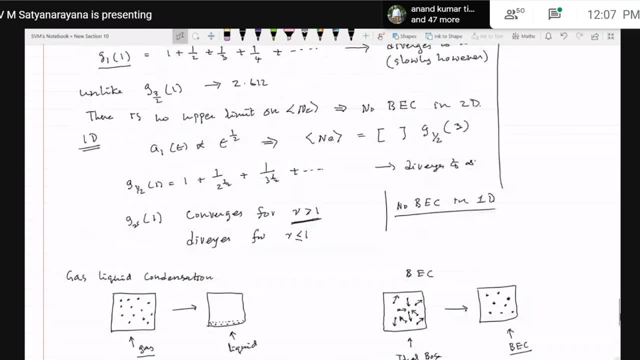 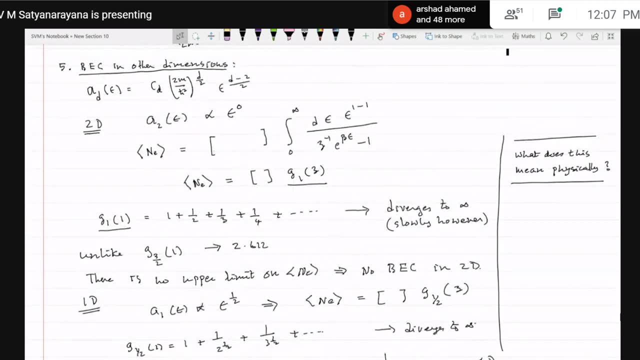 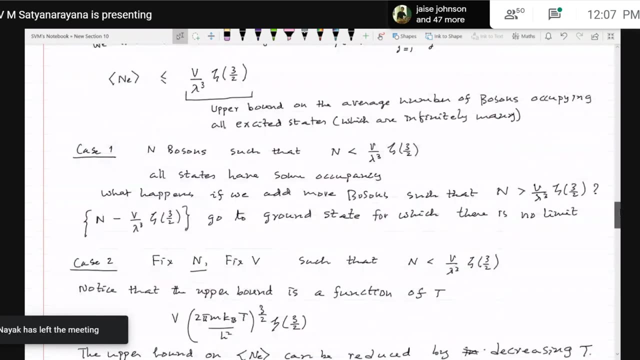 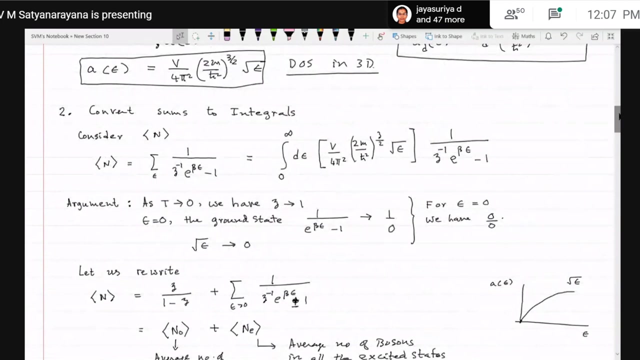 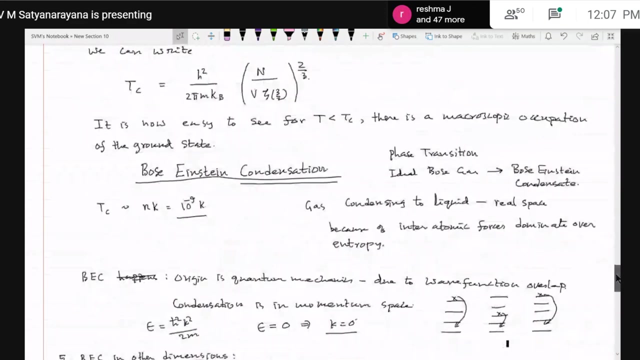 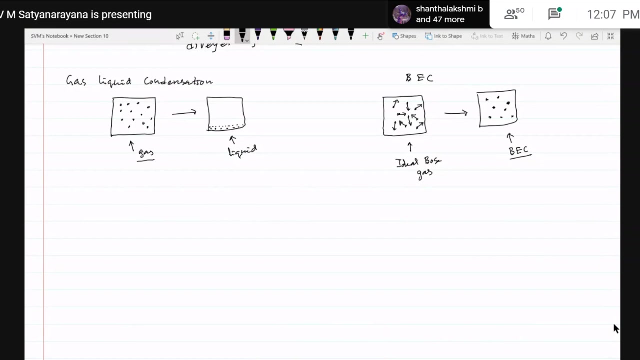 excuse me, sir, can you go back to point two? i'm not sure whether my numbers are continuous. can you explain that? t tending to zero, z tends to one. okay, t tending to zero, that tends to one. so i want you to recall that we had this expression that the average number of 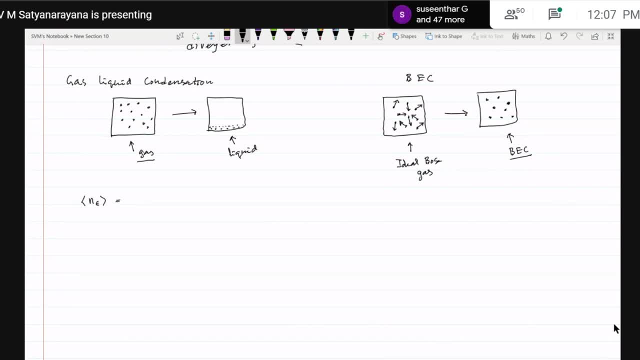 is in energy, is equal to 1 by e, to the x minus 1, where x is equal to epsilon minus 2 by k- d. This is what we have Now. we try to plot this function as a function of x with average n. Then we notice that x has to be positive. 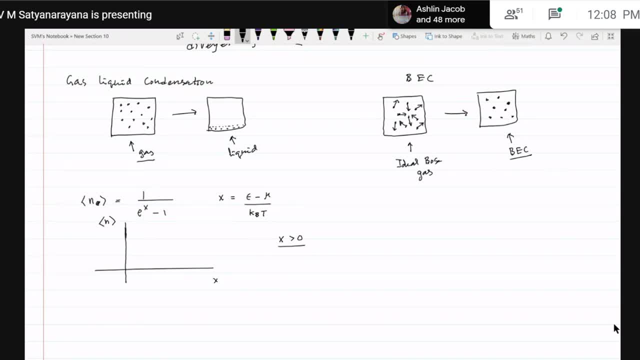 This argument you remember: if x is negative, then x has to be positive. So what happens? If x is negative, x is negative. this implies n becomes negative, which is unphysical, because this is average of n. So because of that, x has to be positive. So the lowest value of x is the lowest. 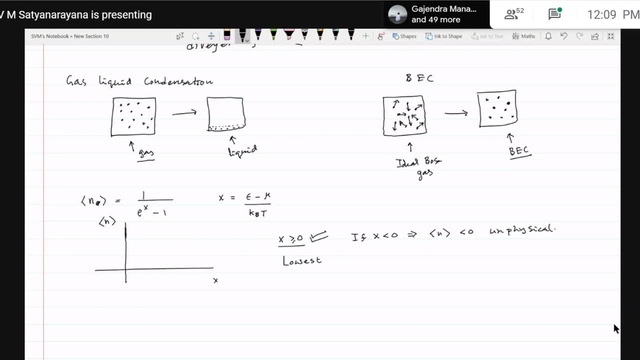 value of x is the highest, And highest value of x can be infinitely, And the highest value of x is the highest. So we have said that now what happens? as x goes to 0, this function will go to infinity, and then it is. So this is the function. So that means suppose, let us say that we have 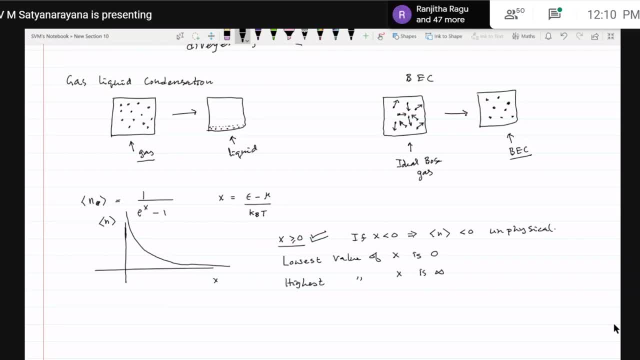 So suppose if I fix my epsilon, fix epsilon is equal to, let us say, 0, ground state. I am interested in this ground state occupancy. So then my x is equal to minus infinity, So minus mu by k. So what should mu be, If mu is anything which is positive? Now let us 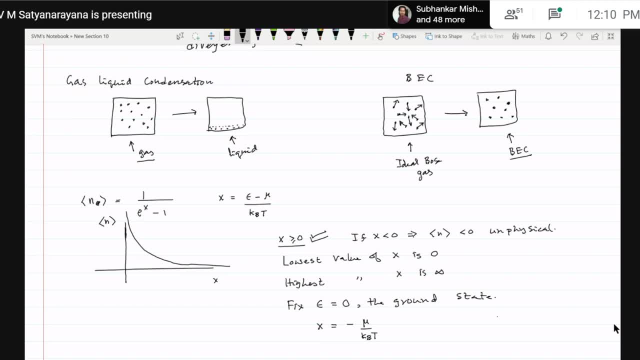 say: we look at what happens if t goes to 0.. t goes to 0,, this x goes to x, t goes to 0.. So what happens if t goes to 0,? this x goes to x, t goes to 0.. So what happens if t goes? 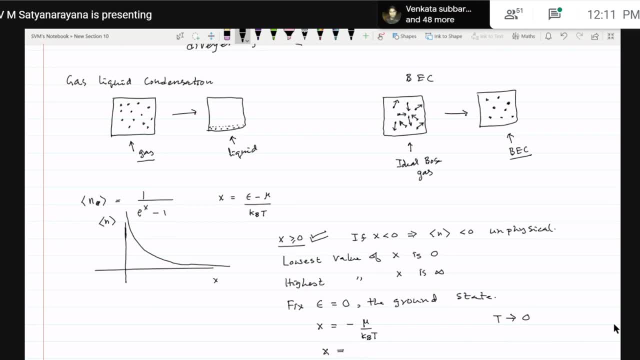 to 0?? Let us say if t goes to 0. So we will write: mu has to be equal to 0 in this case. So that means mu has to be equal to 0. Why? Because since x is greater than 0, since x. 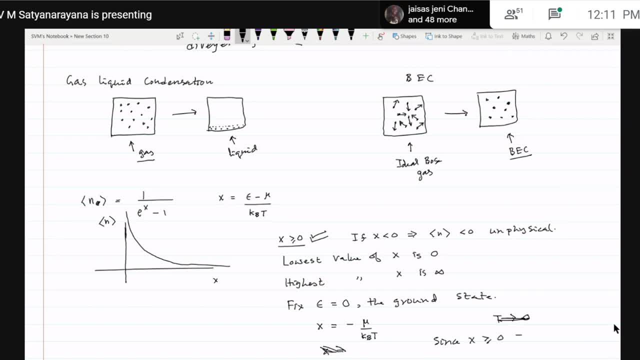 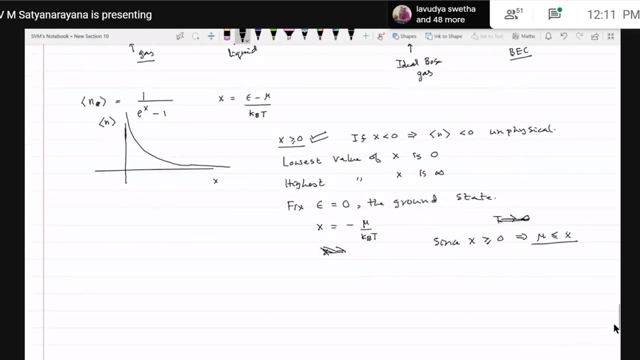 has to be greater than or equal to 0,. this implies your mu mu has to be less than or x, you have to be less than or equal, and you have to be less than or equal to epsilon. so if epsilon is zero, then mu has to be less than or equal to g. 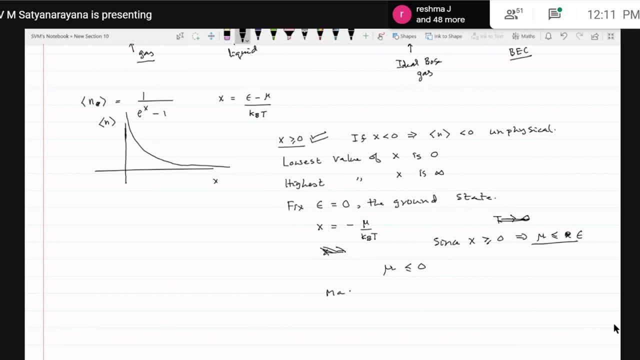 so the maximum value of mu, the maximum value of mu, equal to g. and what is our z? our z is equal to e, to the power mu by k. okay, so you have. you have a situation where maximum value of z, maximum value of z is equal to 1. 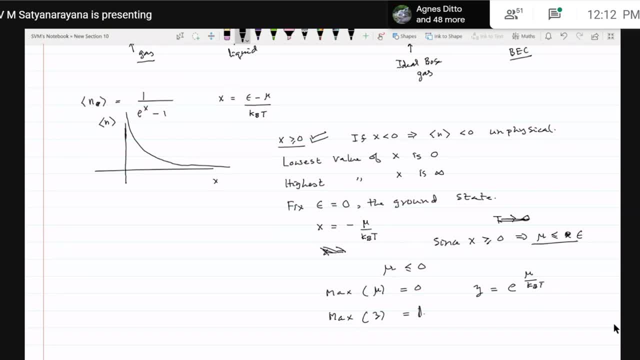 because mu is zero. so it is like: uh minus infinity is less than mu, less than or equal to zero. this directly gets converted to zero. less than or equal to me, sorry, less than or equal to z, less than or equal to one, sir, but uh mu goes to zero. 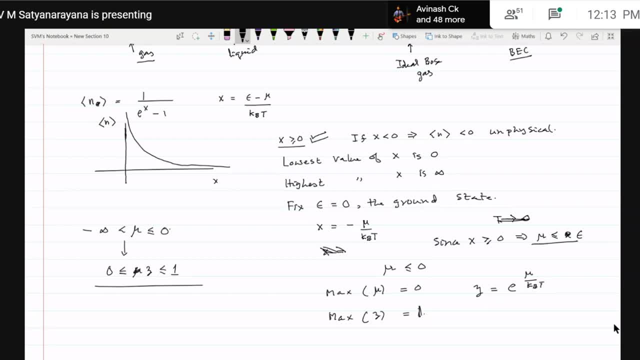 and t also goes to zero, sir. so we have e to the power, zero by zero. yeah, yeah, the point is that uh mu does not go to zero. uh mu is equal to zero. okay, mu is a c for uh for a fixed. which energy is occupation? we are looking. 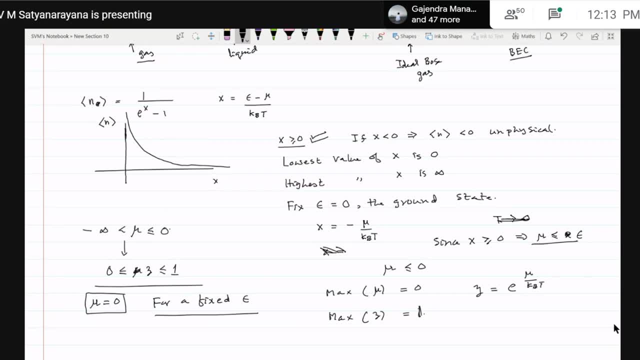 at. so for a fixed energy, mu is. mu is equal to zero. okay, if you say, this will be equal to zero and u is equal to zero. so we have a problem for t equal to zero and so, as t goes to zero, this, this is already zero. so 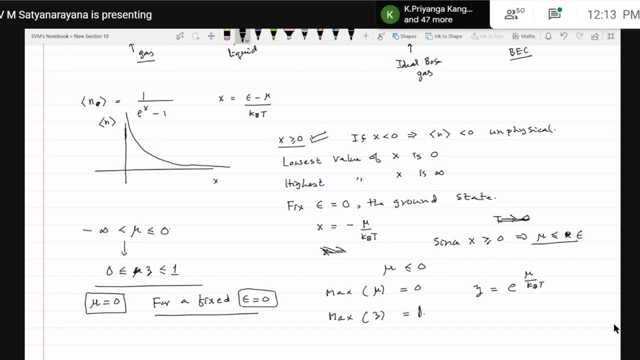 zero divided by some small value, uh will also be zero. only when t becomes exactly equal to zero we have that problem, but that is something which we are not interested in. okay, very close to zero. also, because mu is identically equal to zero, we will have z there. 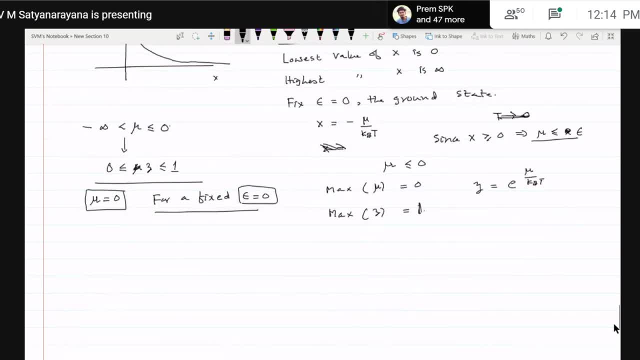 at. it is in the following: so let us say that, let us say that n 0 is the average number of particles, average number of particles in the ground state, let us say in epsilon, equal to zero. so we know that this can be written as, because we had written that by separating this term, 1 minus z. so this i can write it as 1 minus z. 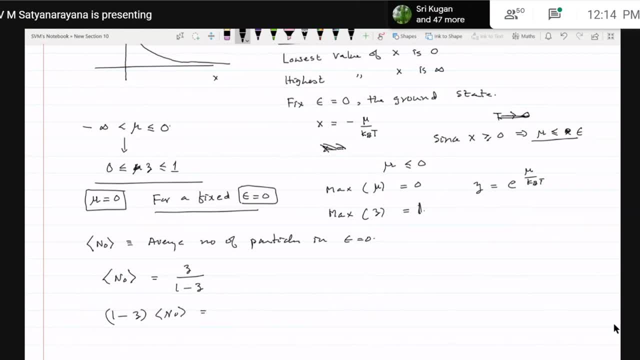 into average n 0 equal to z. or you can write this: z as average n 0 divided by average n 0 plus 1. correct. now you see what happens in in the case when b e c, so b e c, b e c occurs, occurs when p goes to p becomes very small. okay, so that means your average n 0 is very large. 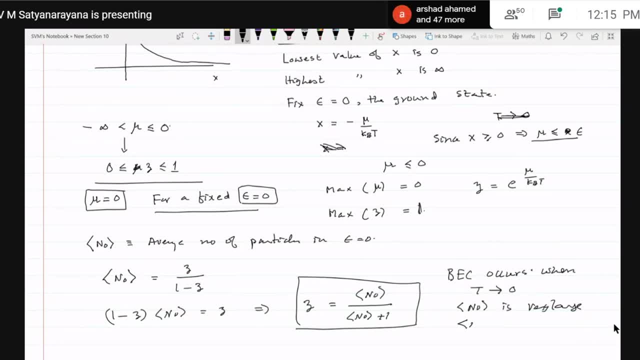 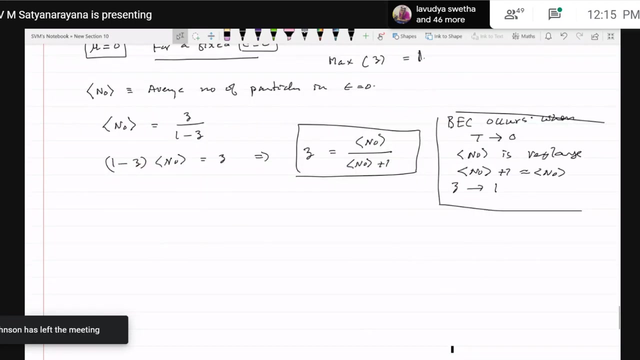 average when zero is very large. so i can write this average zero plus one as average n zeros, because this is very large. so that once again tells you that this z goes to one. okay, this is uh by looking at the average occupation number in the ground state. 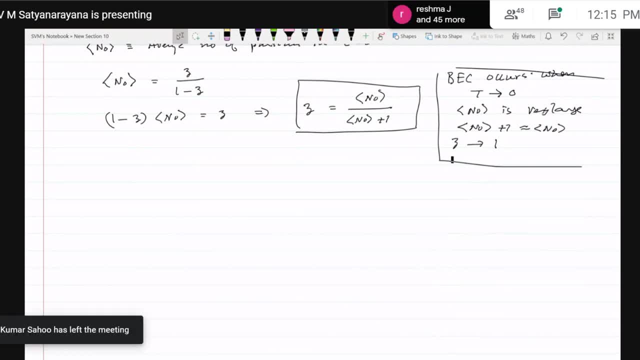 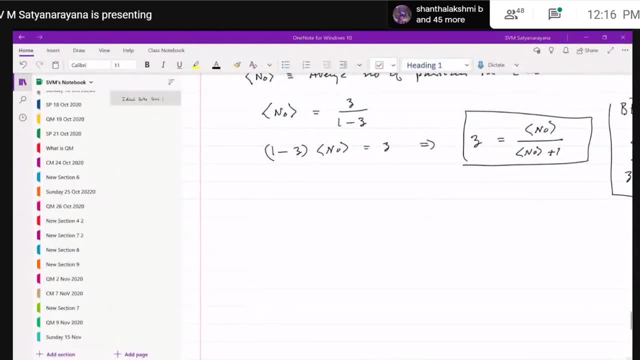 okay, here i have uh andよろ. i keep writing my sorry. any other questions? uh, alas, uh, in other minds ート uh have zero momentum, so it won't uh more. uh, whatever extra particle we add, we add to that system, it won't move. um, actually, i i cannot say that because, uh, we have no access to any. 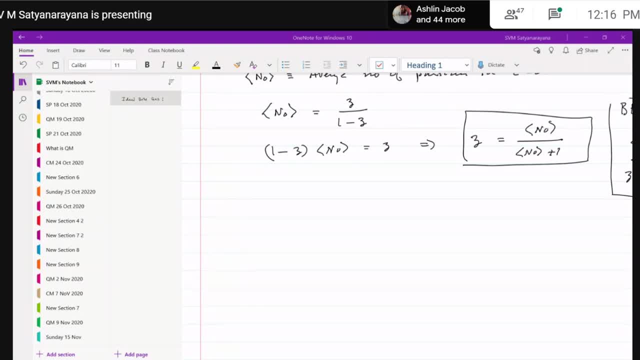 information of individual particles once you add it to the system. okay, i can only talk in terms of average number. okay, so suppose if i have an upper limit and if i am adding more particles than this upper limit, so whatever number that we have, total number minus upper limit, will go to the 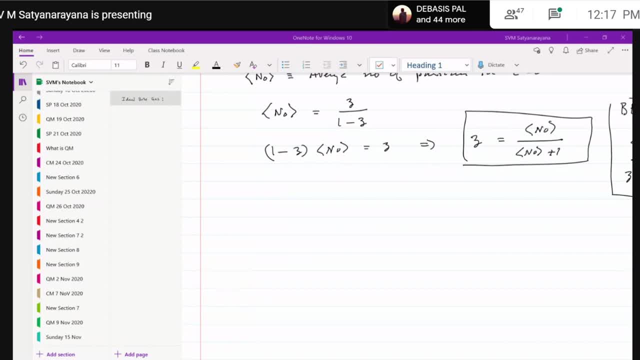 ground state. i will not know which one will go to ground state. that means which one will move, which one will not move. there won't be any uh way of way of uh knowing that information. okay, you understand. so these, these are like average, uh, average statements that we have made. 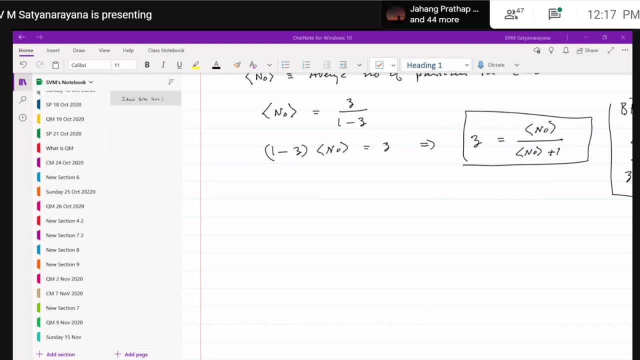 so average number of particles that are occupying the ground state will be total number minus the upper limit. so some of the particle will move. some particles will move. definitely there is going to be a mixed phase. for t less than tc there's going to be mixed phase. but what is interesting is that 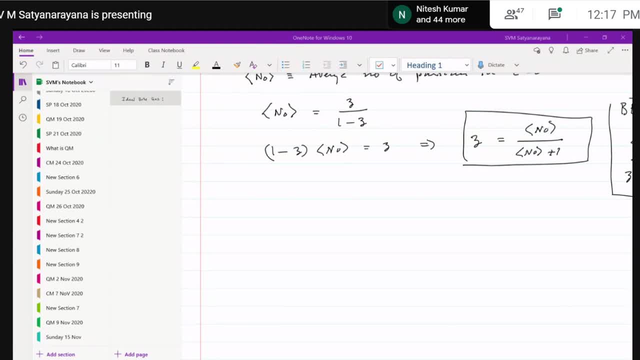 large number of them will not move. okay, any other questions, sir? uh, here for this case, uh, for this ideal, um boson, guess, are this particle interacting with each other? no, this is an ideal guess. so i will guess, sir, but uh, in, in real system, the particle have some? uh, particle interacts with each other. 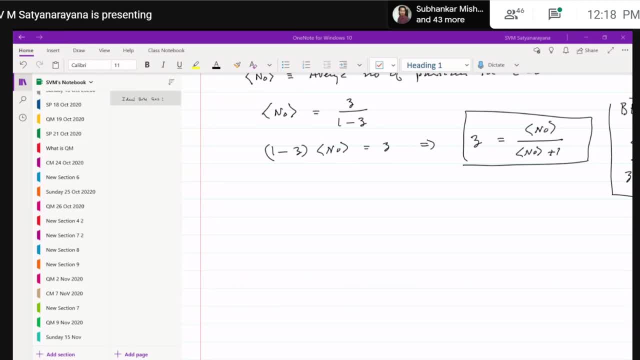 so then also, we got like: experimentally, scientists have got, okay, there is some, yeah. so essentially what they do in experiment is, uh, they try to take a system to be extremely dilute so that there is no interaction among themselves, no question. so they take the, they take this whatever uh gas of atoms, they take them to be 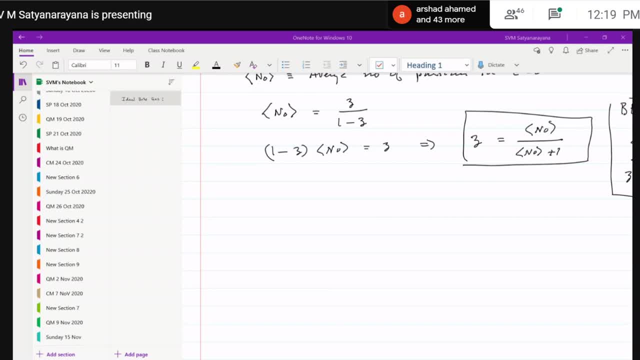 very dilute that interactions can be neglected. they take them also, so dilute that, see, they have. imagine that you take a gas and then decrease the temperature and decrease the temperature to the nano kelvin. do you think it is possible to maintain them as a gas because normal liquid condensation solid. all those things will happen. much higher temperature. 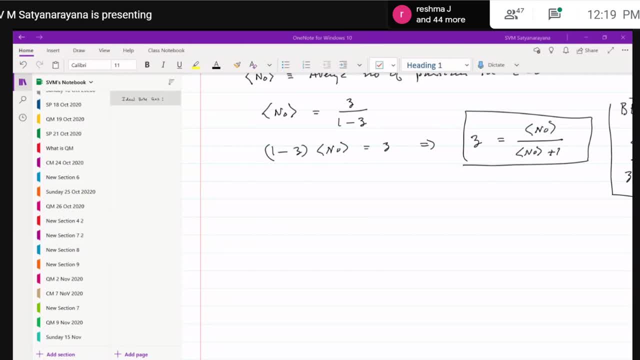 right, yes, like any gas, that will become liquid, liquid become solid. now you have to understand how to avoid this one, because we want to keep this as a gas up to nano kelvin temperature, which is a big challenge, and that is why it took 70- 80 years to experimentally realize this one. 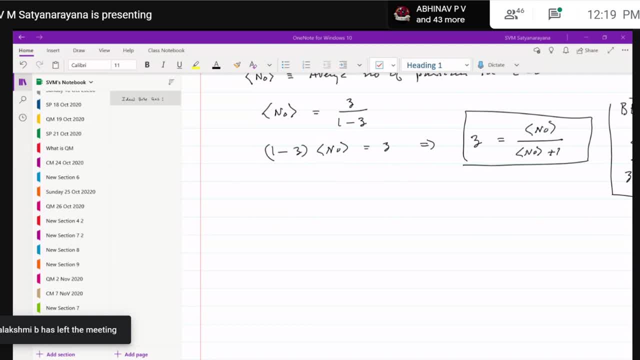 so they can. yeah, like they have to choose some substance that will have very low. uh, you choose anything. for example, boiran condensation has been achieved in rubidium atoms, in potassium atoms, sodium atoms, lithium atoms, hydrogen atoms like that, so these all have interactions. you know that this lithium becomes liquid, lithium becomes solid, right. 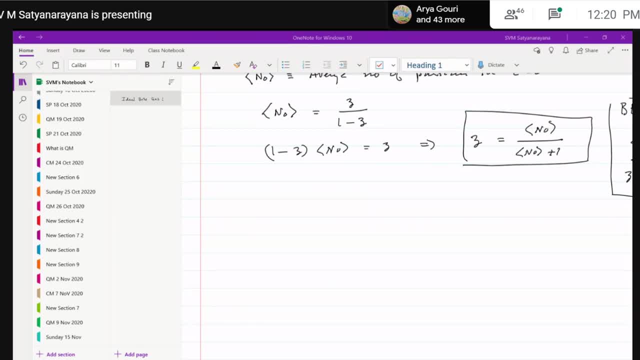 these things have to be avoided. so if you want to avoid, you have to understand how this phase transition takes place to start with. okay, that that understanding has to be there. how a gas becomes liquid. now, a gas becomes liquid because, you see, gas molecules are just gas particles, are just flying around. now they have to. 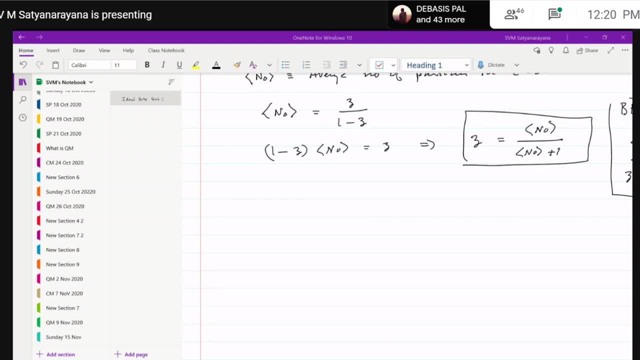 start agglomerating now. they have to start becoming lumps and become liquid means there should be something called some nucleation. should happen, then there should be growth of those particles and that is how it happens. now people understood that such a kind of thing happens when you have some impurities. 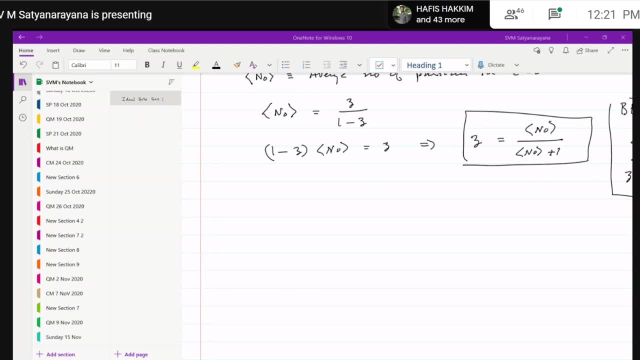 okay, around the impurities there will be some kind of a conglomeration of particles and that will lead to condensation, when the real space condensation. so one has to one helps. one has to choose this: so pure our substance, a so pure a set of particles that there are no impurities. 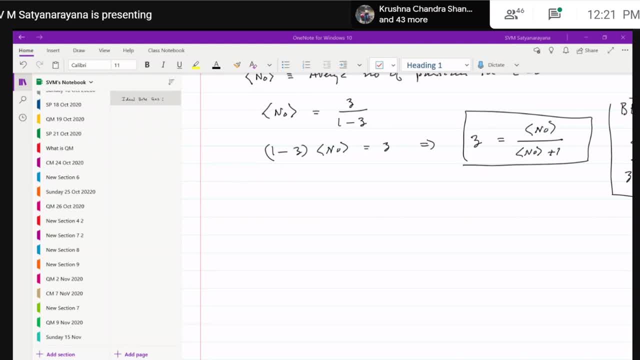 and second thing is that these particles we each are flying around in the gaseous space. they collide in future them. okay, and normally what happens when two particles come together and collide? they will simply exchange their momentum and go away. they will not stick to the. but if 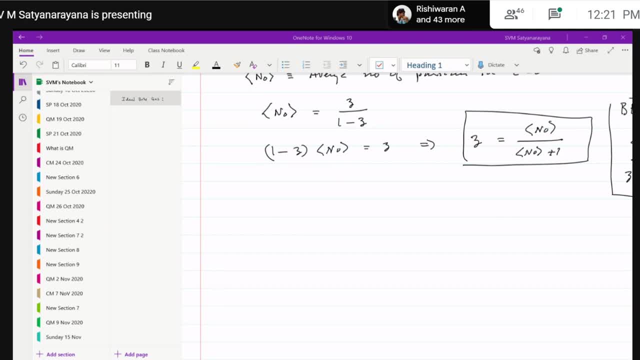 there are three particles coming together then, So two of them can stick together and third particle can take all the momentum and then go away. Now, these two particles then onwards can fly together, then that can become three particles and so on. So three particle collisions is one of the very important criteria to have condensation. 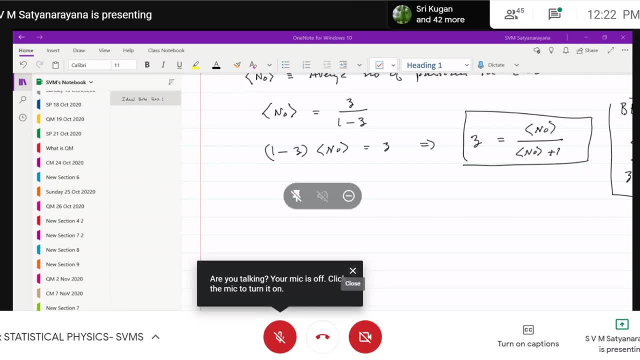 Now they have to choose their system so dilute that the probability of three particle collisions is very, very less. So, like that they have, they have to keep maintain this gas as gas up to nanokelvin temperature. that is the challenge, Okay, sir. so one more thing. sir, like the technique you have applied here, like separating the 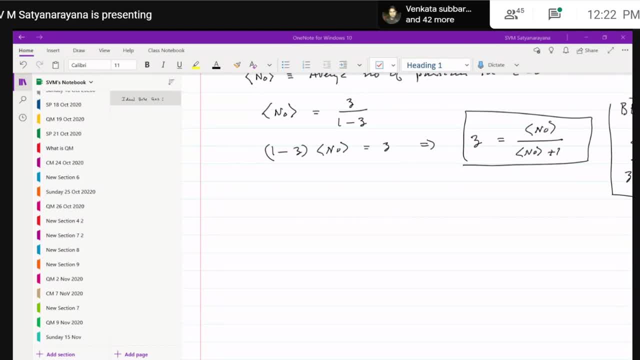 ground state part and the excited state part. Something similar I have seen In, like calculation of Green's function for Coulomb potential, but it is different in one sense, but it is similar in one sense that in two dimension, when we are talking about Green's function in two dimension, similar like this logarithmic series, comes. 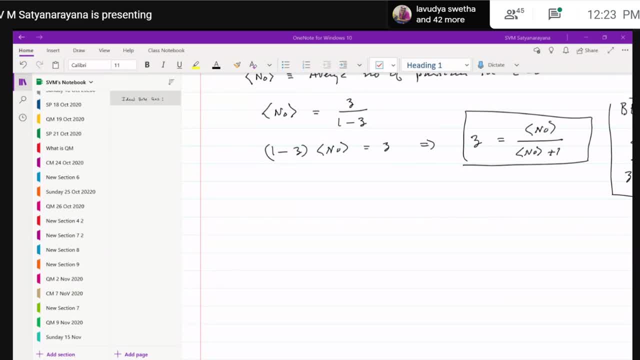 Like suppose we have a system where charged particles are there like and we try to like, we try, We arrange them in two dimensional, like two dimensional surface, and try to find this Coulomb potential or the Green's function for the Coulomb potential. like there also comes a logarithmic. 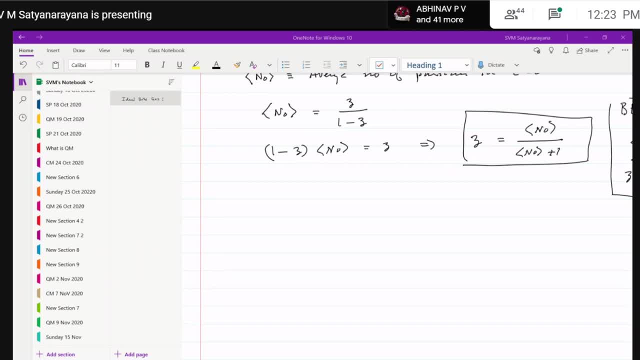 function and here also there is a connection of logarithmic function. Are these things are anyway related? No, I think there is no relation between these two. see, this logarithmic divergence only comes for that. You know, That is because we have the density of states dependence on the energy, like that. 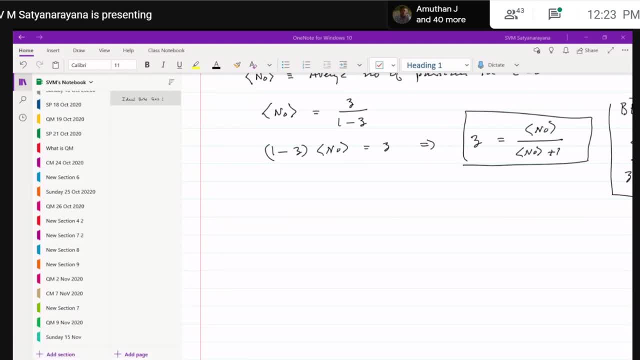 So I think there is no physical comparison between these two, But many times there are different physical situations which will mathematically use the same kind of technique. that is possible, But mathematical similarity does not necessarily Okay. Thank you, sir, Yeah. 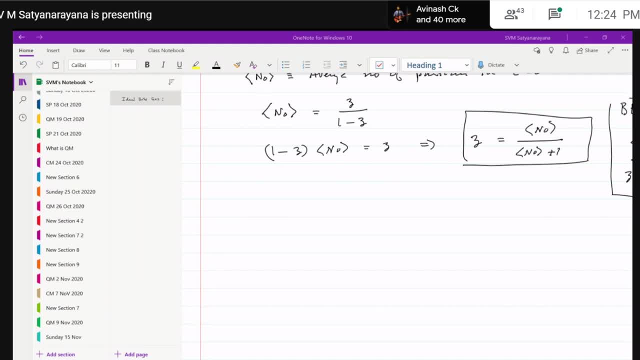 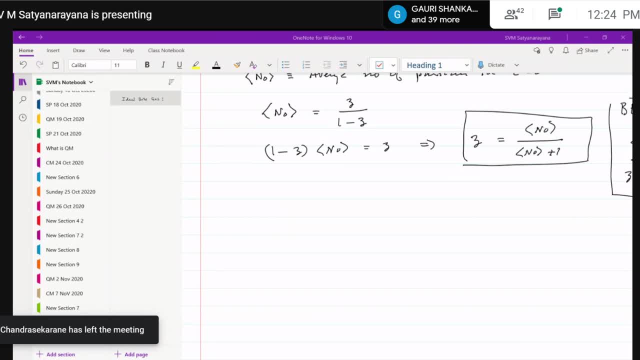 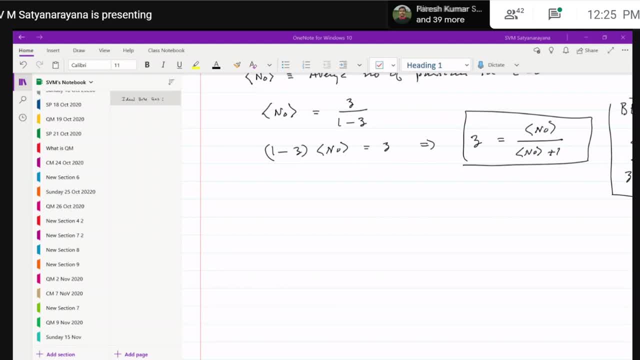 Yes, Yes, Yes, Since there is no interaction with theimentos. Yes, In reality. see, there are some interactions in reality, But what we were saying is that whenever you are trying to do some experiments, you must also choose your parameters in such a way that the interactions can be neglected. 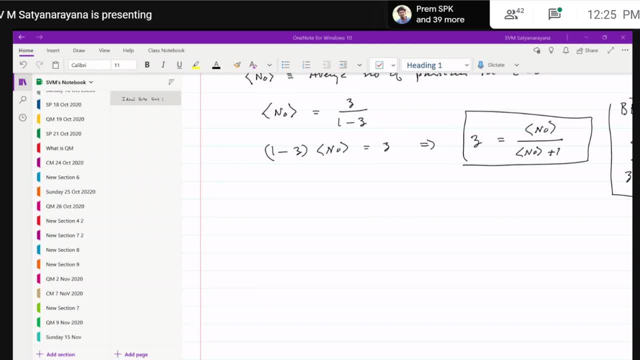 There is no non-interaction within this. ideally, If you can interact, For example夞ğ challenge, Every gas can be considered as an ideal gas: at high temperature, low density. That is because at high temperature they are moving so fast, but they do not give enough. 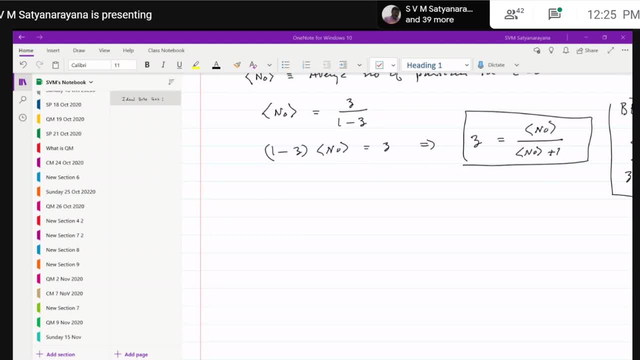 time for them to talk to each other and interact And low density. they are so far away from each other. there is no interaction, So the interactions can be neglected, but there is nothing like a non-interacting system. Some interaction will be there, because all the interactions are long-range interactions. 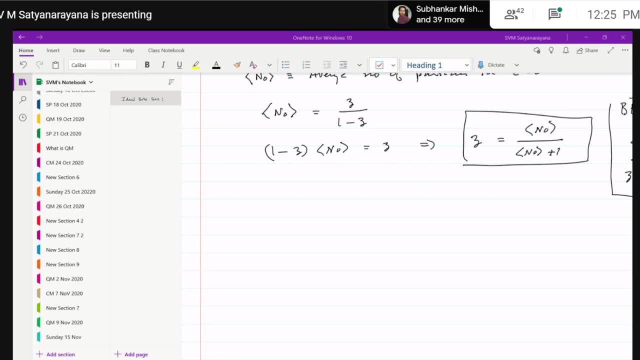 So it is essentially an approximate notion. but when we do theory we consider the non-interacting system, because that is easy to handle, And then you can also do an experiment with an appropriate choice of conditions. What I am thinking is, if we have a gas station, we can also do a non-interacting system. 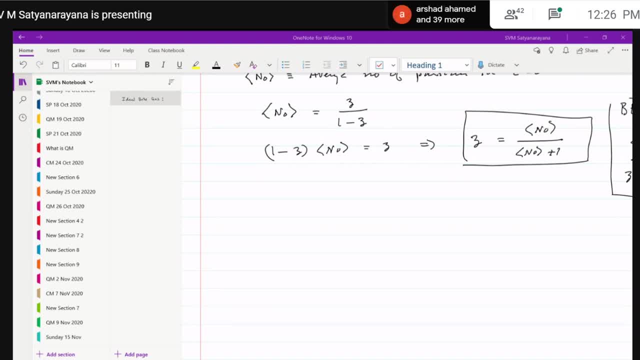 In reality we have some systems which are very loosely interacting. Then this Bose-Einstein condensation can happen at a higher temperature. right, Tc can be large. Yes, So is that possible. Basically, the idea is, why it is not happening at very high temperature, at reasonably high. 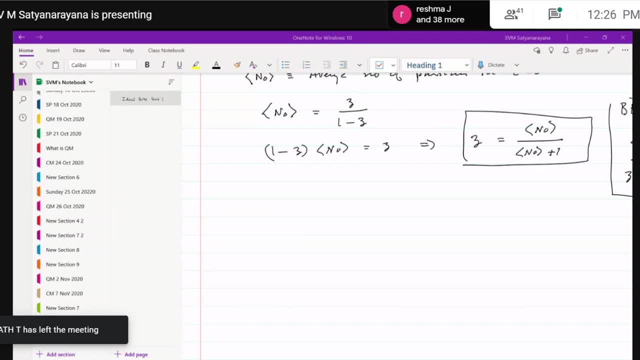 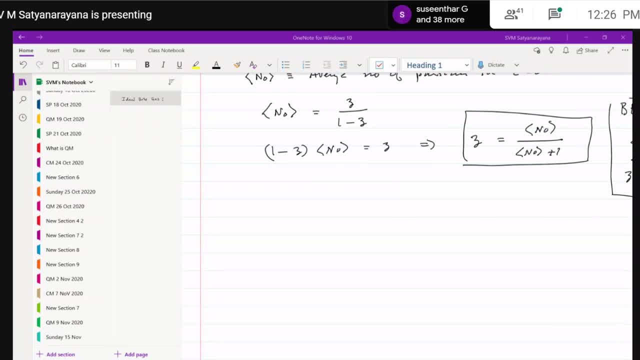 Okay, We are starting with a non-interacting system, So this is fine. But what happens when this Bose condensation happens is that when these overlap of wave functions take place- And this overlap of wave functions means, for example, you take an atom- 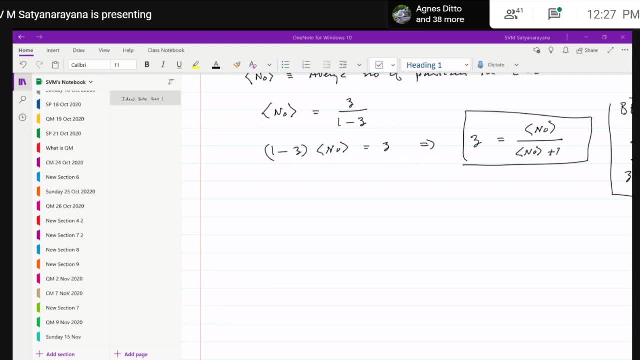 compared to any quantum mechanical system, And the de Broglie wavelength of the atom is very small. Now you want to increase it such that the de Broglie wavelength becomes of the order of the size of the cell in which you are keeping these atoms. And that requires 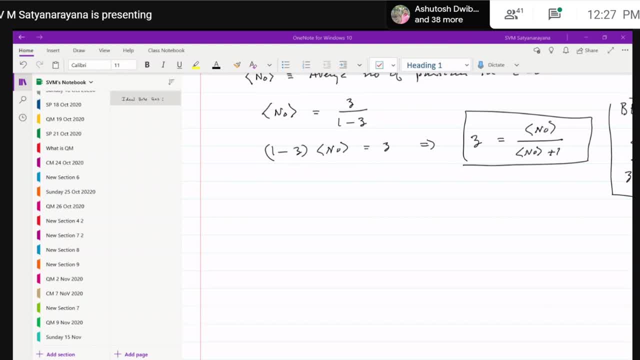 you to go to lower and lower temperature. So that is essentially, that is why I said that this transition, the origin of this transition, is quantum mechanical. So you want to understand how to get it at a higher temperature? then we should consider smaller and smaller particles. 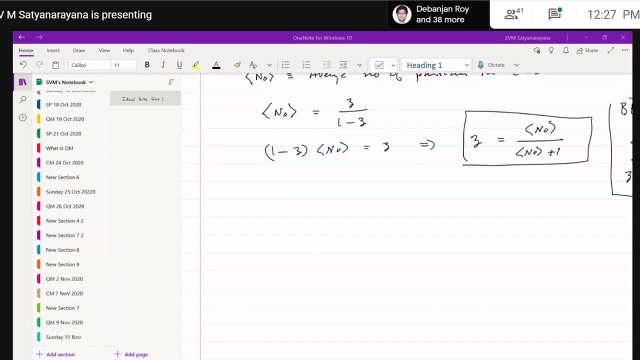 So some kind of bosons which are very small particles. But we do not have such particles, elementary particles, like electrons. Okay, sir, Sir. another doubt I have is: sir, this chemical potential is a thermodynamic parameter, right, Like pressure, temperature, volume, like that. So how to physically increase? 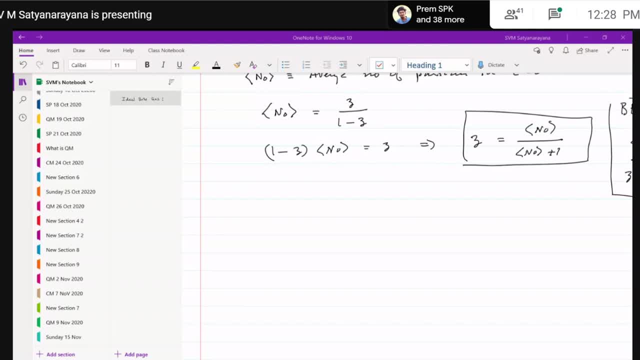 or decrease that, Because we know how to physically increase pressure and decrease pressure Temperature, we also can do So, how to do that for chemical potential. So you have to. you have to do that by changing, by changing the environment only Because. 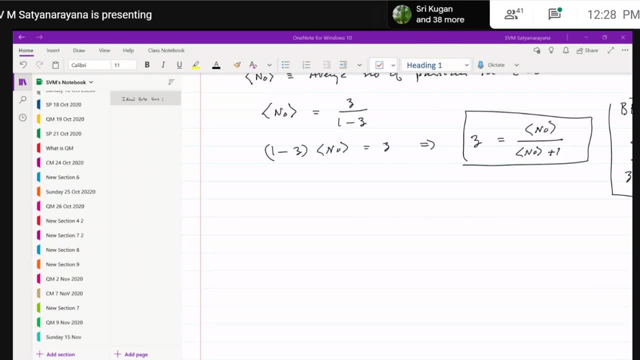 chemical potential is the property of, property of a bar with which your system is interacting, Such that there is there is a kind of particles going from outside to inside or inside to outside. Okay, So the thermodynamic parameters is controlled Such that at a constant chemical potential, you have an average number of particles are. 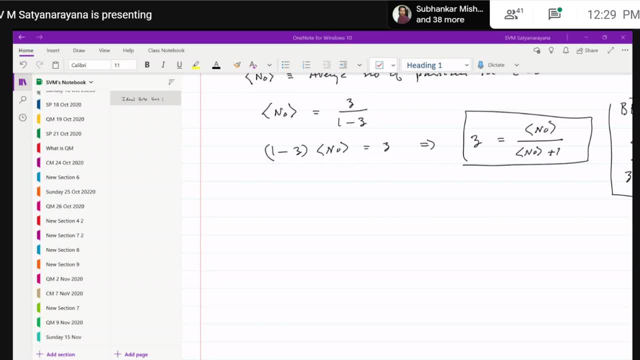 fixed. Okay, So it has to be controlled by- by the environment, For example. for example, if you consider, if you consider a metal, there are 3 electrons inside the metal, But those electrons are not that perfect Okay. 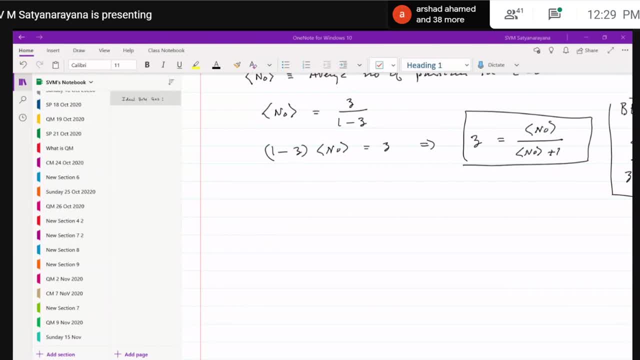 But those three electrons are not that free that they can just flow out of the metal, Correct? Yes, sir, If I just take the metal and keep it in the environment, the electrons will not flow out on their own Right. Yes, sir. 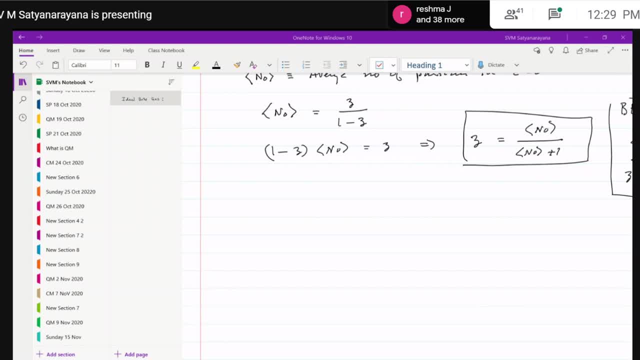 But there is something called a work function, So you have to give some energy so that it overcomes that barrier and then comes out. But now, instead of just putting this metal in the open space, suppose if I put that in some other environment, like I can put it in plasma or in some other environment. 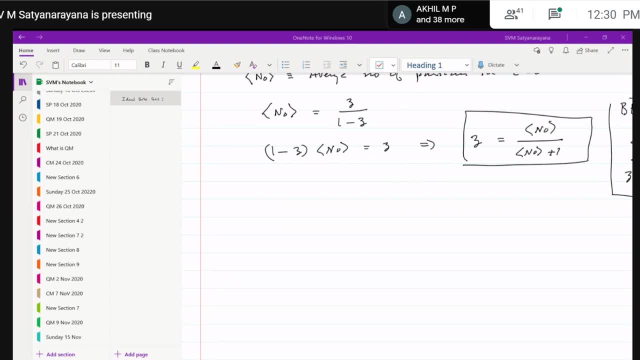 then there is a different chemical potential that these electrons will see. So it is always changed by changing the path. Okay, Sir, the particles can exchange. There is a difference between the system and the surrounding, the bath and the system, right? 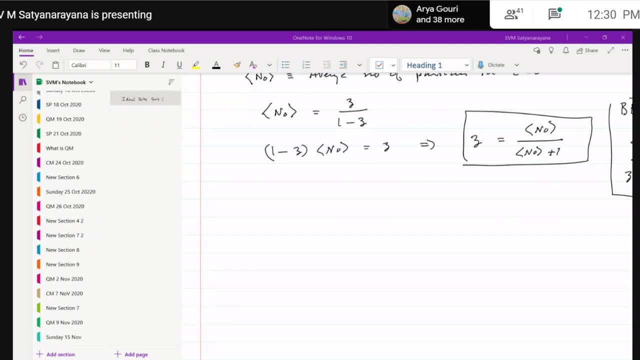 So, sir, in that case the bath has to be made up of the same kind of particles, right? Yes, Otherwise there will be a mix-up. Yeah, Okay, sir. Yeah Okay, So there are no questions. 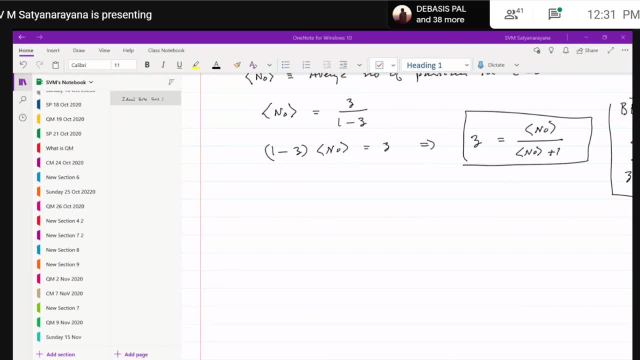 Can you close? Yes, Hello sir. Yeah, Sir, in the previous class, while deriving this partition function, sir, at first you wrote something called occupation number: representation right: N0: number of particles: Yes, sir. so like that, sir, this: the energy state e0 is degenerate right. there can be two states. 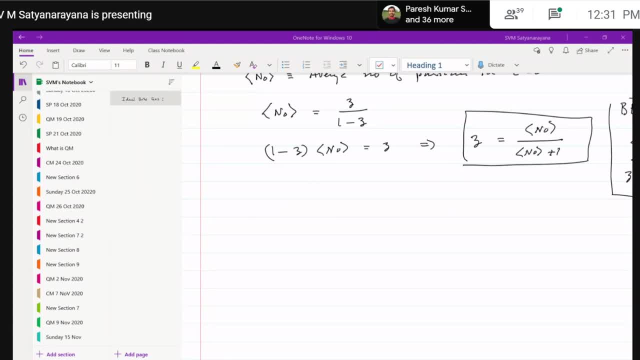 corresponds to that state: e0, yes, sir, e0, e1, e2. so these, these energy states, i mean they are degenerate. there can be two independent energy eigen states, corresponds to that. so when i am listing them, i am just listing the listing, the kind of individual states. 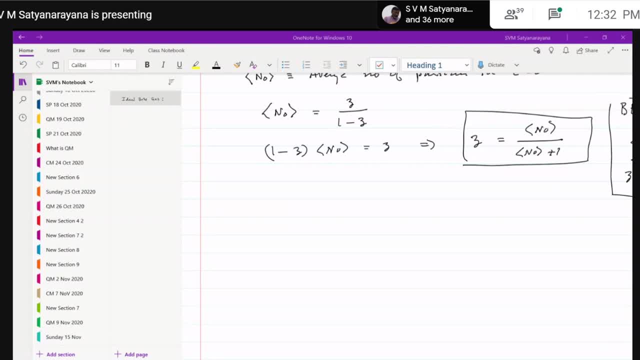 okay, i am not considering that degeneracy into into into account. for example, let's say i have e1 and e2, okay, but it is possible that e1 and e2 are same. but i am listing all of them. that's in this picture. i am listing all of them. 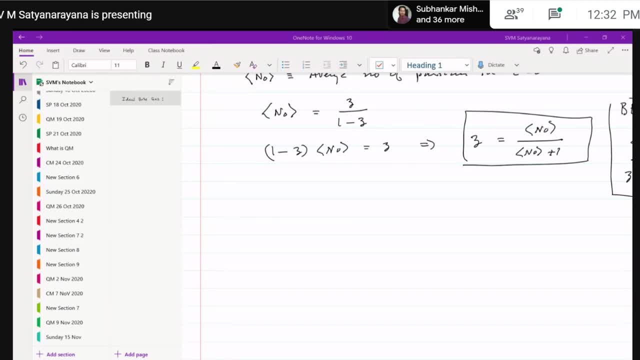 uh, yeah, yeah. so so e0, e1, they are equal, like this you are saying in some cases they may be equal if they are degenerate, but i am listing every one of these energy levels, whether they are degenerate or non-degenerate. but there is also another scheme in which you can keep track. 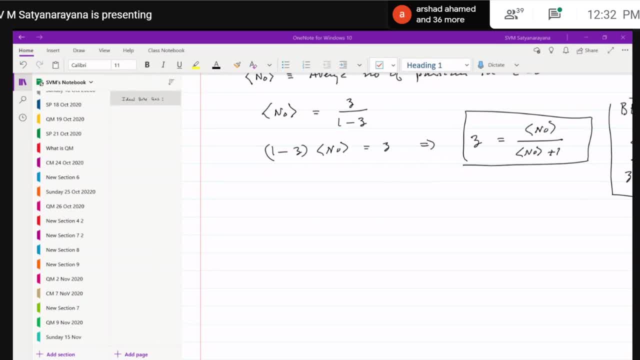 of those degeneracies. oh, so that's not, that's not this representation. maybe, maybe next time i can show that you how to do that one. but that is, you have take the degeneracy of each of these energy levels into account and then do something similar to what we do in microcanonic. 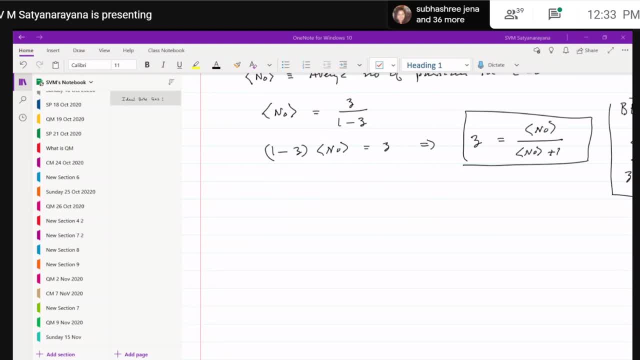 so because, sir, in formidirac, i mean in formidirac, statistics, statistics, if we take our particles as electrons, then since it has been up, we can have to each energy states can be twofold degenerate, right? so therefore i asked: yeah, yeah, but